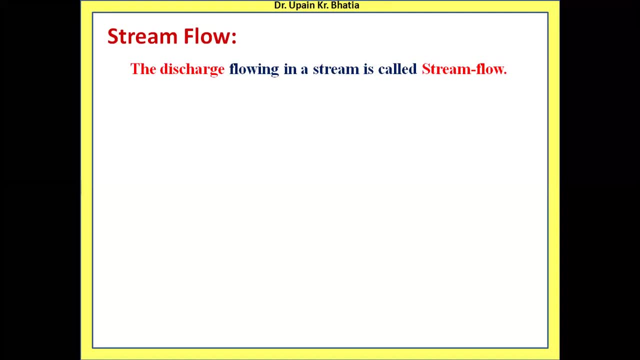 to deal with the stream flow of a stream. Here we have methods of measuring the discharge in a river of the stream, So we have two methods. The first method is the kind of ής, a full amount EBC. therefore the method is called a telefonics stream flow. So this: 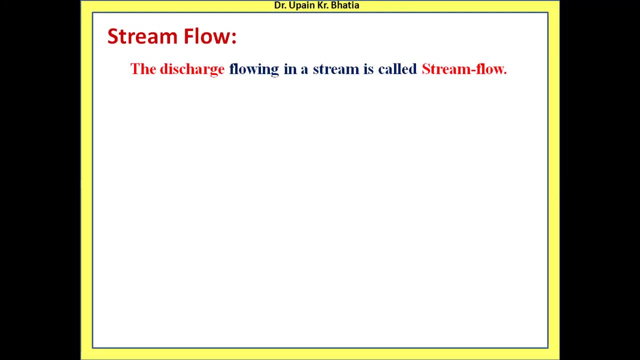 means that the stream flow without even **** flow of water. These are three indicators Now. the most common Retro73 are transformation. The first one is river flow. This is the river flow without any certain activebone. Another one is inflammation. So in that environment, 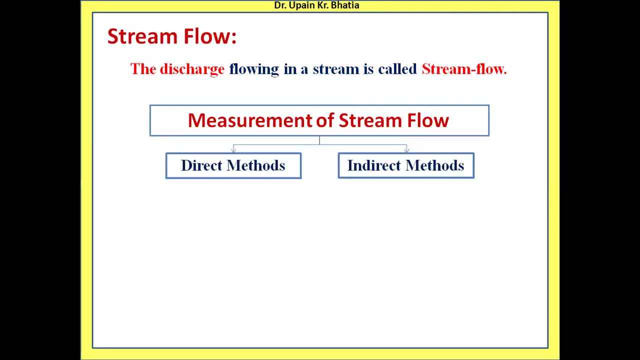 it is very common in that context. So just like a river. So remember, if you see the stream here you can have a video. You can refer to that video and this one Remember to return. divided into two categories, So the methods are included under direct methods or indirect. 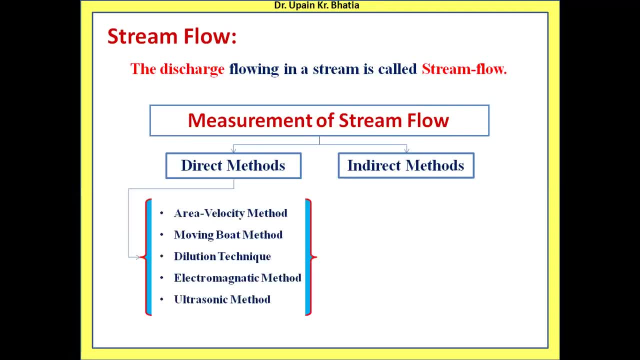 methods. So under the direct methods we have a number of techniques or methods like area velocity method, moving boat method, dilution technique, electromagnetic method and ultrasonic method. So there are many other methods also, but these are the main methods which are there. 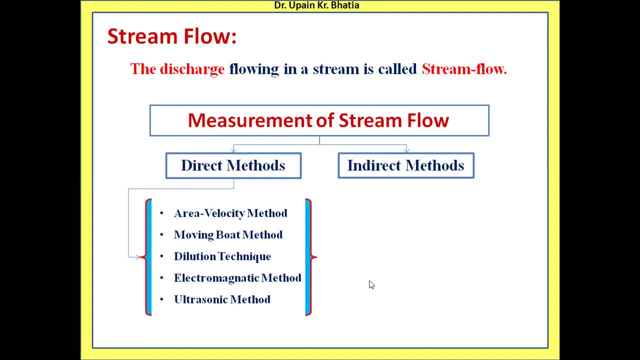 in the curriculum and we'll be discussing about these methods. Under the indirect methods we have a slope area method and by use of the flow measuring structures. So we construct some structures like weirs or notches or some flumed sections so that we can measure, make 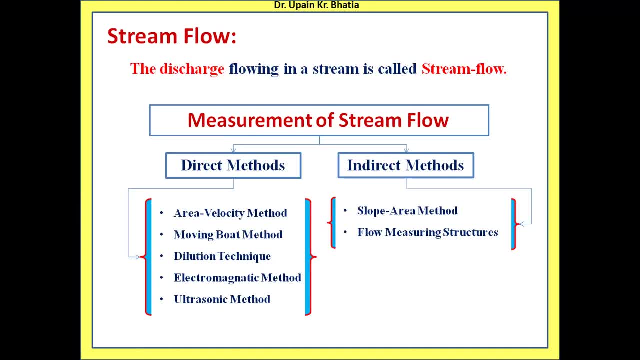 some measurements over there, Some observations, and on the basis of those observations we try to estimate the discharge flowing in the stream. So these flow measuring structures are beyond the curriculum so we will not be discussing about them. So all these methods under direct methods and the 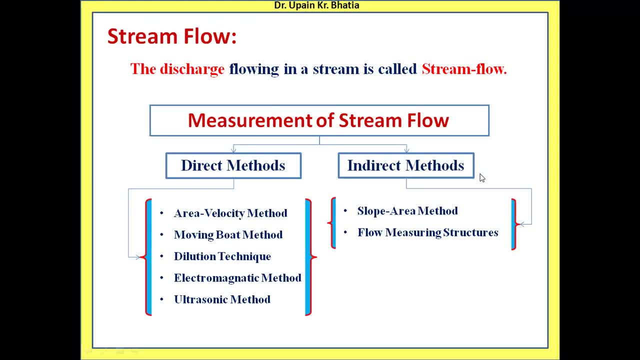 slope area method under these the heading of indirect methods. that will be discussed. So before we start with the first one, I just want to convey you that the flow measuring structures are beyond the curriculum So we will not be discussing about them. So before we start with the first one, I just want to convey you that. 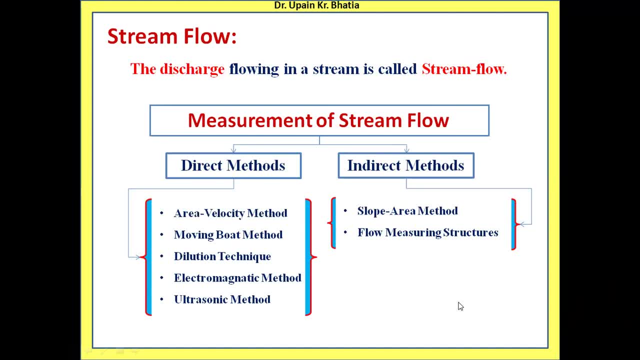 the flow measuring structures are beyond the curriculum so we will not be discussing them. So before we start with the first one, I just want to convey you that velocity method and the slope area method are important for the point of view of test and examination because they form basically the numerical portion. 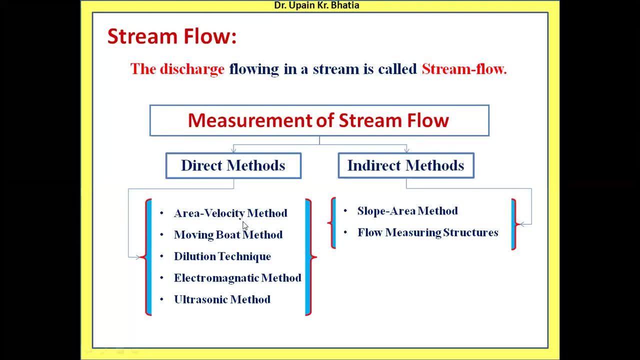 And you can find some question based on area velocity method or the slope area method, either in the test or in the final exams. These moving boat methods, dilution technique, electromagnetic method and the ultrasonic method are important for the point of view of test and examination. 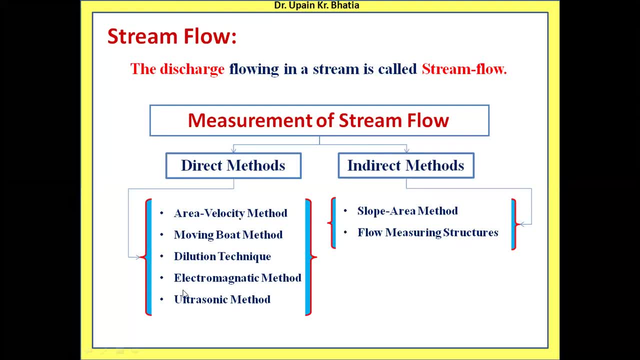 So these four methods. of course they involve some calculations, but in this particular context, in this particular chapter, we will be discussing about their theoretical part only. So first of all we will consider these four methods, that is, moving, boat method, dilution. 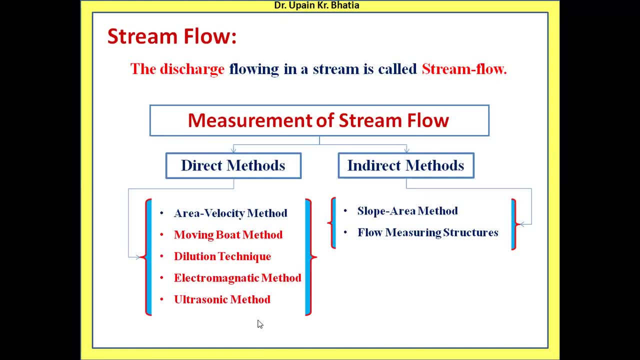 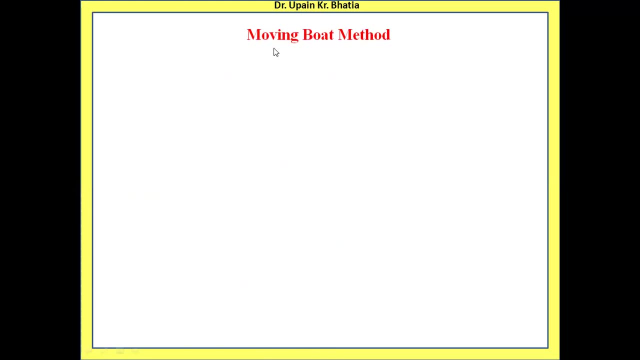 technique, electromagnetic method and the ultrasonic method. Then we will go to area velocity method and then to the slope area method. So today we will be discussing all these six methods. So the very first one is moving boat method. So, as the name suggests, 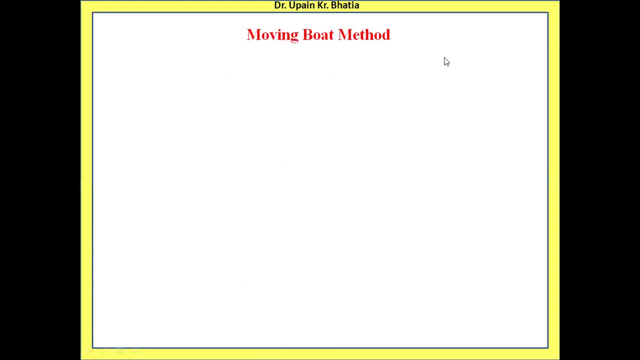 we have to take a moving boat. In the last lecture we discussed about measurement of velocities, So there was a topic of current meters, that we have to insert some instrument called current meter at some depth below the water surface. And what was that depth? That was dependent on the size of the river or the stream. If 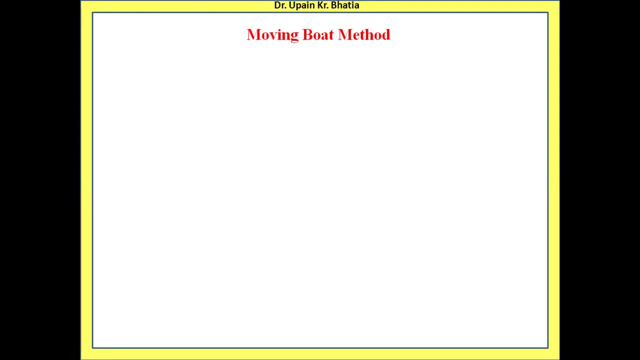 it is a shallow one. we use one point method. That means the current meter is to be lowered at a depth equal to 0.6 h, where h is the overall depth of the stream. So at 0.6 depth. 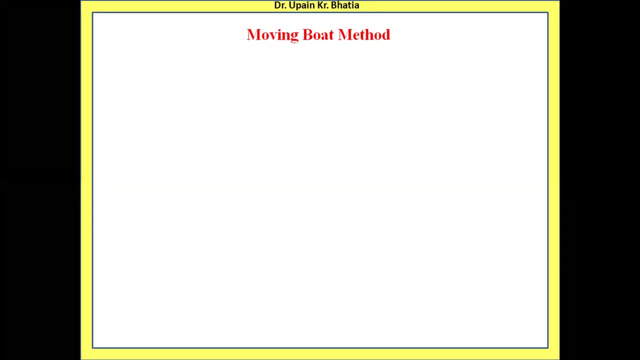 whatever velocity is measured by current meter, that is taken as the average velocity of the stream. So we need to insert the current meters at various sections in the river So these current meters are taken up to that point in the river through the boats, Of course, if the flow is. 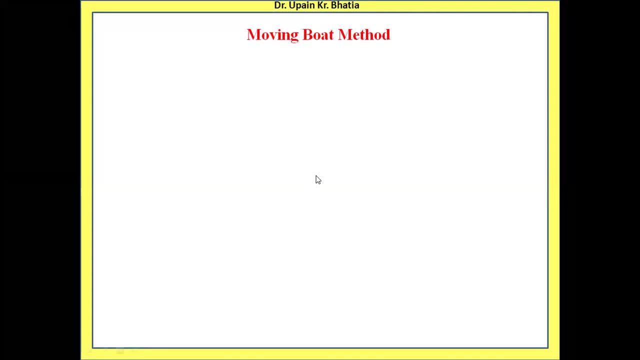 gentle in the river, then it is possible to maintain a still position of the boat so that at a particular point you are able to measure the stream velocity. So we need to insert the current meters velocity below the boat inside the water cross-section. But if the water is flowing at a very high 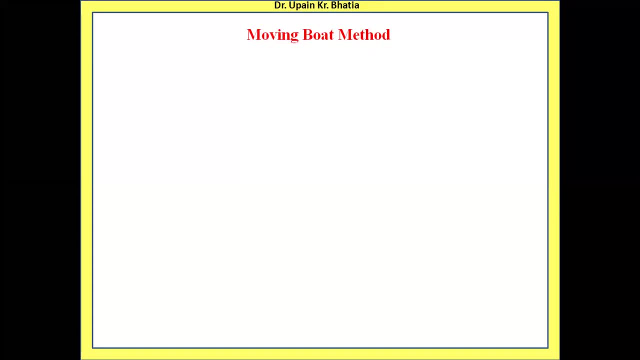 speed, or if the river is under flood, then it is not possible to maintain the boat still, so it will be moving. So under this moving boat condition, how we measure the discharge or how we measure the stream flow, so that method is basically the moving boat method. 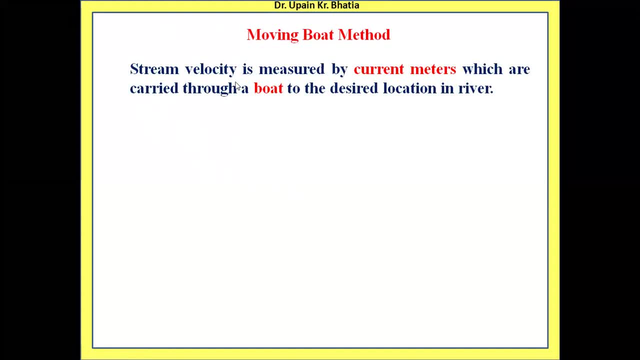 So let us consider these some points. Stream velocity is measured by the current meters, which are carried through a boat to the desired location in the river that we have just discussed. So stream velocity is to be measured by the current meter. So this is one of the important. 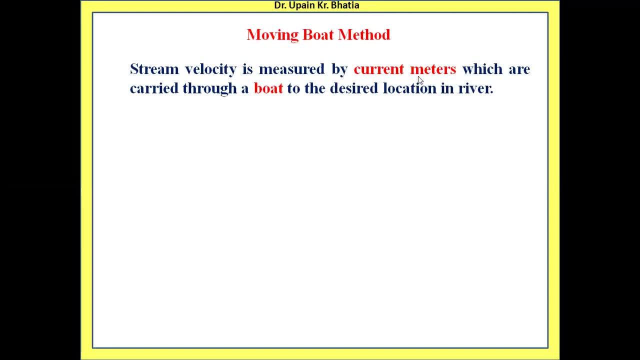 points And these current meters are carried through a boat and they are lowered below the water surface up to a desired depth, and then we can measure the velocity. So in order to measure the stream velocity accurately, the boat is to be kept stationary, So this: 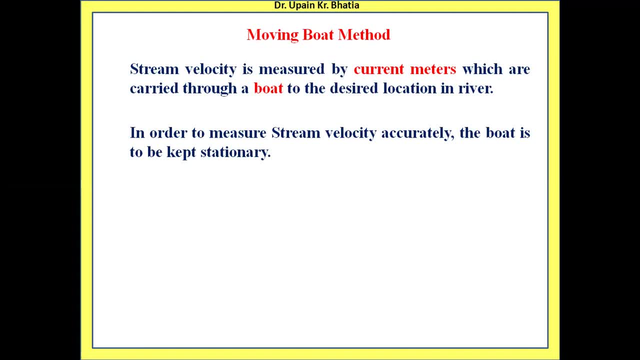 is very important because at a point, if you are going to measure the velocity, say at 0.6 depth, then the current meter will be lowered up to that point and the observation is to be made for a certain period of time. If you recall, the current meters had a certain 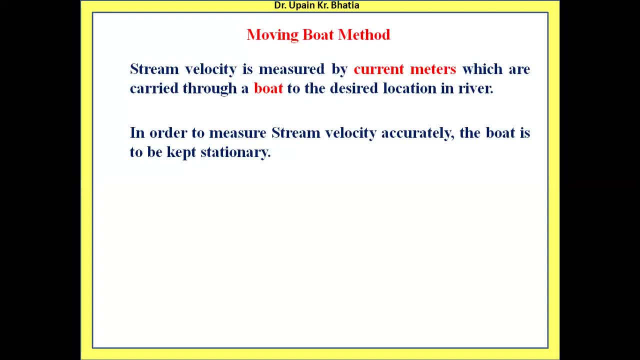 duration like 10-15 minutes, So I can change. I can say that for each of the everytime measured thing we can do, for example, a distance and then proceed with a corresponding Deriv image, and then we cannot measure a certain's depth right now. So each of the 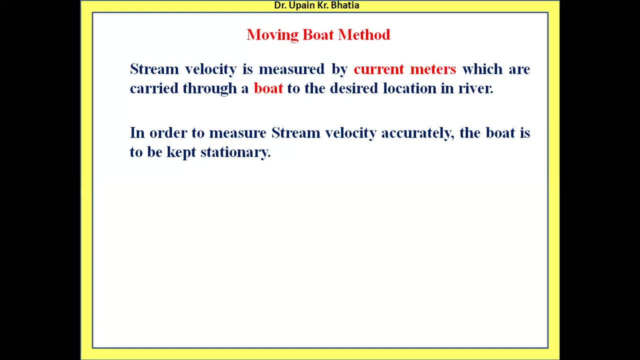 15 minutes, let us have the duration. So for each of the 15 minutes here we have minus one meter for each of the number of observed times. So it is the number of rotations on this ship and the speed of the currentвон or the velocity of the birth, both of these. 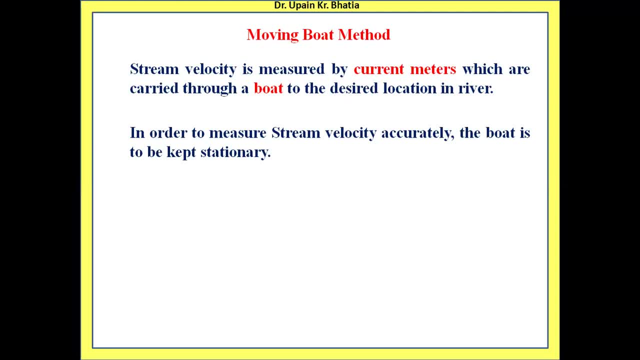 are pointed, And this is for the different transitions. these two, two types of transitions depends on the velocity. Then there is a number of rotations, depending upon the calibration equation, that are being measured. I have reduced, therefore the rotation speed is calculated. 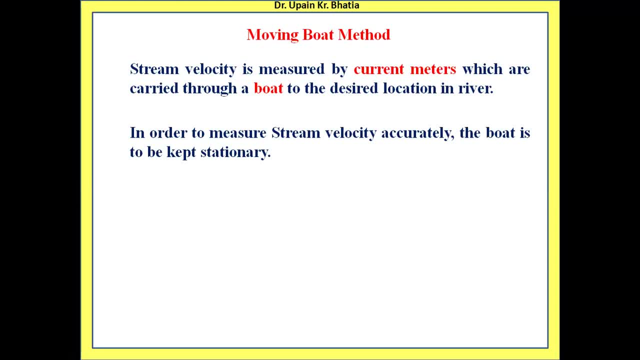 if there is, we can also give constant Curiosity in terms of the number of rotations, during which we will be counting the number of rotations. so that's why it is very important to keep the boat stationary in the stream. so that's why it is the sentence says: in order to measure. 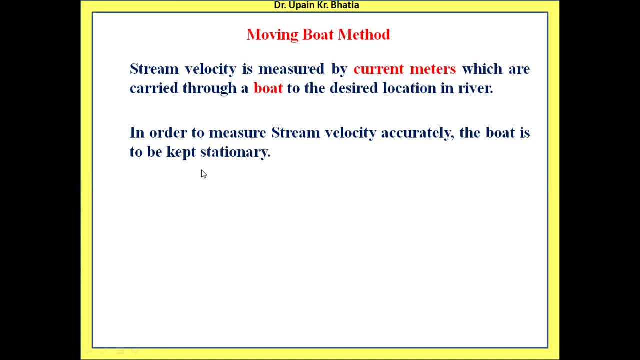 the stream velocity accurately, the boat is to be kept stationary. okay, now let us move on to the next point. so when the river is in spate or in flood, it is difficult to keep the boat stationary. that is also true because if the river is under flood, that means the flow velocity is. 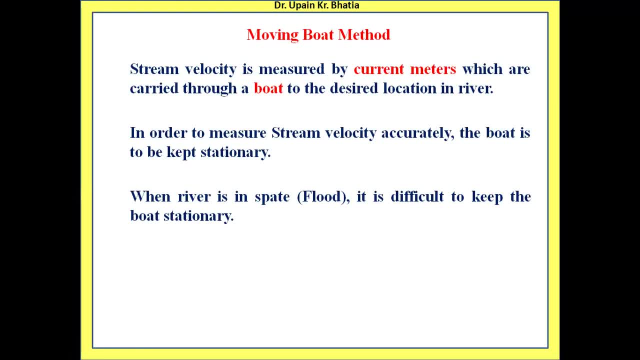 very high, then it is not possible to keep the boat stationary at a particular point, so moving boat technique is helpful in such situation and a special current meter is used which is free to rotate about a vertical axis. so you have studied two types of current meters: vertical axis current meters and horizontal axis current meters. so it is very 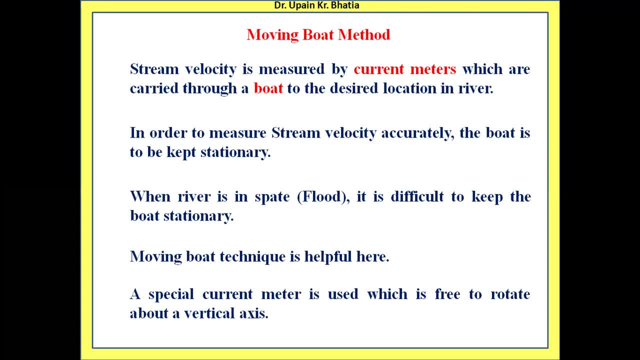 important to mention over here that we should not get confused with the name like vertical axis- current meter- and the horizontal axis- current meter, with this vertical axis. so this vertical axis is to orient the current meter itself, not the rotating element. so by default, whatever current meters we have, 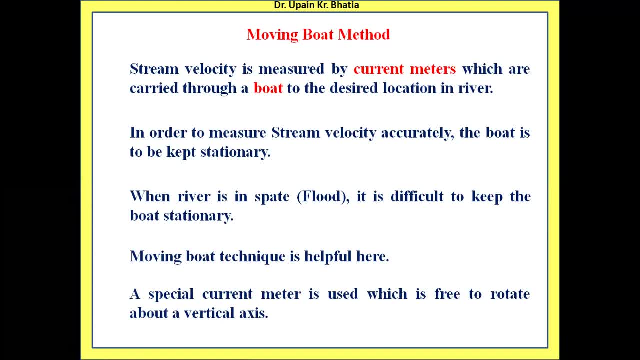 discussed in the previous lectures. they are of this type that they are free to rotate about the vertical axis, about, about the hoisting cable, just cable, say us current meter co suspend character panic and the leakage I data. I took current meter k back side page of stabilizing. 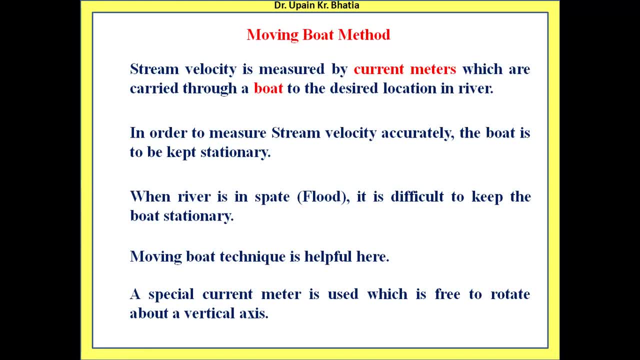 fins. hey, whoa, automatically align car. they have current meter k propeller co. you have to escape cup assembly co towards the upstream so that the water which is coming from the upstream side that is directly taken by the rotating element. okay, so when the boat is moving. so there are two components if you move a boat in. 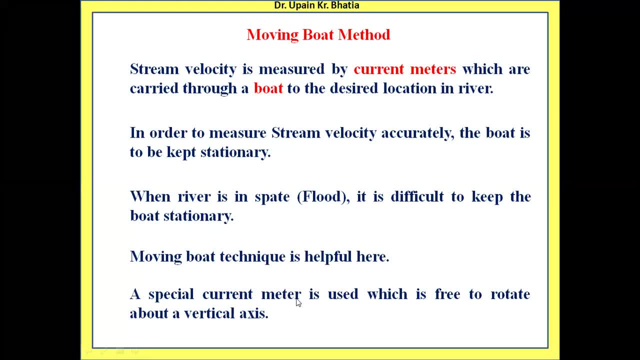 still water and tow a current meter along with it. I got up make boat may. I got up a current meter, Nietzsche's, and if the boat is still, then current meter will not be recording any rotation. but if you start moving the boat, if the boot boat is a say moved at a particular velocity, lake is still under that. 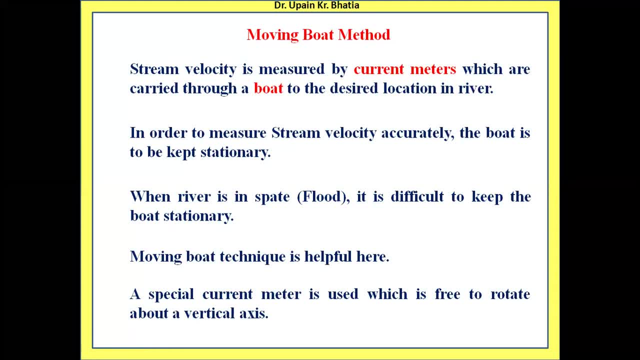 situation, the current meter will also be towed along with the boat and some rotation will be observed. so that will be relative velocity of the lake water with respect to the current meter. so we have to take into account that also. because in moving boat, in when the boat is moving, one velocity will be observed by the current meter on account of the velocity of the boat itself and another component of the velocity will be due to the flow velocity of water in the stream. so that's how a special current meter that is to be used with respect to the current meter. so we have to take into account that also. because in moving boat in when the boat is moving, one velocity will be observed by the current meter on account of the velocity of the boat itself and another component of the velocity will be due to the flow velocity of water in the stream. so that's how a special current meter that is to be used with respect to the current meter. so we have to take into account that also. because in moving boat, when the boat is moving, one velocity will be observed by the current meter on account of the velocity of the boat itself and another component of the velocity will be due to the flow velocity of water in the stream. so that's how a special current meter that 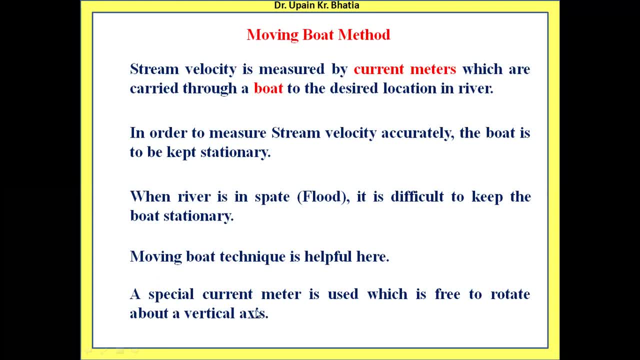 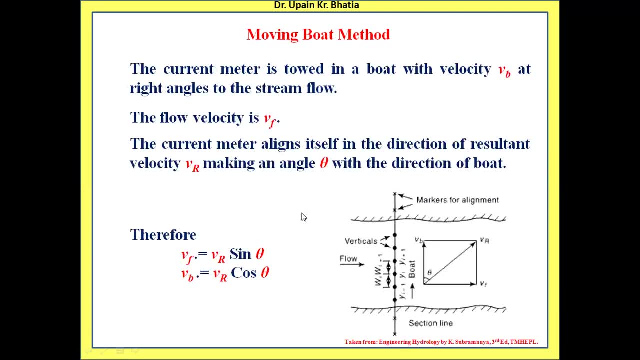 also because in moving boat, when the boat is moving, one velocity will be observed by the current meter on account of the velocity of the boat itself and another component of the velocity of the water in the stream. so that's how, a special current meter that down on the banks, so that we can align this cross section, So at this cross section, so 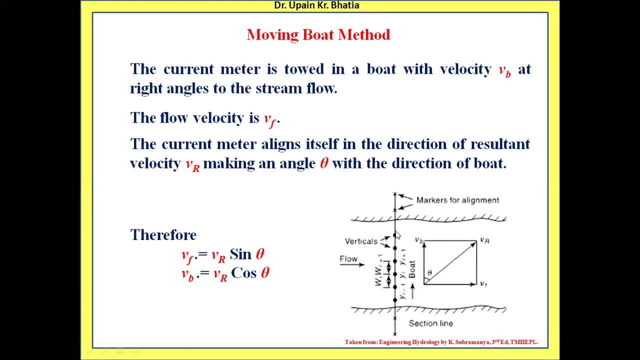 let us divide this section by some points further. These are known as verticals. So here, because you are looking at this river from top, so these verticals are viewed as a point. Okay, so this is not actually a point. it is a vertical line which is extending from 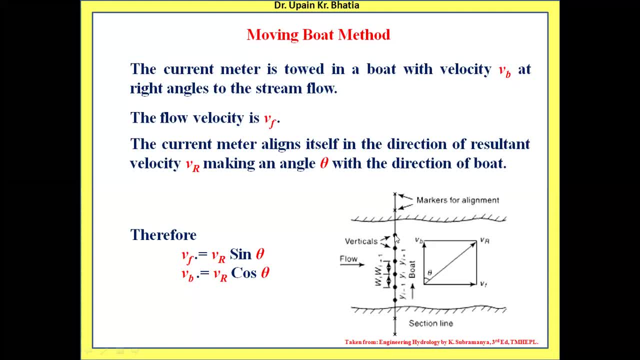 the water surface up to down, up to the bottom of the stream. So all these verticals, this vertical, this, this, they will be having different vertical heights because from water surface, the bottom of the river or the stream at this location will be at different depths. 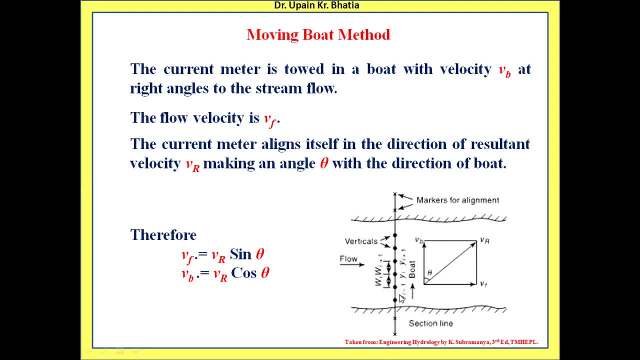 So all these components will be, all these verticals will be noted down for their various depths. So for that we can make use of some acoustic. you can say the depth meters. Now, further, if you see, the current meter is stored in a boat with velocity Vb. So Vb is basically. 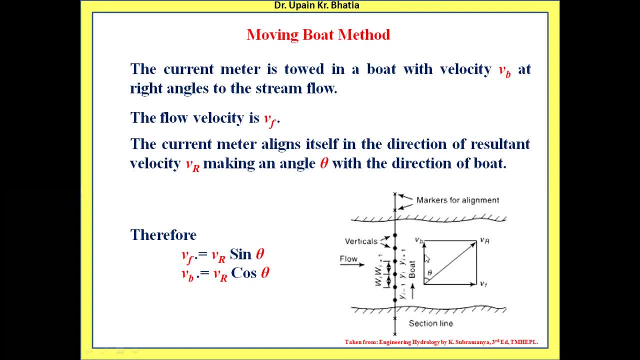 the velocity of boat. So velocity of boat is in this direction. So we try to carry the boat along this cross section with the velocity Vb, So which is at right angles to the stream flow. So stream flow is in this direction. that means velocity of flow Vf, The flow velocity. 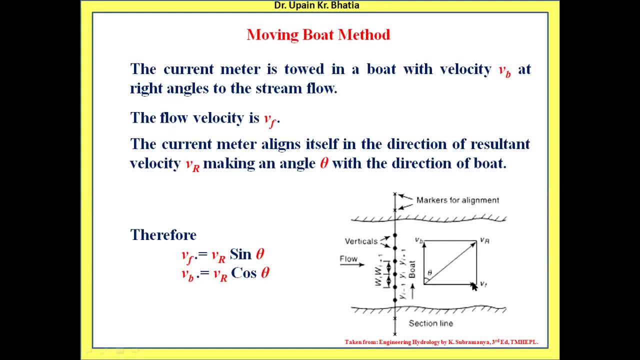 is Vf, which is in this direction, in the horizontal direction of your screen, And the Vb is in vertical direction of your screen, So both are at right angles. So this Vb is at right angles with this stream flow and the flow velocity is Vf, so Vb and Vf are perpendicular. 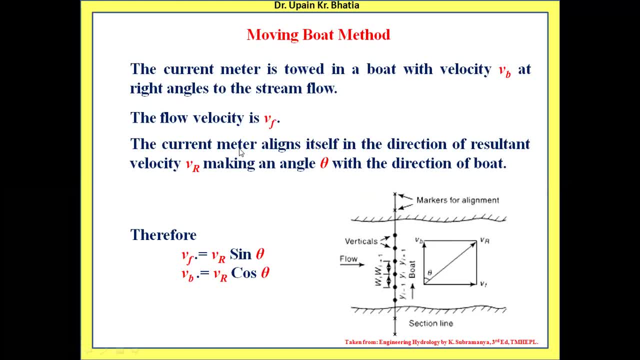 to each other. Now, next is the current meter aligns itself in the direction of resultant velocity, vr, making an angle theta with the direction of boat. So we have measured this angle theta with the direction, of course. So this is also important: If you measure this direction, this theta with the direction of boat, then these components, 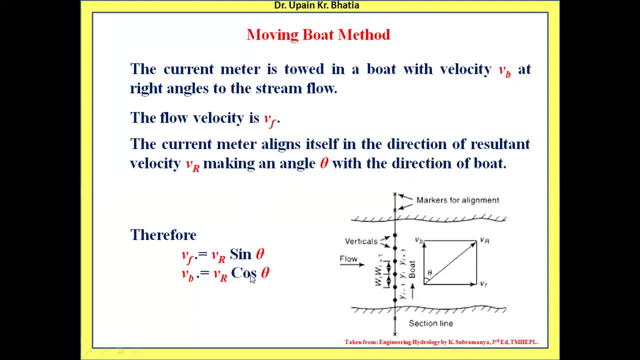 will be sign and cost theta will be put in some order. But if you measure this theta instead of measuring it with the direction of boat, if you measure it with the direction of flow of water, then obviously the sign and cost will be reverted. 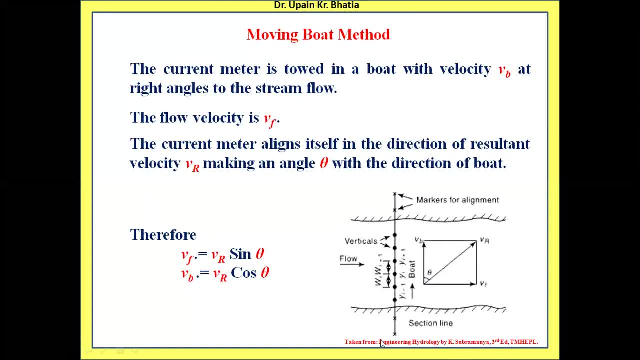 So if you see this diagram, which is taken from engineering hydrology book by K Subramanian Tata, McGraw-Hills education private limited. So it is taken from the third edition that is available with me. This is the diagram which is given in that book, but actually this diagram is not perfectly. 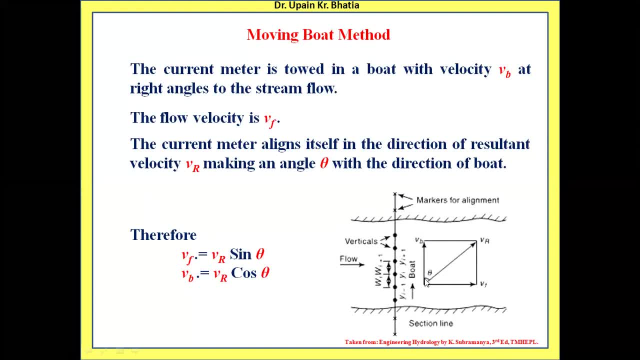 okay, because when the velocity of flow is in this sorry- velocity of boat is in this direction and velocity of flow is in this direction, then resultant is not in this direction, because this is the flow velocity. Okay, That is the velocity of water which is observed by the current meter. 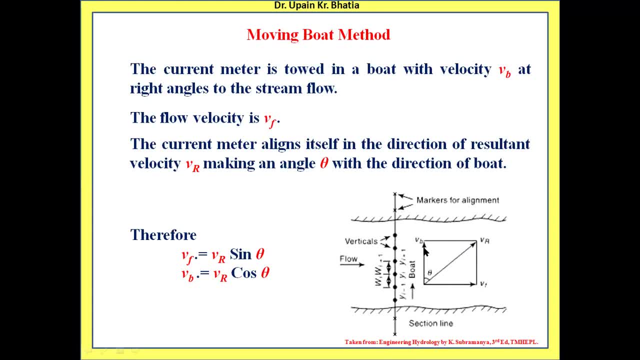 And if the boat is moving in this direction, the apparent velocity will be opposite to that. So velocity of the water. suppose if this river is still, if the water is still and you move the boat from this point to this point, So this is the direction along the arrow, then the current meter will feel that this. 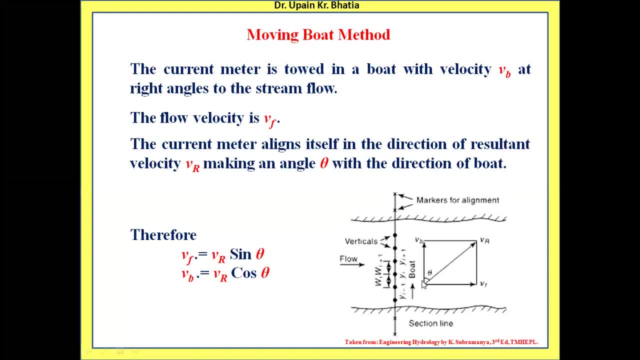 water is flowing from this point to this point. that is opposite direction. So, if you see the apparent directions of the flow due to movement of what, it will be in the downward direction over here, as of this screen is concerned, and the flow velocity is in right direction. 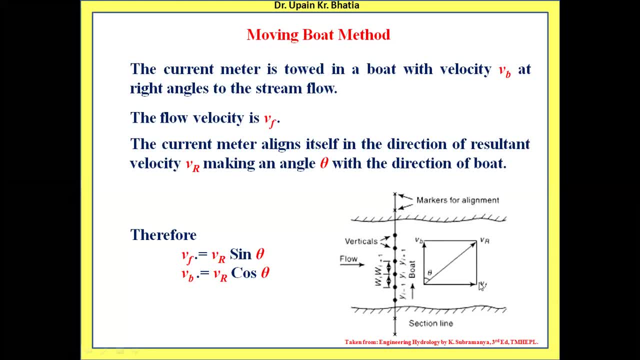 So resultant will not be along this line, rather, it will be along this line. Okay, So this is one mistake in this particular diagram, which is taken from engineering hydrology by K Subramanian. It is a very, you can say, well-established book. 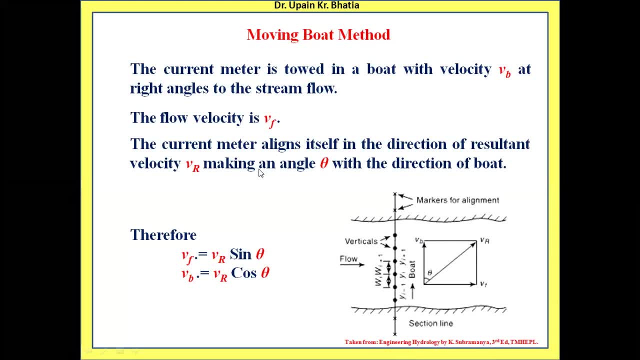 Okay, But somehow some mistake is there. So, anyways, it doesn't make any difference If you just calculate these values, the components, if this is the VR, that is, the velocity in resultant, or the resultant velocity, because these two components are perpendicular to. 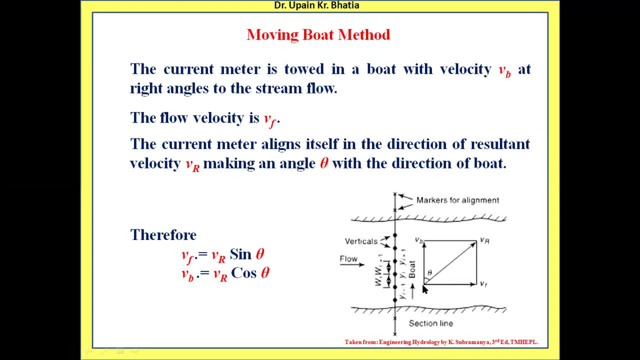 each other. the length of this diagonal or this diagonal, that is the same, but so magnitude of the resultant It is the same, but the direction is this much, from this VB point to this VF point. So this will be the apparent direction. 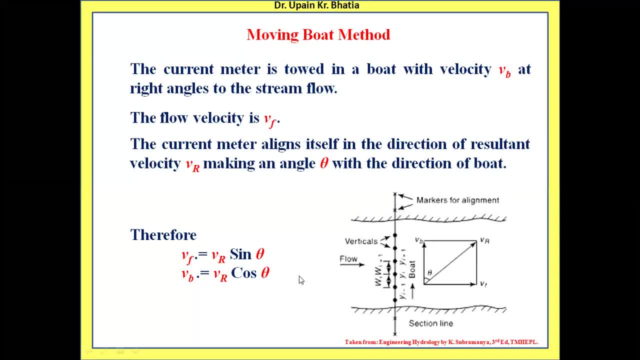 So as of uh, you see the values of these components. So that will not be uh, that will not make any difference. So velocity of flow that is equal to resultant velocity multiplied by sign of theta, and velocity of boat is resultant velocity multiplied by cost of data. 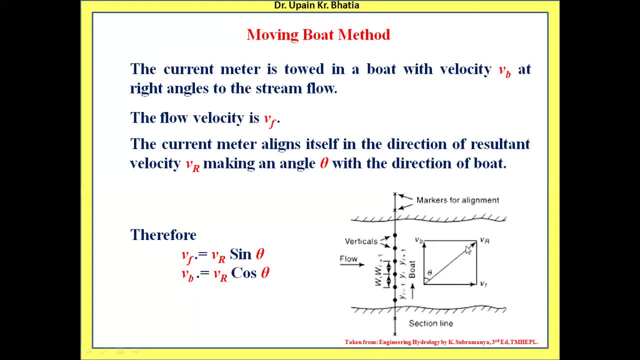 You know that if this is VR, Okay, Then the component of this V are in the direction where theta is aligned. So, along with theta, this component is of cost value and the opposite component is of sign value. So if this is VR, then this component is VR cost data and this component is VR sign theta. 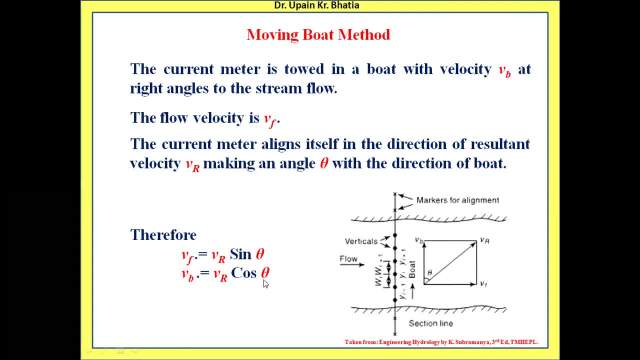 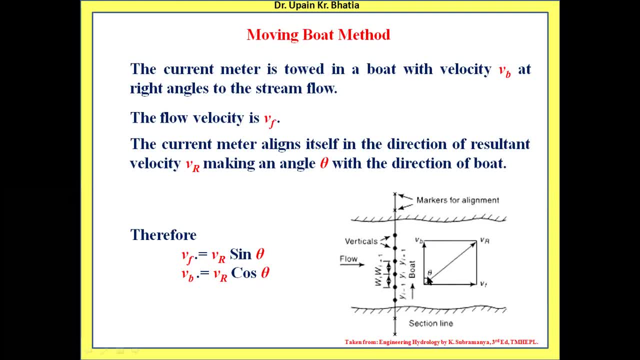 Okay, Okay, Okay, Okay, Okay, Okay. Now, this theta is also measurable because we had us. we had this special current meter, So it is free to align itself along any direction, and the direction of its alignment is observable from the boat itself. 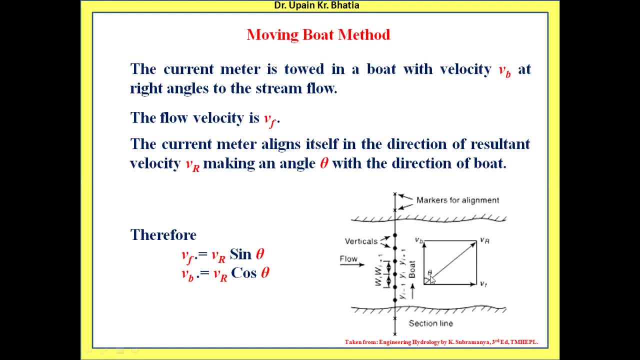 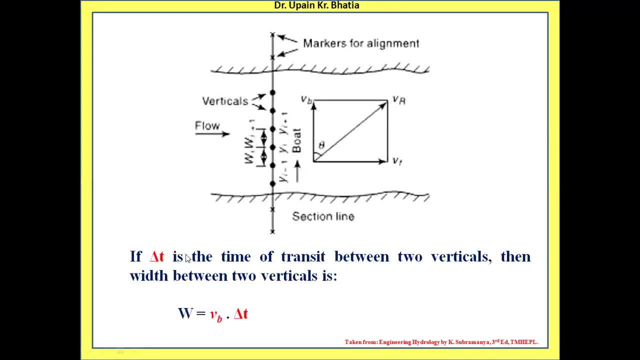 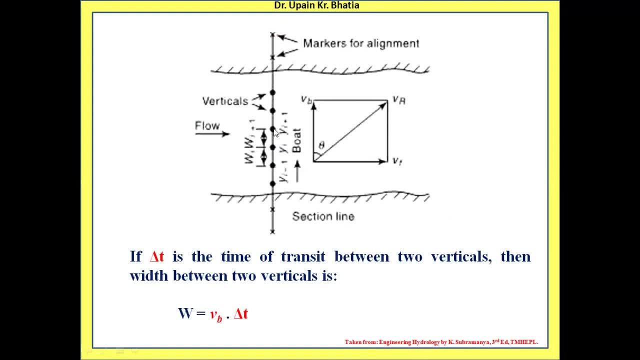 to this point, or from this point to this point, so between any two verticals, if the boat is moving from this point to this point, if the boat takes time, delta t. so if delta t is the time of transit between two verticals, then the width between two verticals is: if delta t is the time, and along with 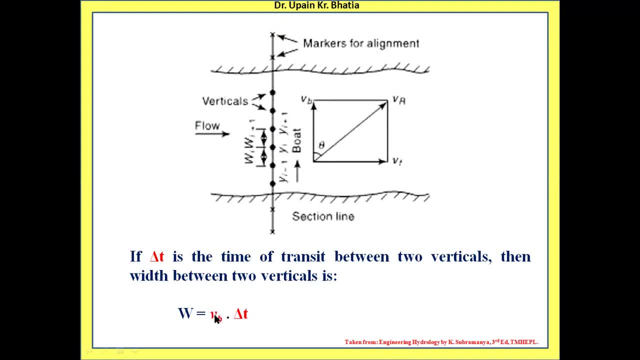 this direction. the velocity is VB, then velocity multiplied by time is the distance covered. so distance covered will be equal to W, so the width of this river between two verticals. so you will be dividing it into various segments: first, second, third segment, fourth, fifth, like one. so between any 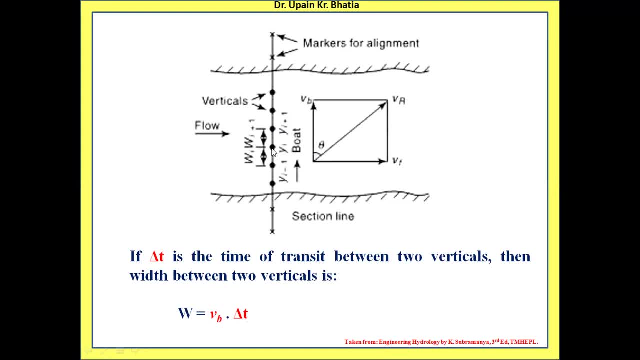 two verticals we had. we have a segment whose width, W, can be calculated in this fashion. so W is equal to VB multiplied by delta t. so likewise all the W values can be calculated. and for convenience we generally keep these verticals equidistant, and so that big time which is taken because VB is constant, so every time same. 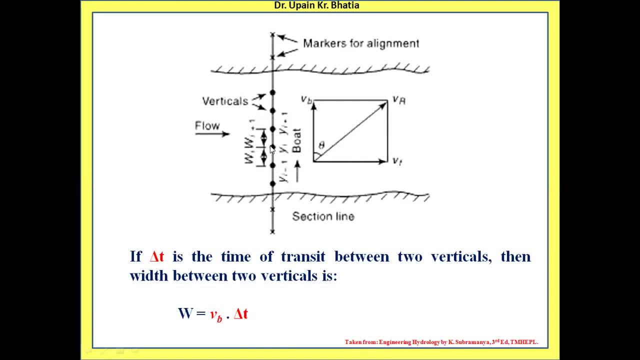 time, delta t will be taken from one one vertical to the next and from next vertical to the next further. okay, so all these W values will be equal. otherwise, if you have different verticals at different spacing, so you can calculate the distance between the verticals in this fashion. 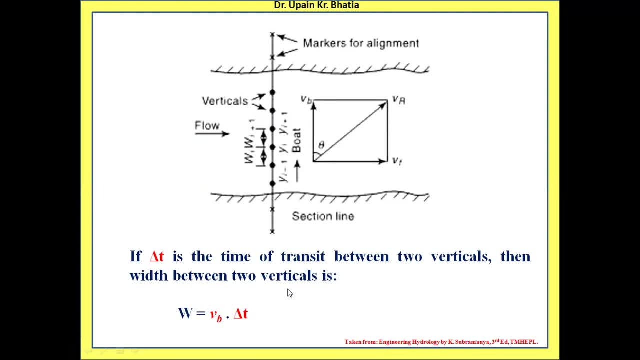 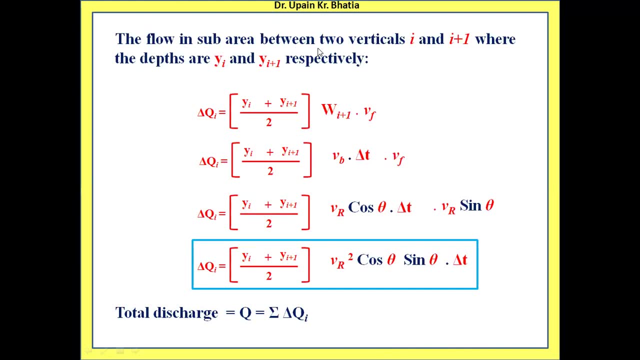 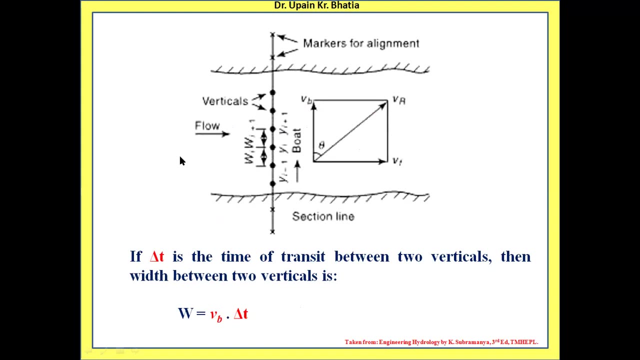 by noting down the time interval. now, if you look at this procedure, the flow in the sub area between two verticals in the previous diagram. if we have selected any two verticals, let me mark over here, let us say this vertical and this vertical, if you say so, between 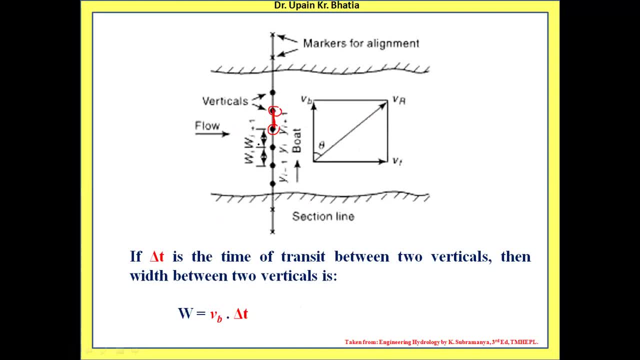 this: this is the width of the vertical And if you see the cross section, this is deep enough up to the bottom of the stream. So if you see from this side, if you see from the side, you will see a cross section area between these two verticals. Okay, So that's. 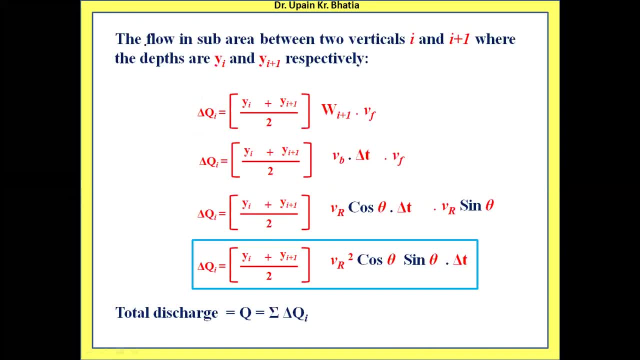 why? here the thing is the flow between a flow in the sub area, between two verticals. Let us say I have vertical and the next I plus one vertical, where the depths are why I and why I plus one? because at every vertical depth is different, So the at I, vertical. 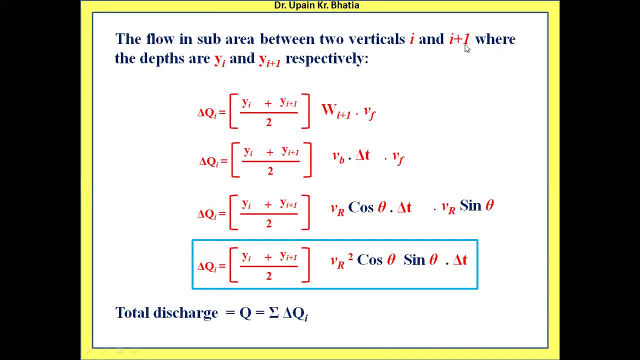 let us say the depth is by I and the next vertical I plus one. the depth is why I plus one. So if you work out the discharge, so discharge is equal to area multiplied by velocity, So area is the average depth that is adding the two. 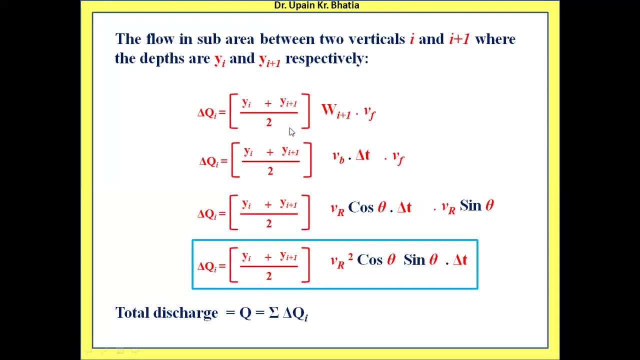 Depth at two verticals divided by two. So this is the average depth of flow. This is the width of the strip or that sub area. So this depth multiplied by this width, this portion gives you the area. And if this area is multiplied by the flow velocity, V F, then 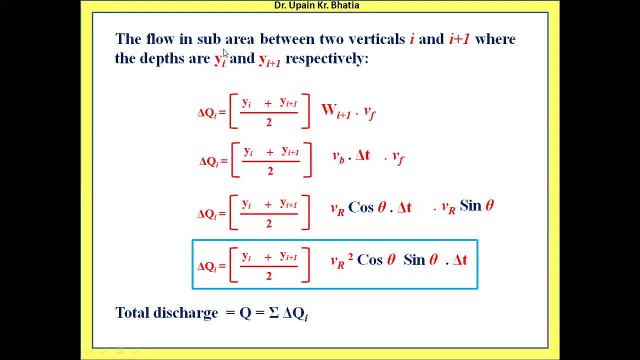 you get the discharge which is passing through this sub area. Okay, So all these discharges are added to it Together. So if you uh see it further, this W I plus one or this width can be written as VB into Delta T, as we have discussed in the previous slide. So this velocity of boat. 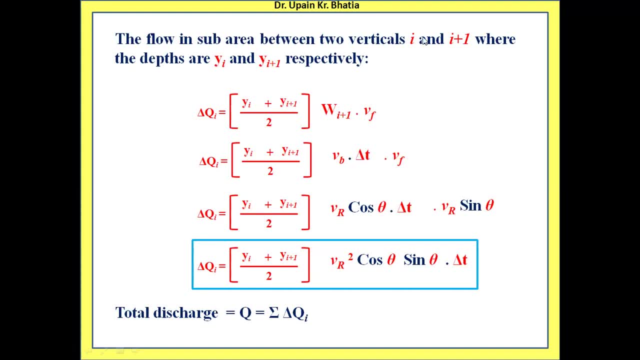 multiplied by the Delta T, that is the time taken to travel from I vertical to I plus one vertical. So that is this W, I plus one is treated as it is replaced by velocity of boat multiplied by Delta T. Now, In this particular expression now put the values of VB and VF. So VB is VR, cost theta. 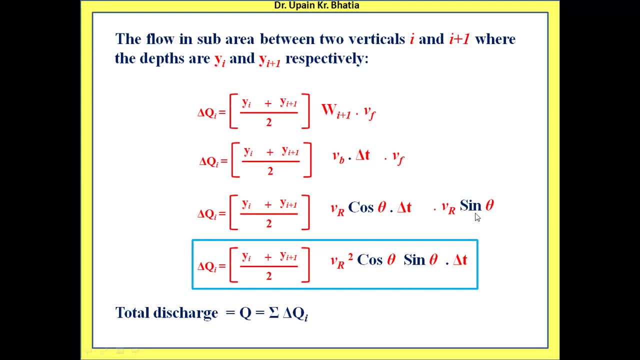 and VF is VR sine theta. So if you have put it this way, so we are, is appearing twice. So you can rewrite it as VR square cost theta multiplied by sine theta multiplied by Delta T. So this gives you Delta Q. I value in a particular sub area or the particular segment. 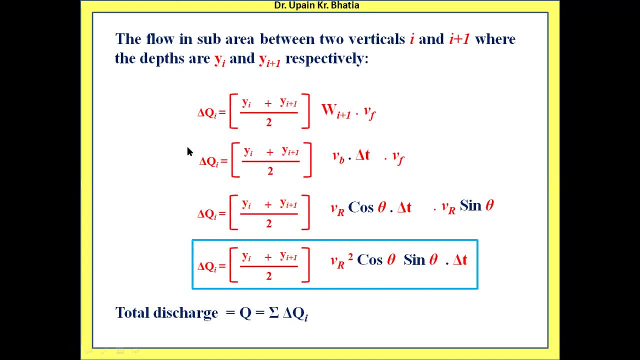 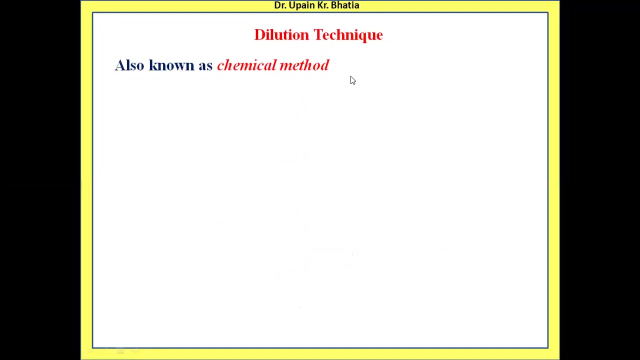 And then finally, for every sub area, if you calculate these Delta Q I values, you can add them together, summation of Delta QI values, to get the total discharge. So this is the basic concept of using the moving boat method. And if we move further, the next method is a dilution technique, which is a chemical. 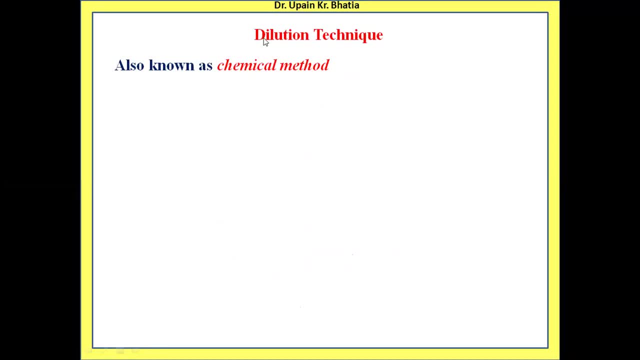 method. Okay, It is also known as chemical methods. So dilution technique is basically in the previous video. You have to use the method of dilution And, by the way, I made method. So dilution technique, as the word says, dilution, that means you have to put something. 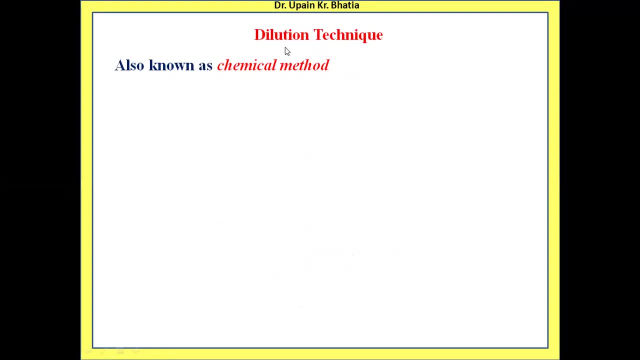 which is concentrated and later on it will get diluted. So that dilution, measurement of this, that concentration, or the dilution that will be used for measuring the discharge. So let us consider these points one by one. So let a non-reactive tracer has the initial. 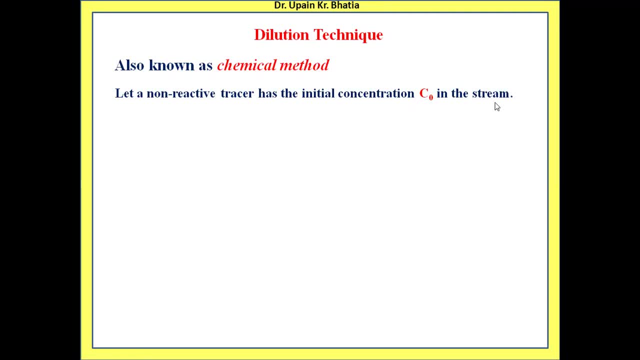 concentration C0 in the stream. So let us understand this: We are talking of a tracer. We are talking of a tracer, a material which is non-reactive. It is not reacting with anything in the water or any other equipment that we are inserting it into it. So it is a normal. 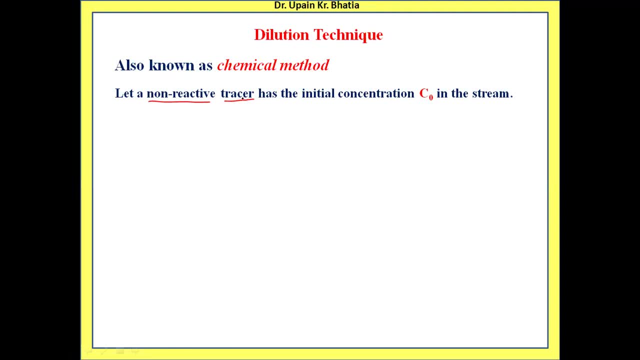 tracer. So tracer is any material which we can observe, which we can measure, whose quantity we can measure. So that is the tracer, And its characteristic is that it should be non-reactive, So that whatever tracer we put in the river, it should be observed in a non-reactive way If it reacts. 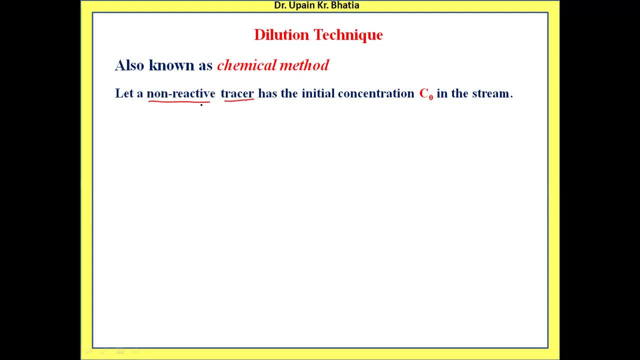 with something else, then it will be consumed. Then obviously we will not be able to measure the exact concentration of this tracer. So let us consider this. So this tracer should be non-reactive. So this tracer should be non-reactive. Now, next is: has the initial concentration, initial concentration C0 in the stream. 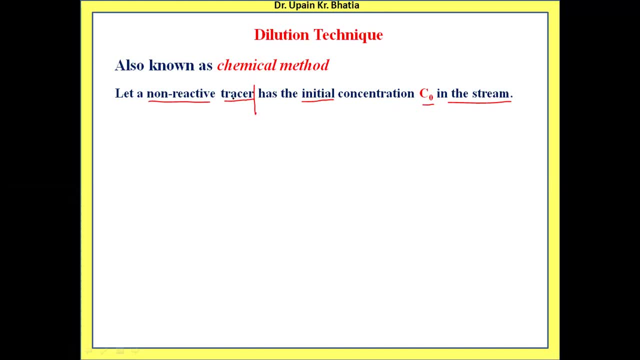 Now in the stream, initial concentration of this tracer is C0 in the water. That means before we add this tracer into the stream, some part of it is already present in the stream, the stream. so this makes an important observation or important point that 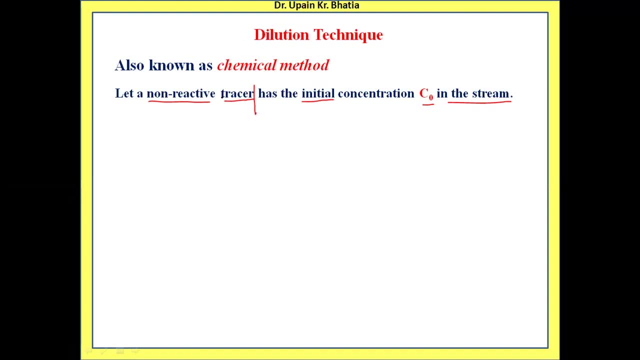 generally the tracer is adopted as a material which is already present in the stream water to do naturally stream water can the case are a minerals, who think is our contents? who they have? only may say we as I, a component, less again, just key concentration. I'm easily measure cursory, or before we add that 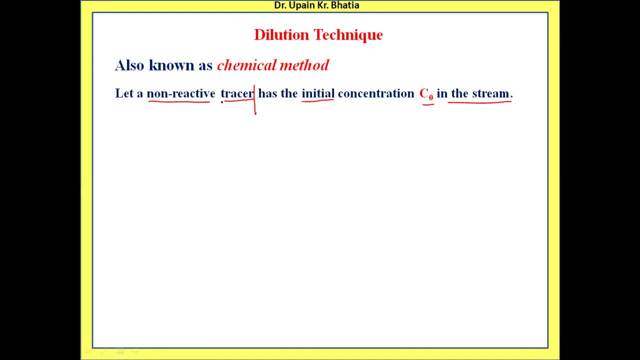 tracer into the water. how many booze keep hello? initial concentration check key: that value is C 0, so C shouldおき concentration already. ooh, stream water may present head. so let us move further. inject the tracer, the concentration C 1, in the stream at section 1. 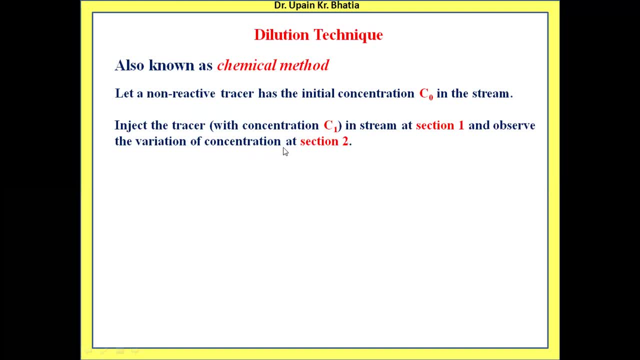 Tdoggle 244, 3, 0 and observe the variation of concentration at section 2.. Now let us understand about this. We are talking of section 1 and section 2.. This means we have to take two sections. So what are we doing at section 1?? 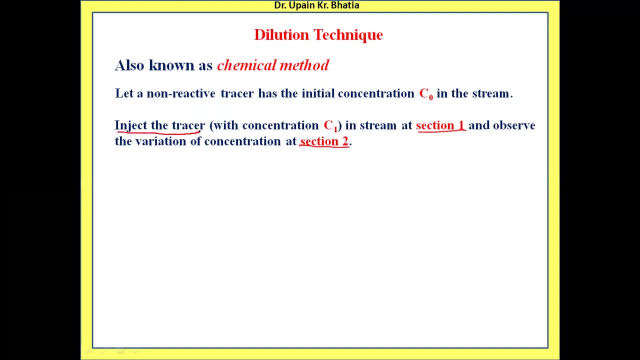 We are injecting the tracer. Inject the tracer whose concentration is C1. So it is not C0.. C0 is the concentration which is already in that stream. Now we have made another concentration, C1, of that tracer and injected it in that stream water. 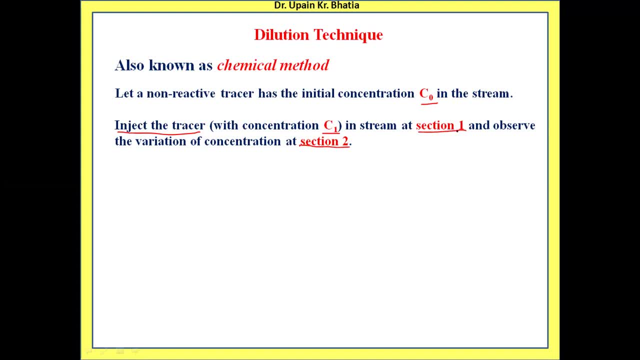 And where did we do it? At section 1.. And what did we do after that? Observe the variation of concentration at section 2.. At section 1, it has been injected. Its concentration is C0. And when it reached section 2, it was diluted. 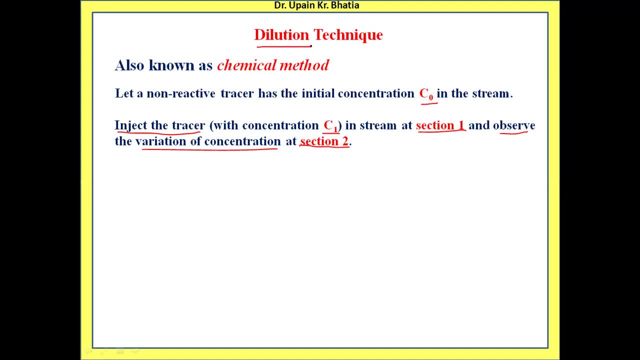 This is why it is called dilution technique. When it is diluted, we are checking the variation of its concentration at section 2.. So this is important to note. Okay, Next point is the tracer will be diluted during its journey from section 2.. 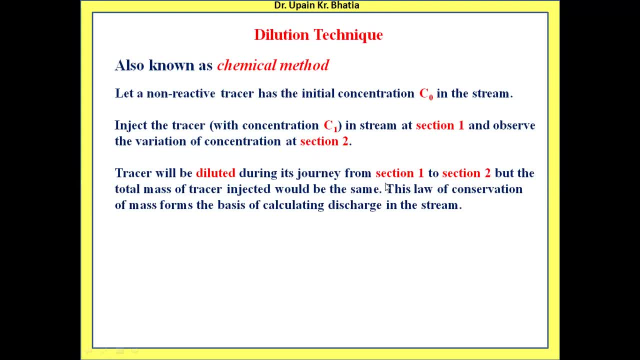 Section 2.. Then section 1.. Section 2.. Now let's do this. We have Take sections into river. mass of the tracer is same. It was in a small volume of water earlier whose concentration was C1. After. 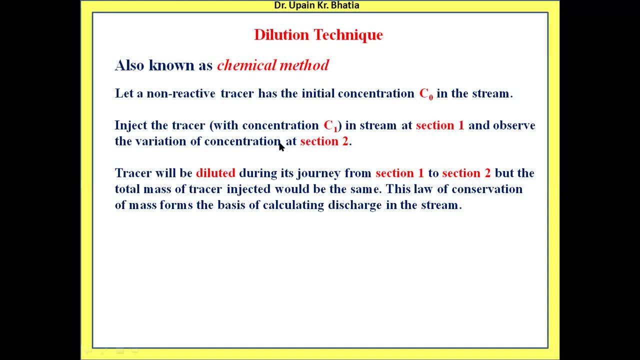 injecting that tracer mixed with the river water reaching section 2, it diluted. Now the same mass of that tracer is mixed with the larger quantity of river water. That's why it is diluted, But the total mass of the tracer injected would be the same. 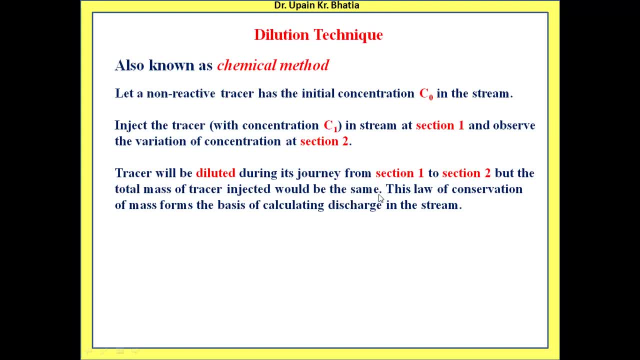 The total mass of the tracer will not change. It will not change. It is the same. It was in a small volume earlier. Now reaching section 2, it has mixed with the larger volume of water of the river. This is the only difference. 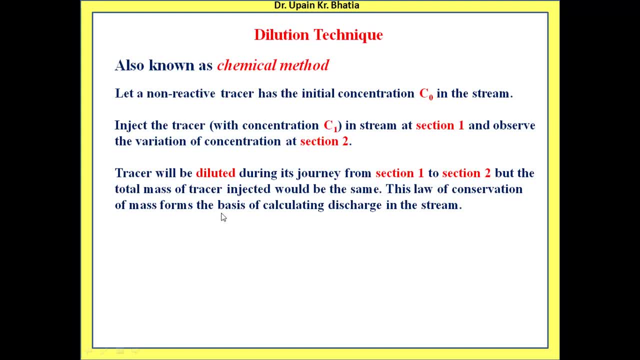 So this law of conservation of mass forms the basis of calculating discharge in the stream. Now, this is the law of conservation of mass. The amount of mass we have injected into the tracer, it will remain in it. So its variation, the concentration that we check. 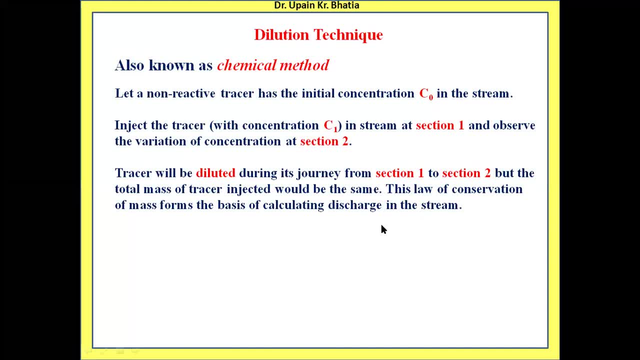 that will be the basis to calculate the discharge in the stream, And for that we will use two types of approaches. So two approaches of this technique are adopted. One is the sudden injection and the other one is constant rate of injection. Now what is the difference? 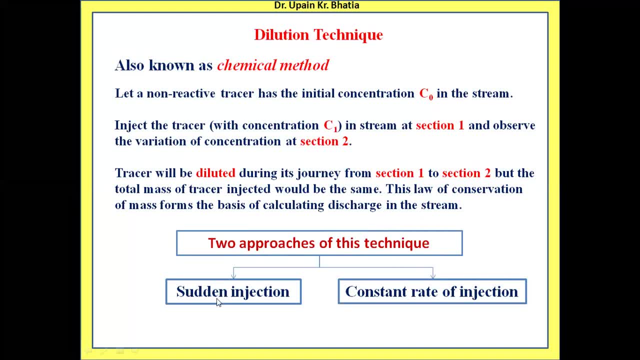 between these two techniques. We will discuss that in the next slides. But as the name suggests, the sudden injection means this tracer which is injected at section 1 is injected all of a sudden. That means the complete quantity of tracer is all of a. 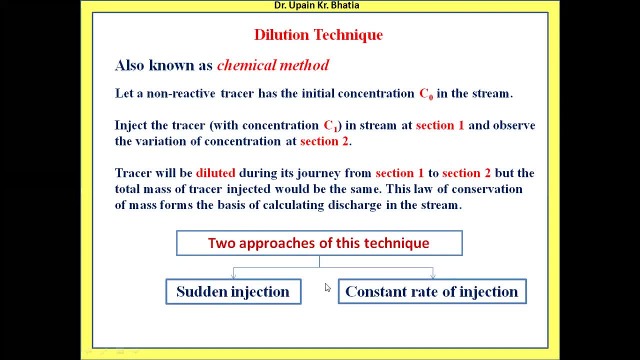 sudden it is put into the water at section 1.. But in this particular approach, the constant rate of injection. that means we have a liquid tracer of the concentration C1 and that tracer is injected continuously at some constant rate, So at a fixed rate. we 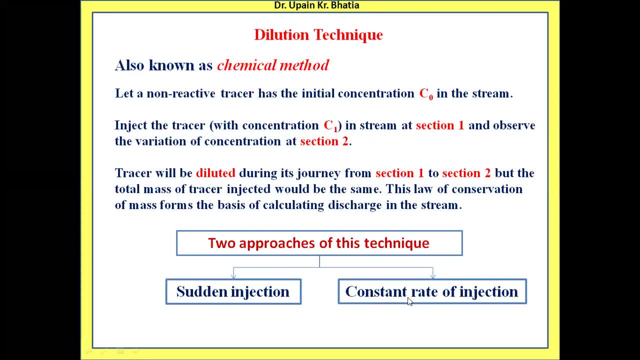 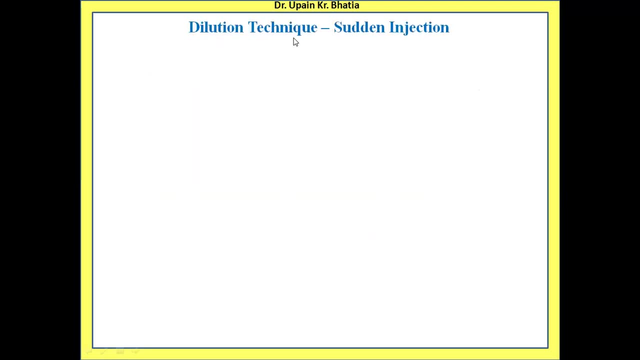 have started injecting, So we are releasing it through some pipe, So constantly we are not stopping it, So constantly we are releasing it into the stream. So how these two approaches function, So let us discuss them one by one. So, dilution technique: 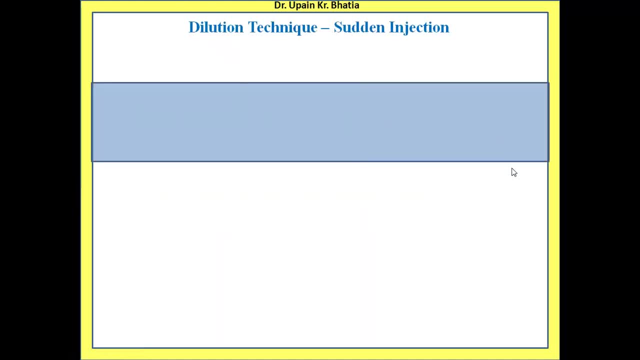 in sudden injection mode. So let us say: this is the river and this is section 1 and this is section 2.. Of course, this section 1 and section 2 should be at some appropriate distance So that we can allow the tracer. 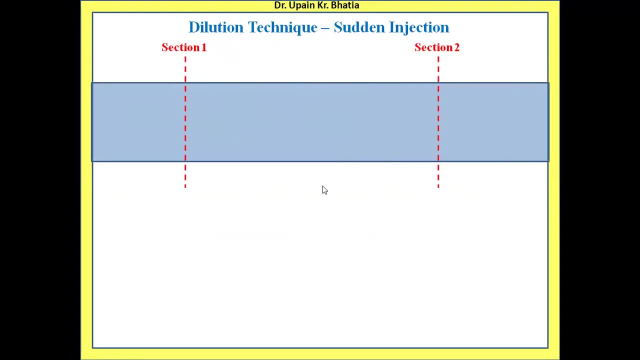 to get diluted from section 1 to section 2.. So at this section 1, the concentration C1 is injected. The total volume that is injected into it is, let us say it is, V1.. Now if you just release the tracer, all of a. 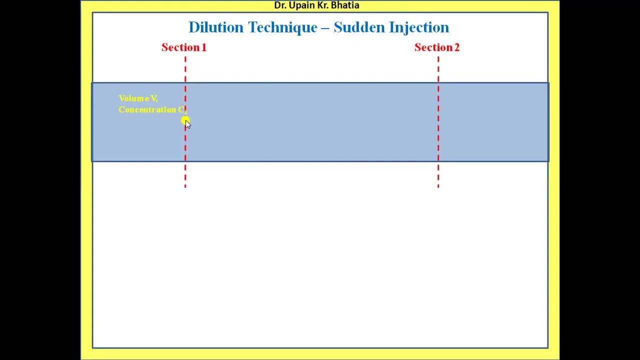 sudden. that is the sudden injection. we have put all the tracer at once. We have put all the tracer at once. Now, what will happen Here? that patch will be concentrated, But as it moves further it will increase in size, and I am lightening its color. 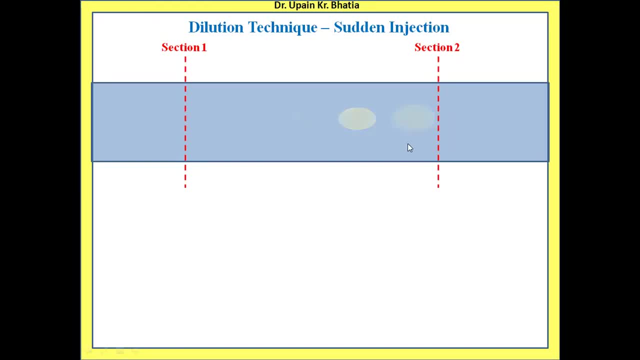 a little bit, Which is showing that it is getting diluted Now. so this tracer, which was put at section 1, it will flow around the section 1.. Now the size of this patch has increased, But what you see is the yellow color of its concentration. 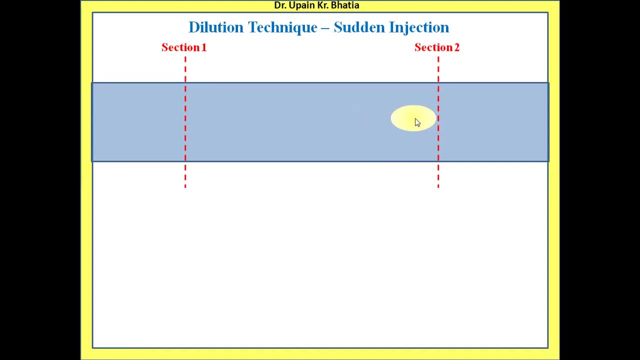 is means dark yellow color is there in the middle and light yellow color is there in the outer boundaries. That means the tracer that is there will start mixing with the river water from the outer boundaries only, So concentration at these boundaries will be lesser and the concentration will increase. 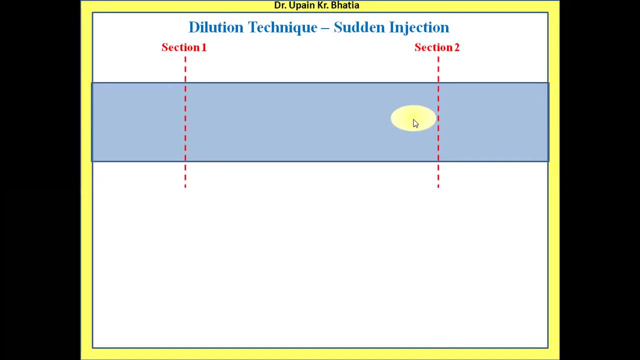 inward, So maximum concentration will be in the middle. So as this particular patch passes through this section 2, continuously, we have to measure the concentration. So the variation of this concentration is to be noted down. So when this patch touches it at this level, the 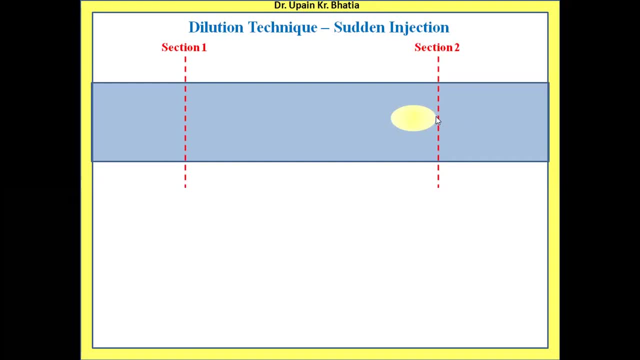 concentration of this tracer will be just equal to the concentration which is already there in the river, that is, the water. So as this patch crosses this section 1, so now this section 1 will be at here at this point. So concentration is increasing. 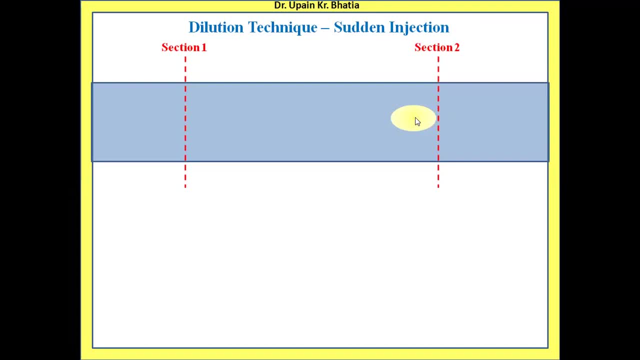 So, as this patch will go, it will pass this section 1, the concentration at section 2 will keep on increasing up to this. When the half of the patch has passed at that particular point, the concentration observed at section 2 will be maximum. 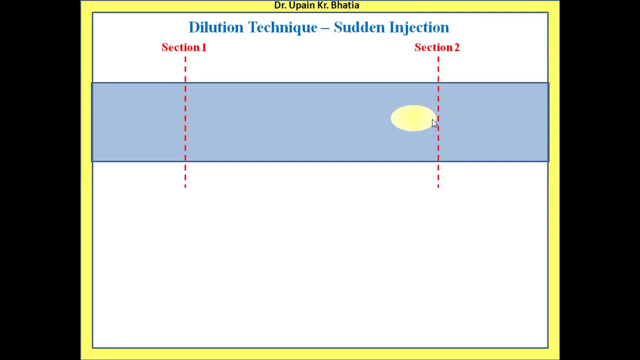 Thereafter, when the remaining half of this patch will be passing, that concentration will start decreasing down ultimately to the original value which is there in the stream. So this forms the basis. So it is written over here like: diluted and enlarged patch. Diluted- 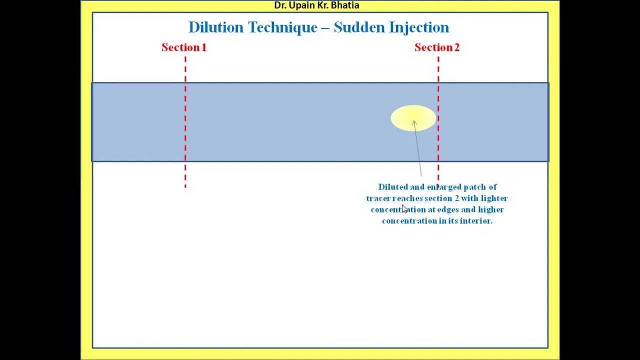 and enlarged patch of the tracer reaches section 2.. Dilute or enlarged patch has reached section 2. With lighter concentration at the edges, concentration at the edges is less and higher concentration in its interior. Its interior concentration is higher. Now what will we do? 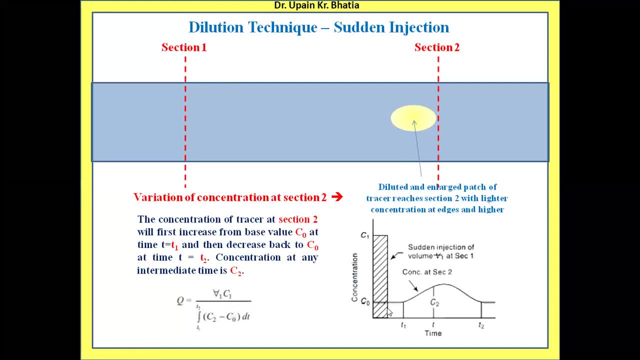 The variation of the concentration is observed. So this type of graph is observed. So this is the variation. the shaded one is the sudden injection volume V1 at section 1.. This is the high concentration. This tracer was injected at section 1.. 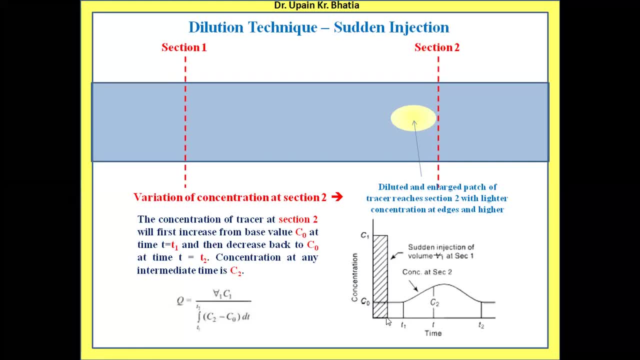 As soon as it was injected it finished. in a very short time It reached again, Because what we added, that is finished, That is not going to last longer. So this is the variation of section 1.. But at section 2, if you see, 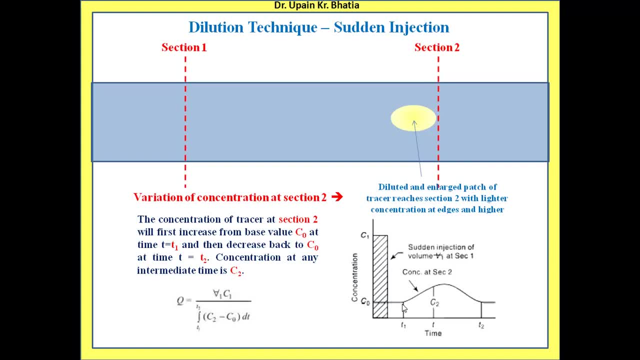 C0 is the concentration which is there After time T1,. this patch reached here As soon as we released it here. after time T1, this patch reached here And while reaching here, it was diluted and enlarged Now, as soon as it. 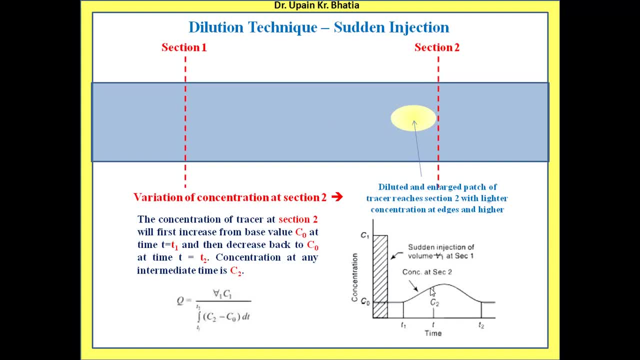 crosses from here, its concentration will start increasing up to a maximum value. Then it will start decreasing back to the same value, C0. Because C0 is the concentration of the tracer which is already present in the river water. So now this particular variation is because of: 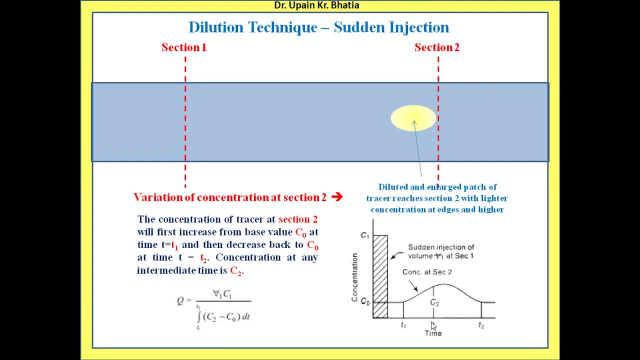 this injected tracer. So let us say at any time T, the concentration is C2. So the concentration of tracer at section 2 will first increase from the base value C0 at time T equal to T1. And then decrease back to C0 at time. 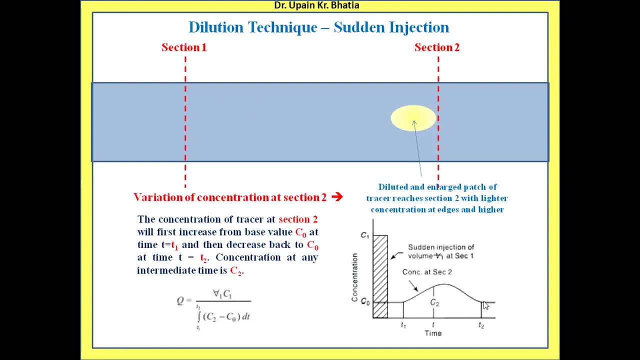 T2.. It will increase first, Then it will decrease back to C0 at time T2.. And the concentration at any time intermediate time between T1 and T2, that is C2.. Now, at any particular time of T1 and T2,. 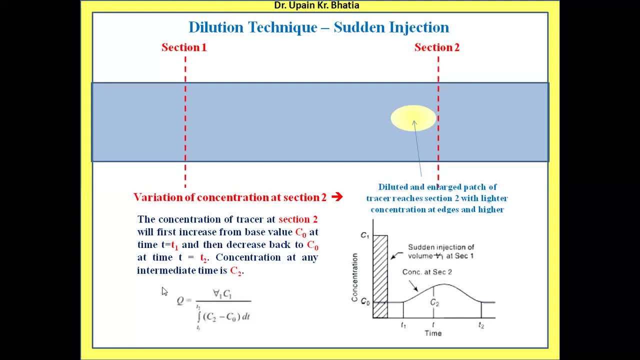 let us say, at T time its concentration is considered as C2.. Now this is the formula which is used, That is the volume multiplied by concentration C1. It is what is injected at section 1.. And this is the integration: See C0 minus. 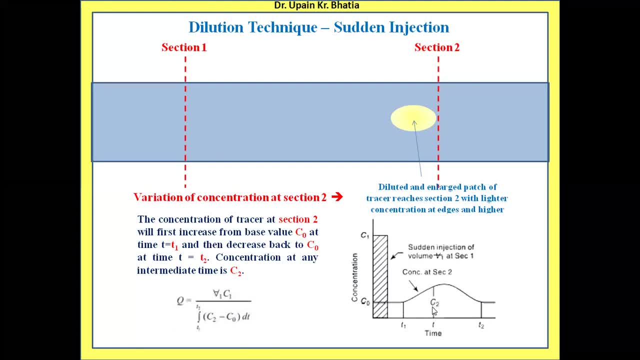 C2 is basically C2 minus C0. So because the total concentration, which is C2, is observed at any particular time, T this C2 is because of the tracer as well as what is already present in the river. So if you subtract C0 from, 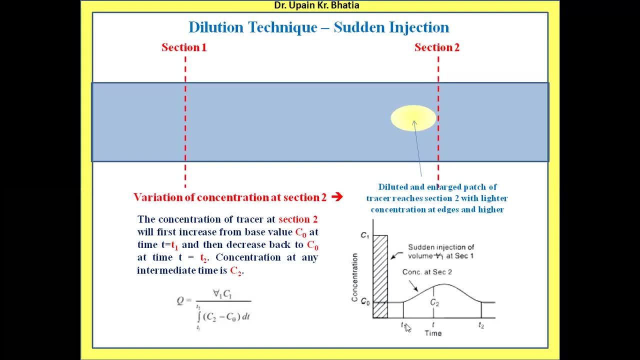 C2.. So C2 minus C0 is there And with respect to time, if you integrate, then if you draw a line over here, then this upper portion will be obtained. So this is the concentration and mass basically in the upper portion. 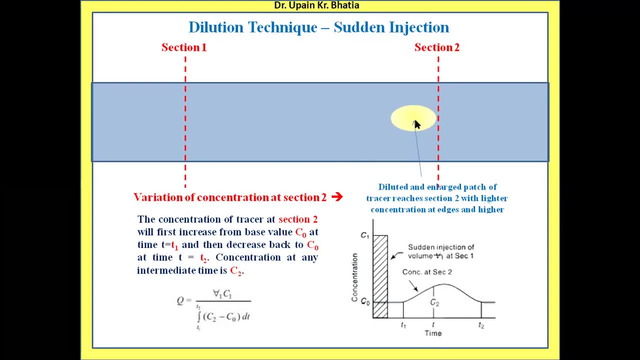 that is injected at section 1 and it has reached at section 2.. So integrating from time equal to T1 to T2 with respect to time Dt. So this is going to give you the discharge, because concentration over here and concentration over here, these units are. 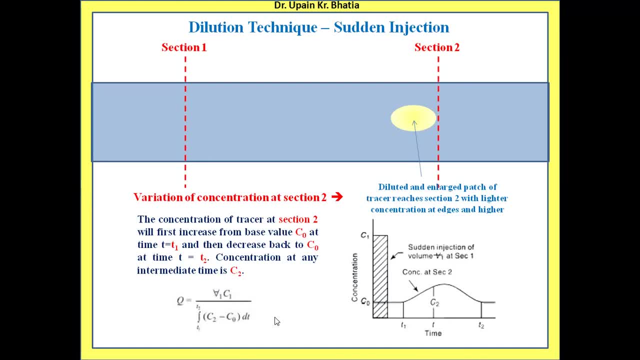 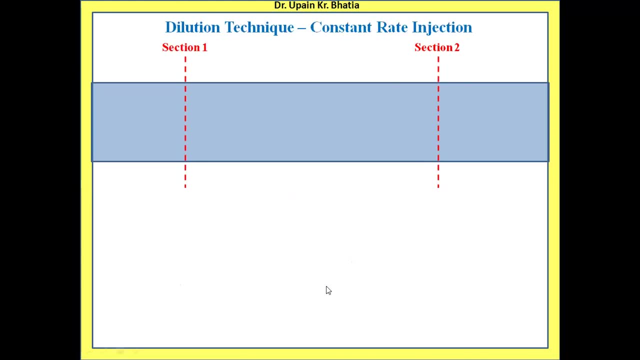 canceling. Here it is volume and here it is time. So volume per unit time. ultimately, this is going to give you the discharge Now. next is the constant rate injection technique. That means the tracer at section 1 is not released. all of a sudden That. 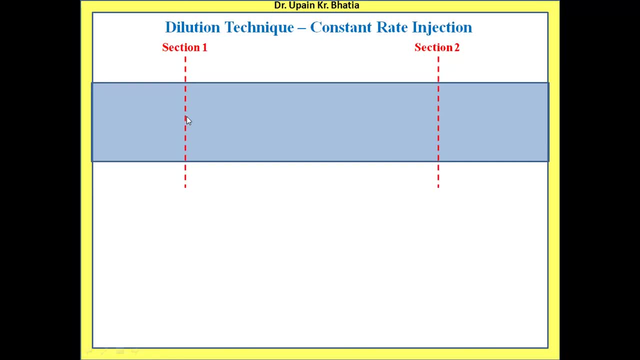 means you don't have to put all the tracer at once. Rather, you have to continuously inject it at a constant rate. So in that case concentration C1 is injected at the rate, at a particular rate. so rate of injection is Qt, So Qt is: 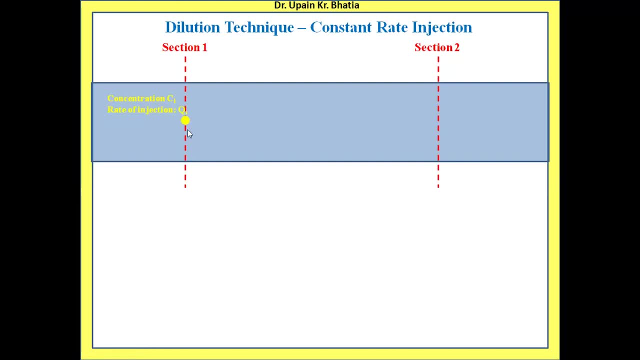 basically the discharge of the tracer, Because tracer is continuously discharged and released. So that rate is Qt. So when we inject it at a constant rate, then what you see is a continuous trail. Continuous trail of this tracer is there, But by the time it reaches section 2, 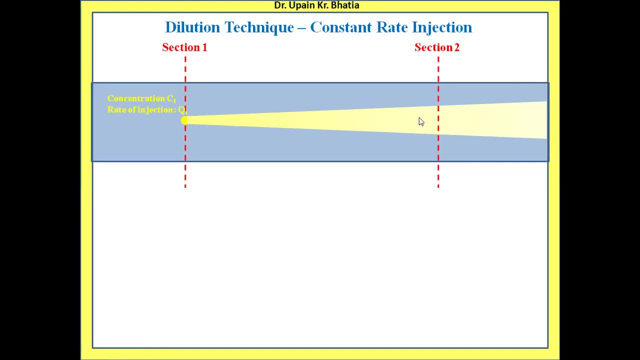 it is diluted. Okay, If you see again and just observe this leading edge, It is straight. I could not make it curved and so that it can progress also in the increasing fashion. But it will be same, as you can say it will be somewhat elliptical. 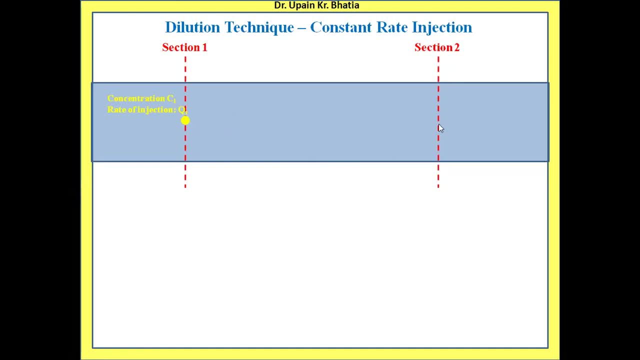 in the front, So that when it touches this point, the concentration will start increasing, and when it passes after certain time, a constant rate is there. So now the tracer is coming constantly and depending upon this length, a particular or specific dilution is achieved. So a 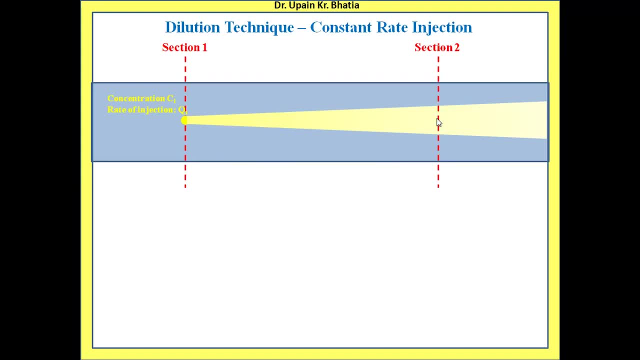 constant concentration will be observed at this after some time. Okay, So what you see is the diluted but continuous streak of tracer reaches section 2.. Okay, It is diluted but continuous streak is coming. It is not stopped from the back, because it is. 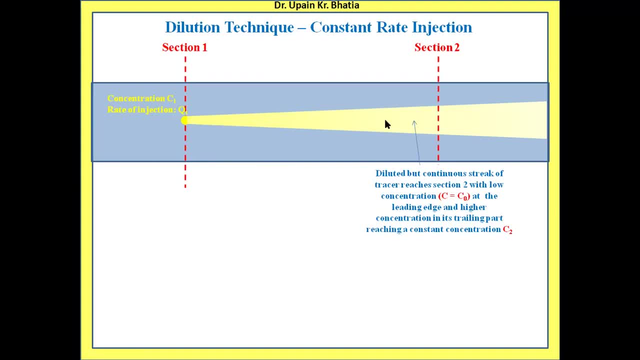 continuously being injected. So now the concentration is coming over here and it is a continuous streak With low concentration- C equal to C0- at the leading edge, which was leading the leading edge, and higher concentration in its trailing part, The trailing part of the leading edge. 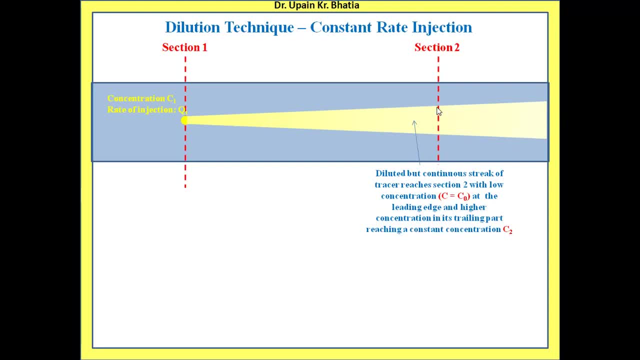 has its concentration comparatively higher. See, at any point, the concentration at the back is more here, the concentration is more here, it is more. So the trailing part at the back has more concentration. Now, if we see at this particular point, so we are getting. 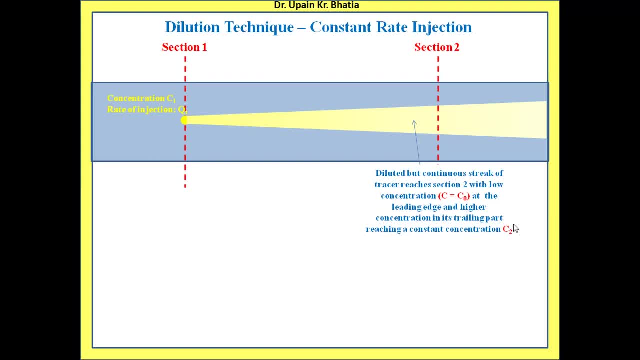 the concentration which is reaching at a constant value: C2.. Okay, While coming here, its value, concentration, becomes constant. It will not be reducing now, Like in a sudden injection at the peak value. it was reducing because the tracer was not coming from the back. 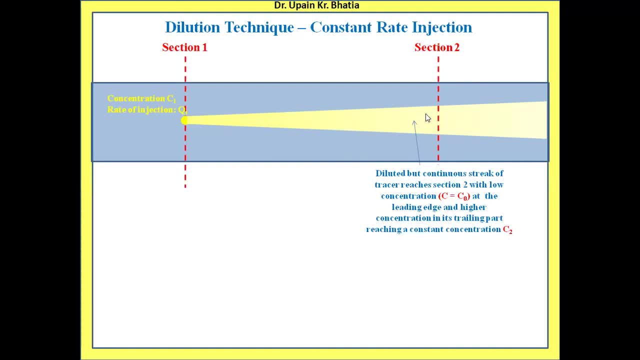 But here we are continuously injecting the tracer So that concentration will continuously reach over here and a constant value of the concentration C2 will be observed in this fashion. So this is the background concentration which was there in the water, which is already there in the water. So this much is. 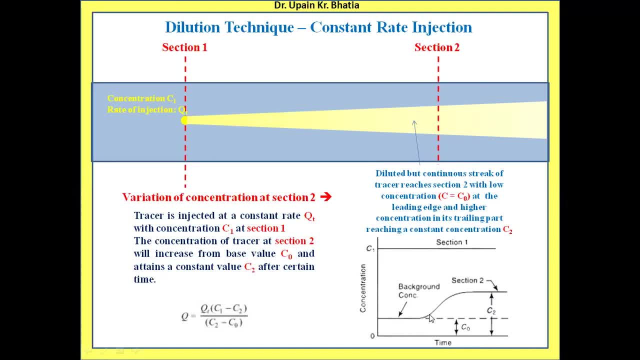 already there, which is C0. But after some time it has started increasing and attained a constant value. It is not coming down now. It has attained a constant value. And at section C1, at section 1- sorry C1- concentration is constantly being. 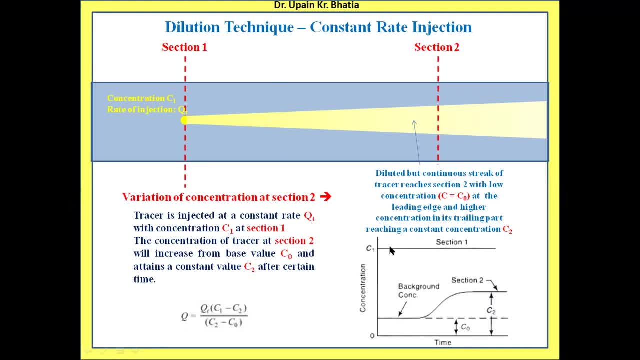 injected. In the previous slide you saw that it is all of a sudden injected and thereafter it was stopped. Just for a small period of time it was injected and then it was stopped. So here in continuous rate of injection, so this continuous line is observed over here. So 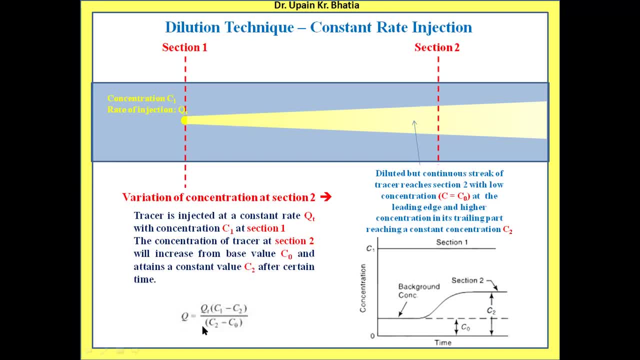 in this way. the discharge in the stream can be calculated by using this equation, where Qt is the rate at which the tracer is being injected, C1 is the concentration of the tracer being injected, C2 is the concentration at section 2 and C0 is the 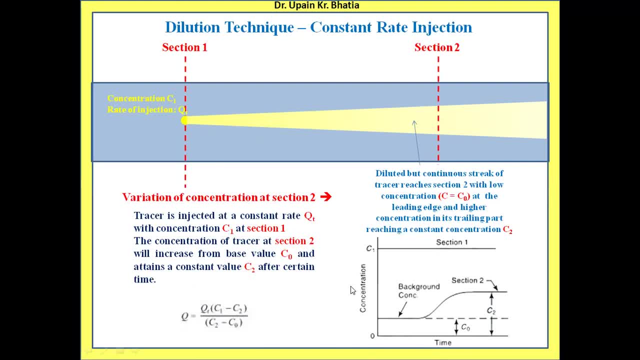 initial concentration, or you can say the background concentration of the tracer. So how we reach up to this formula, That you can explore at your own level, but ultimately this is the expression that we use generally for calculating the discharge in the stream. Now the third method is: 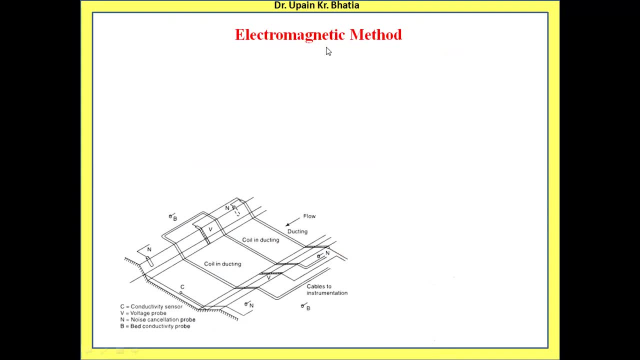 electromagnetic method. So this electromagnetic method, it forms the basis from the physics in 10 plus 1 and 10 plus 2, or in 10th class. even In physics we study the chapter of electromagnetism, or the magnetic effects of current or the electric effects. 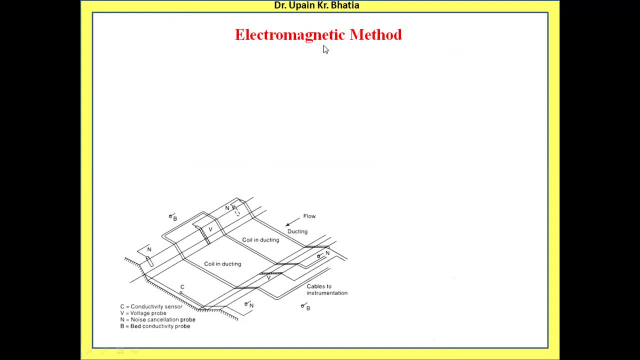 of magnets or their, let me say, electromagnetic effects. So what are these effects? It is based on the Faraday's principle. There are Faraday's laws, there are Faraday's principles, that EMF, that is, electromotive force, if you recall from the physics. 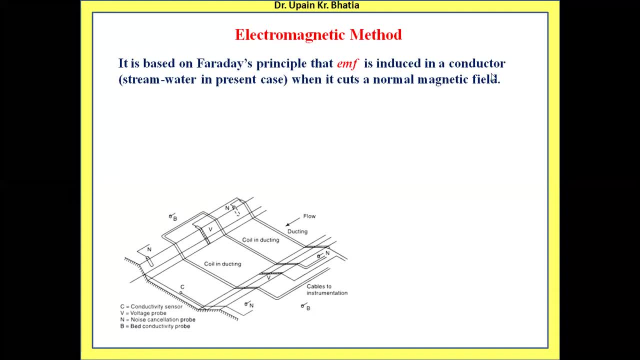 electromotive force is induced in a conductor when the conductor is cut the normal magnetic field, that means when the conductor is moved inside a magnetic field in such a way that the conductor cuts the magnetic lines of force, then some voltage is generated, which is called electromotive force. that 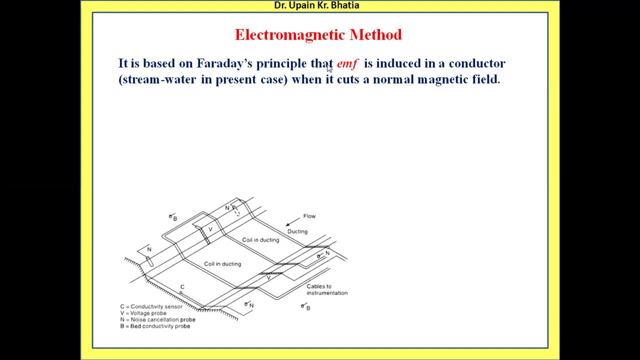 means some force is generated within the conductor which moves the electrons. that is why it is called electromotive force, EMF. it is same as the voltage. It is based on the Faraday's principle that EMF is induced in a conductor when it cuts a normal. 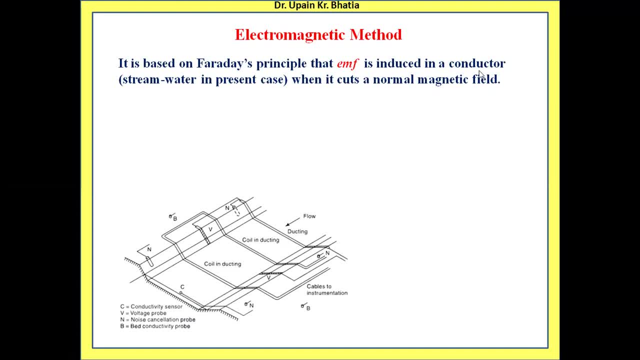 magnetic field. Normal means the direction in which the conductor is moving. the magnetic field is in the perpendicular direction and the conductor is cutting the magnetic lines of force. Now, this principle, Faraday's principle, which is generally used for generating the electricity in generators, that is being deployed. 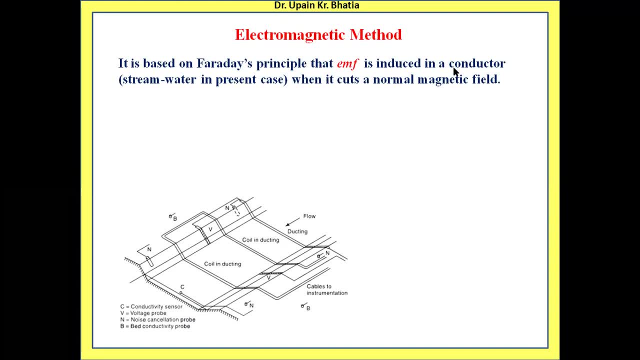 over here for measuring the discharge. so in the present case this conductor will be the stream water. Now the water which is flowing in the stream, that is basically conducting, because it has many types of salts and minerals which are dissolved, so that water is conducting. so stream water in the present 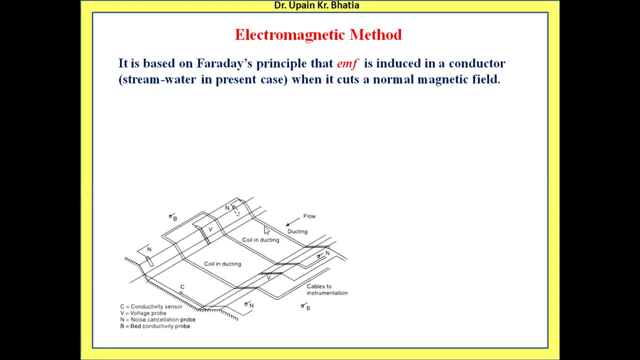 case, is acting as the conductor. Now in this diagram you are getting to know if you see it carefully. so we have a coil in ducting. ducting means that a coil is embedded under the duct. here a coil is made and what is there? so we have some. 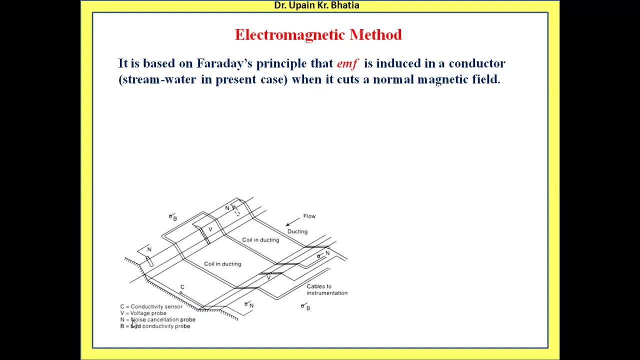 points like N and N. they are observation points like noise cancellation probes are there, B and B? these points are bed conductivity probes. C is the conductivity sensor- somewhere here we have installed the conductivity sensor also- and V is the voltage probe C. over here we have the electrodes which are voltage probes. 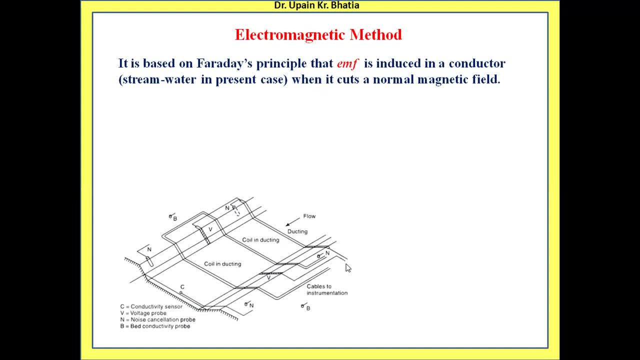 and these voltage probes are taken over here. so at these two points we can measure the voltage or the electromagnetic force that is generated. Now, what is its main concept? the vertical magnetic field is produced by current carrying coils which are buried under the channel. what does this mean? 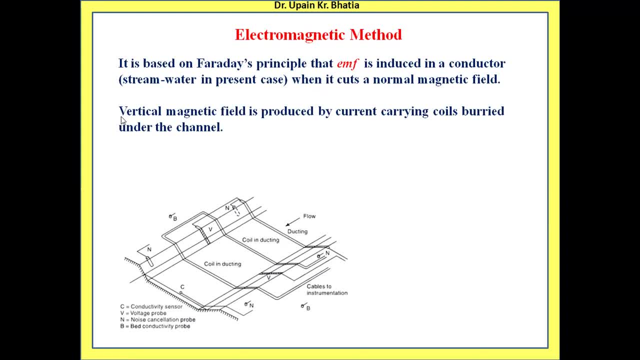 that we artificially produce the magnetic field in vertical direction. how will we do it? by passing some current in the coils which are buried under the channel. now, inside the channel we have buried these coils, and in those coils when we pass current, a magnetic field of this coil. 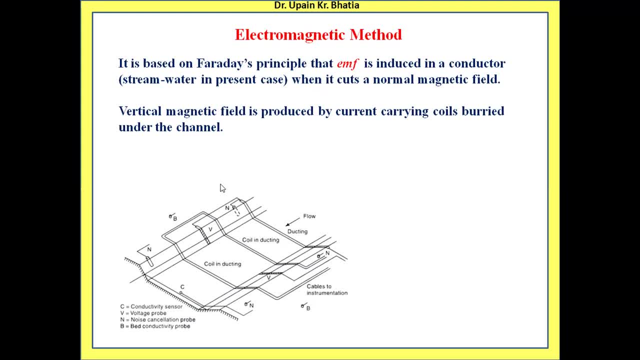 will be generated, whose direction will be vertical? now, the direction of the current, I will not tell here. if you want to find about it, then you can find it yourself. if current goes in clockwise direction, then what will be the direction of magnetic field? upward or downward? you can find it yourself. 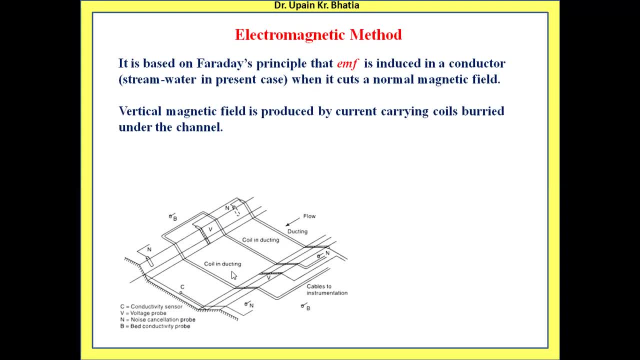 and if you will do it clockwise, then what will happen? you can make sure that the magnetic field will be vertical. so magnetic field is vertical and the flow of water is in horizontal direction. so definitely it is cutting the magnetic lines of force if the field is vertical. 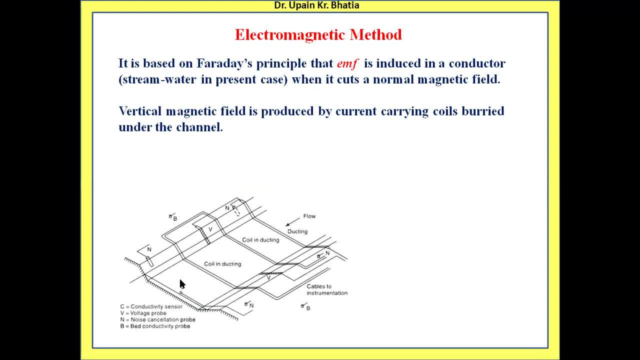 and in one horizontal direction there is flow, or conductor is moving, then the perpendicular across the channel. so this is the Faraday's principle. so now, across the channel, electromotive force or the voltage will be generated, and to sense that voltage, these two voltage probes are applied. 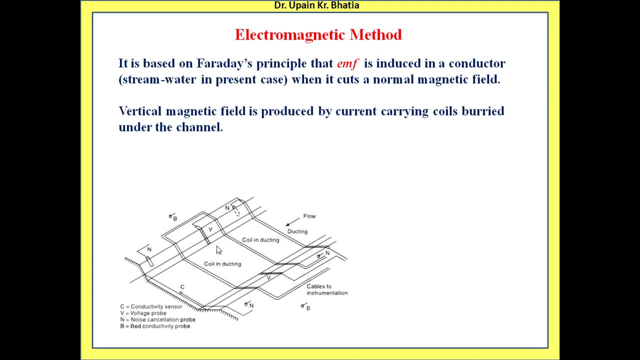 two electrodes are applied on both the banks which will measure this voltage. so now, on these two terminals, if we apply a voltmeter, a sensitive one, so it can give us the voltage or the emf which is generated, so electrodes measure the emf which is denoted by capital E. 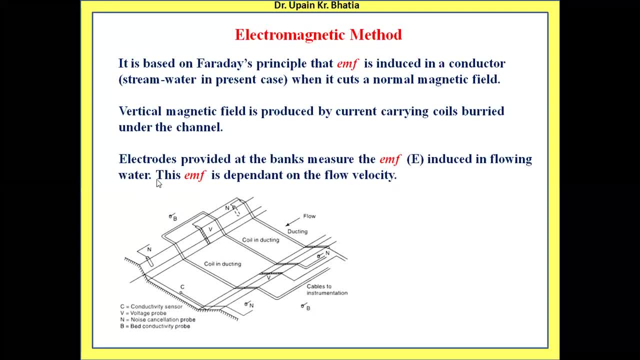 induced in the flowing water, which is denoted by capital E. induced in the flowing water, the emf which is induced in the water, or the electromotive force or the voltage which is induced. we have denoted it by capital E and this emf is dependent on. 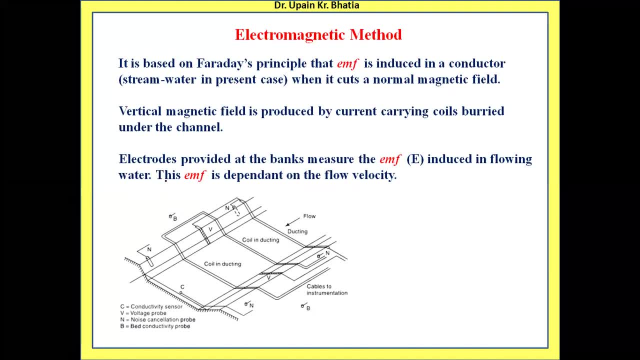 the flow velocity. now, if I explain this point in reference to physics, it is dependent on the flow velocity. you know that when the conductor is moved in the magnetic field, then electricity is generated, voltage is generated. but how much voltage is generated? that depends upon the speed at which 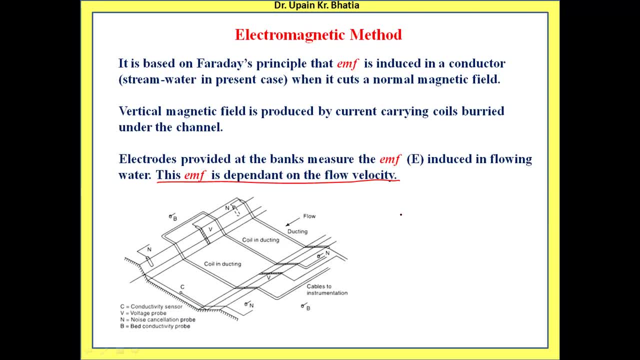 that conductor is moved. the faster you move that conductor, the more voltage is generated. so in this case, because that conductor is our stream water, because our stream water is the conductor, this conductor is the stream water. so to make it move faster means the flow velocity. if the flow velocity is more, 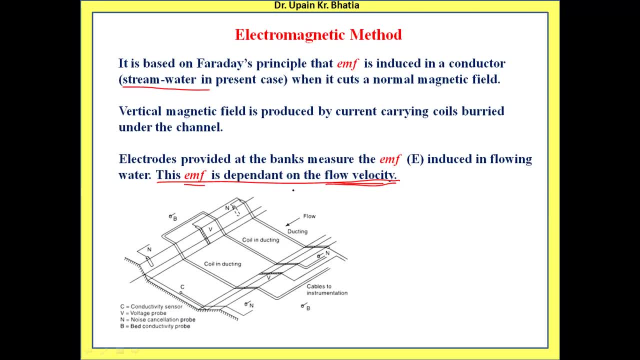 more emf will be generated. if the flow velocity is less, then lesser emf will be generated. so if you measure the voltage on these two terminals, then obviously you can get some idea about the flow velocity. now the discharge is calculated by this expression. discharge is equal to: 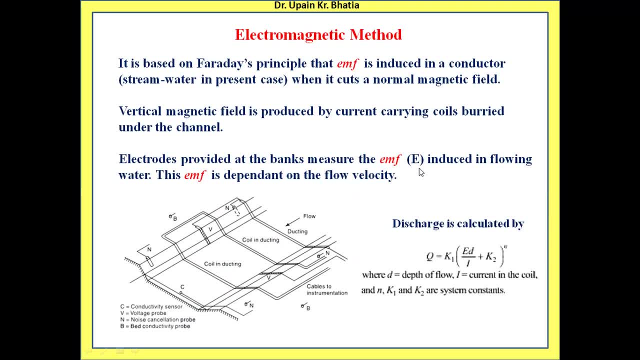 k1, e, ie, electromotive force d, which is depth of flow. upon this I, this is capital, I which is current in the coil, the current which we supplied in the coil, that current plus k2, whole raised to power n. now these n, k and k2. 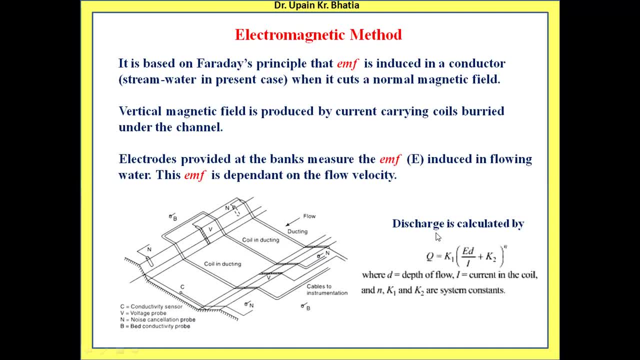 they are basically the system constants. so these system constants are dependent upon this total arrangement and various other, you can say the parameter or the observations, like conductivity and all. so it will depend upon them if k1, k2 and n, which are the system constants, they are known to you. 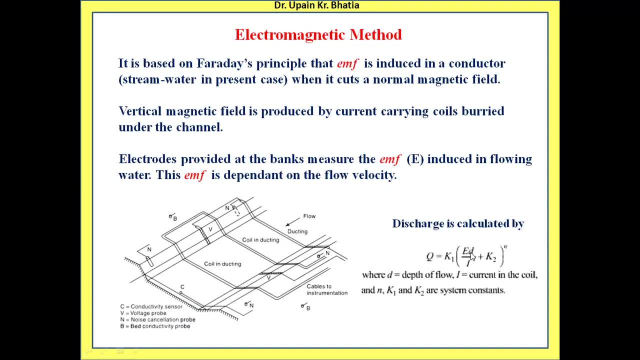 and if you apply some current depth of flow is known, current that you have supplied is known and you observe the emf generated, you can directly calculate the discharge that is flowing through the river. so this can be done just by sitting in the adjoining office or in the room. 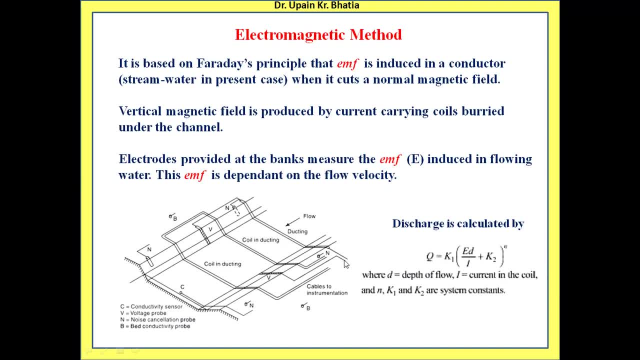 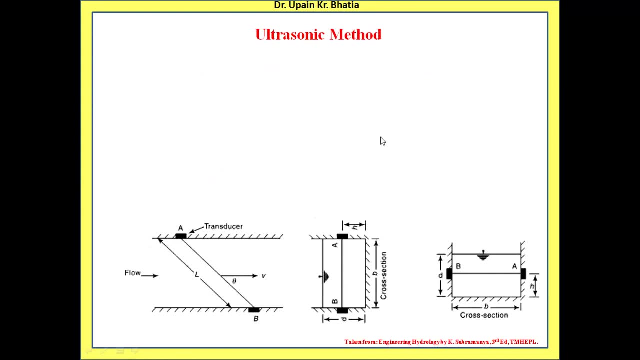 from that control room only, you are just applying some current and within that control room only you are noting down the emf. so likewise you can use this electromagnetic method also for measuring the discharge. now the next method is ultrasonic method. so ultrasonic method, if you see. 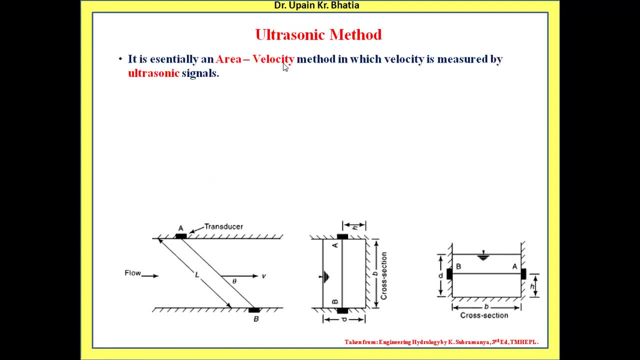 it is essentially an area velocity method which we will discuss later. area velocity method means area is to be multiplied by velocity, so it is essentially an area velocity method in which velocity is measured by ultrasonic signals. now, what is done for that? if you view the river, 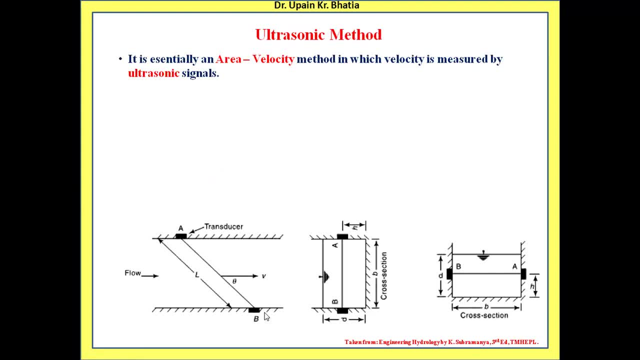 or the stream from the top. so these are overall two banks. at one place, one transducer is applied, whose name we have kept as A, and on the downstream side, in the opposite direction, on the opposite bank, another transducer is applied, B, so that the distance between 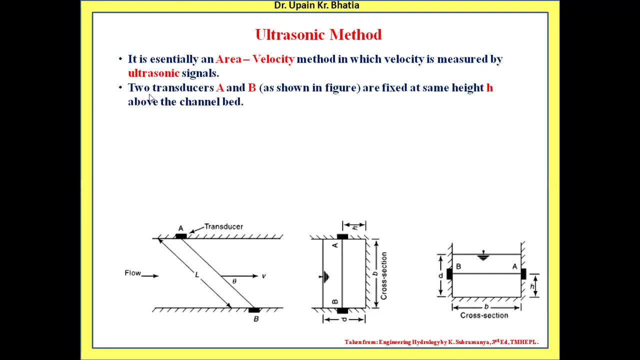 let us consider this point first. two transducers, A and B, are fixed at same height, H above the channel bed. this method is generally more applicable for rectangular channels, channels which are of rectangular shape, or wide rectangular channels in which depth is same everywhere. there is no irregular depth. 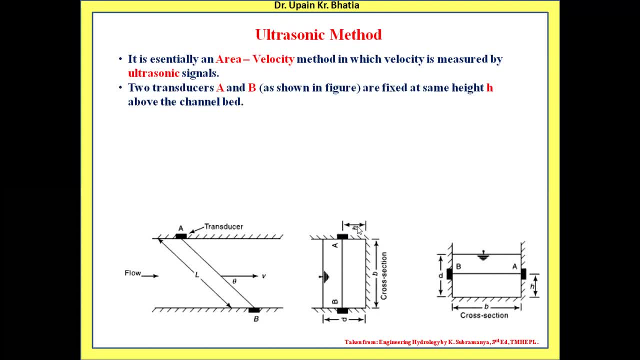 so in this case, from bottom to H depth, we have applied transducer A and B. this is the cross section if you view from this side. this is because, according to this view, if you turn it, this is the cross section. this is rectangular cross section. transducer A. 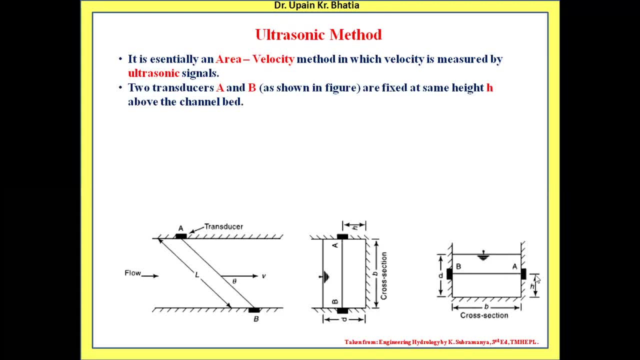 and transducer B. both are fixed at height H above this bottom and base width is small b and depth of water is small d. so at what depth we have to fix these transducers so that it gives us the average velocity, like if from top, say 0.6 d? 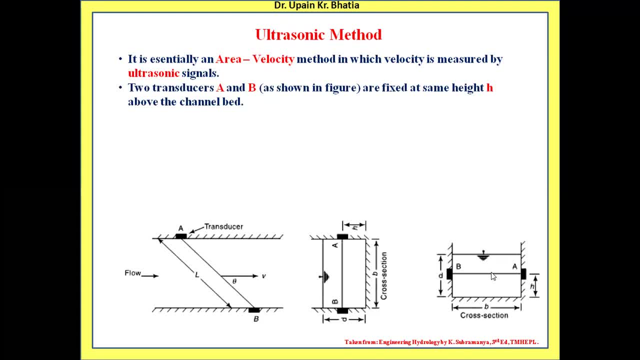 d is the total depth, so if we set it at 0.6 d, so whatever velocity we get, that will be the average velocity anyways. coming to this system again, so distance between A and B is L, as seen in this diagram, and the angle made by 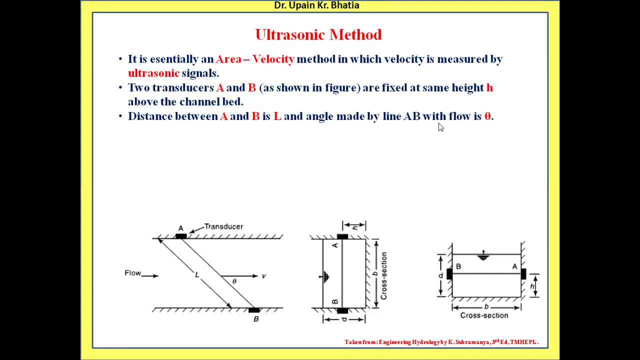 the line AB with the flow is theta, so flow direction is this. so this line AB is making an angle theta, so these transducers can emit as well as receive the ultrasonic signals. now these transducers, now the word transducer is mostly used in electronics in general. 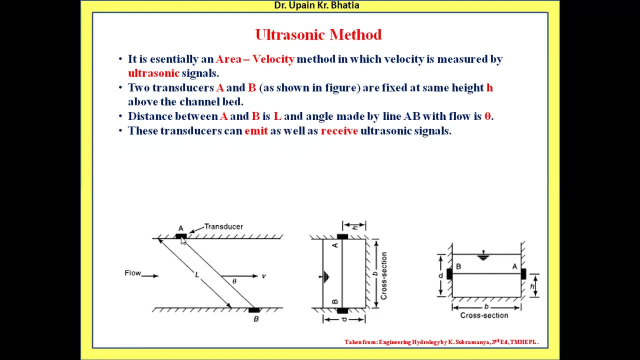 transducers in general. if we tell you what is transducer, so transducer is such a thing which converts one form of energy into another form of energy. so, if you see, we use these transducers very frequently, like tube light or LED bulb. if you see that setup. 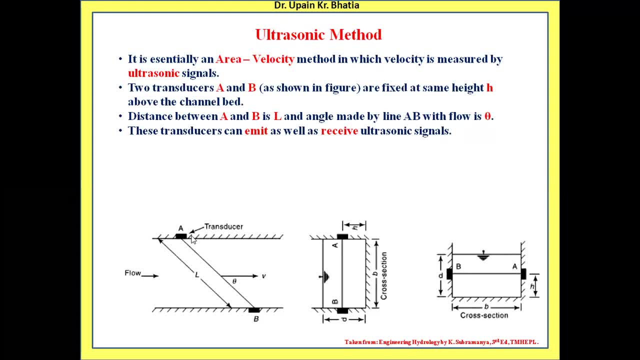 that acts as a transducer which converts electrical energy into light energy. as of now I am speaking, so whatever I am saying, mic is such a transducer which converts sound energy into electrical energy, ultimately as soon as it is transmitted to you, so in your system, whether it is mobile phone. 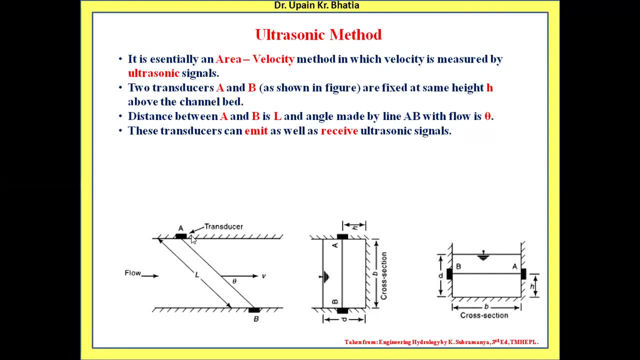 or laptop, whatever you are accessing, you are listening through speakers so that sound is transmitted to you in the form of waves and your system again converts it into electrical signals and gives it to the speaker. and speaker is another transducer which converts it into sound which you can hear. 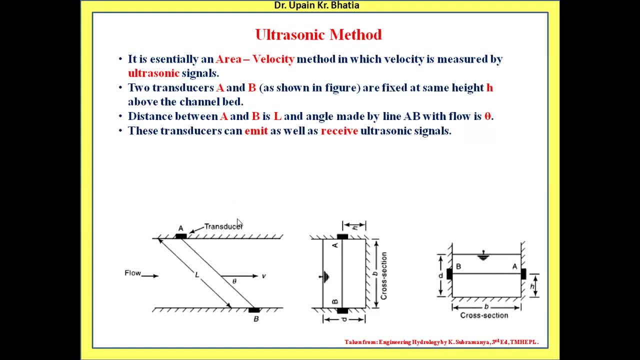 so all these things are basically the transducers. so here this is also a transducer which converts electric pulses into sound waves. but the frequency of sound is more than the frequency of listening, so we call it ultrasonic sound. we will call it ultrasonic signal. so that means 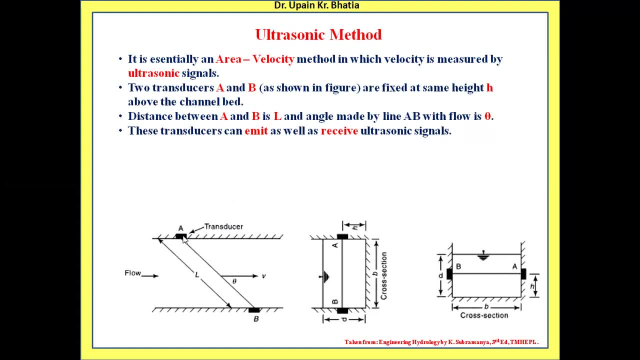 this transducer converts electrical signals into ultrasonic signals, and this is a dual character. it not only converts electricity but can also convert sound into electrical signals. so this is a dual. so these transducers can emit as well as receive ultrasonic signals. so first, A is our transducer. 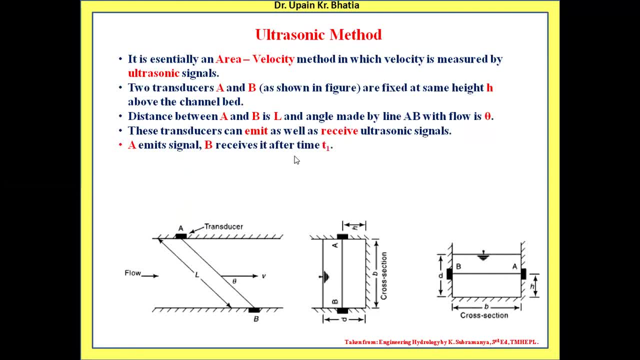 it emits the signal, B will receive it after time T1, because we have the control of both these transducers. so as soon as A is received, our system emits an ultrasonic signal and after moving L distance, it reaches B and B receives it as soon as B receives it. 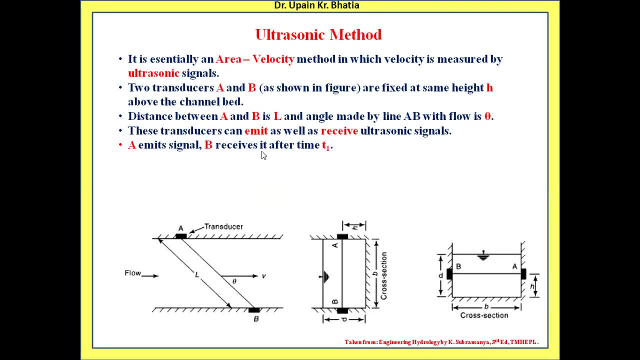 our system notes it. yes, B has received this signal. and in this whole process, the total time that took for emission and reception, that is T1. and then B generated that signal control panel. our control system triggered B, B emitted that signal and A received it. and to go from B to A, 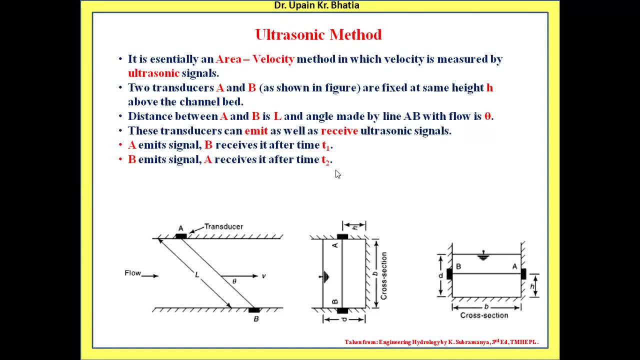 it took time T2, because this distance is again L in both the cases. the difference in these times T1 and T2, that is because of the flow. if it is a still water, then these time T1 and T2, both will be same, but this flow is. 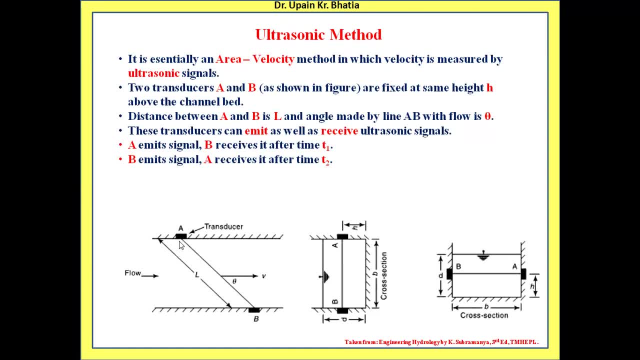 flowing left to right, its component. if we see A to B, this direction is assisted by this component. so time T1 will be lesser. but if the signal has to travel from B to A then this flow velocity is opposing it. it is trying to oppose the flow of signal from B to A. 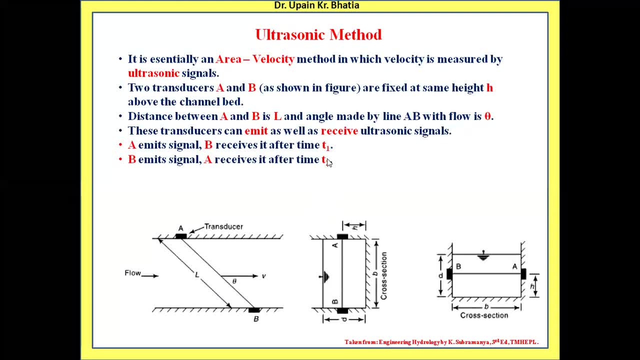 so it will take more time. so the difference in these times, that is basically the reason for calculating the discharge. so the flow velocity is calculated by using the formula this one: L is the distance, theta is the angle of that line, AB, with flow velocity 1 upon T1 minus 1 upon T2. 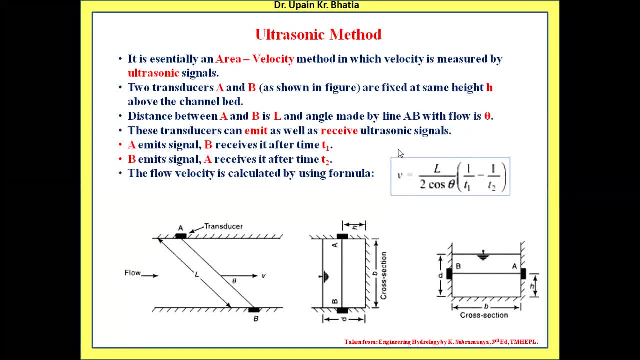 ok, so 1 upon T1, because T1 value is lesser, T2 is more, 1 upon T1 is higher and 1 upon T2 will be lesser. so higher minus lesser, it is going to give you a positive value. so this V is going to give you. 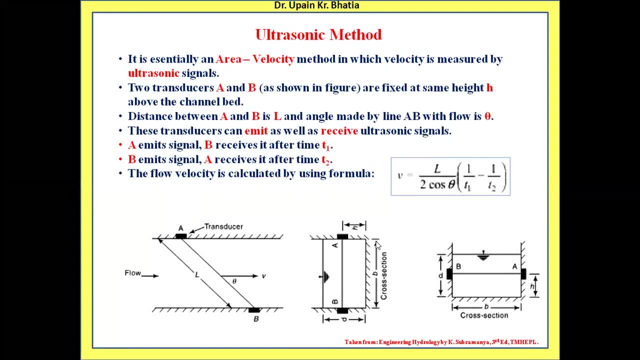 the velocity of the flow at the depth, at the height H above this bottom, ok, from this bottom H height, on which level we have fit these transducers. so, on this height, what is the velocity of this stream? so, if we up or down the whole setup, if its depth is more, 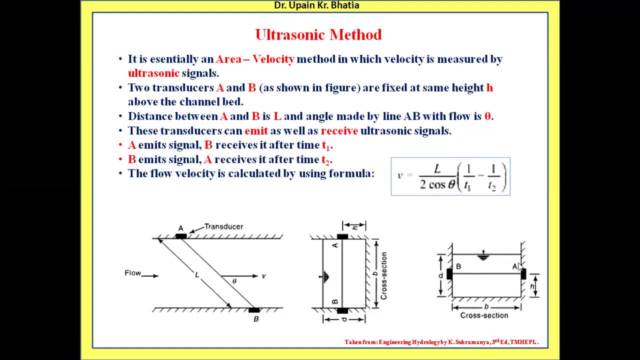 more than the shallow river. so we will set it twice, once on 0.2D and once on 0.8D. so we will work out two velocities and take their average. so this was discussed in the previous lecture. if you have any doubts, then you can watch it again. 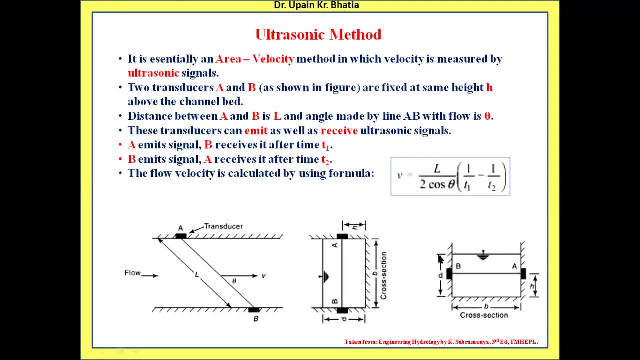 ok, once you have the velocity, then you have to multiply with the area area of cross section. is this B multiplied by D, so this area multiplied by the average velocity, V, that is going to give you the discharge which is flowing through this channel. so this is basically area velocity method. 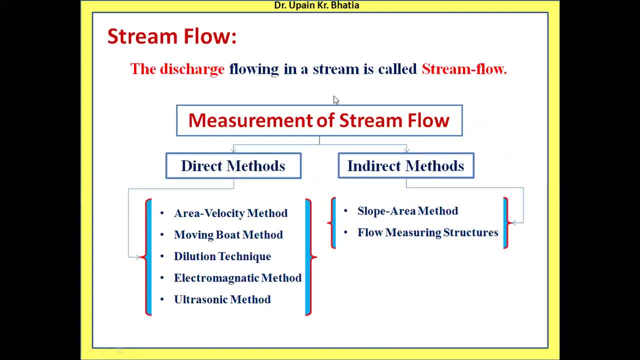 now moving again to the same slide that we saw initially, so moving boat method, dilution technique, electromagnetic method and the ultrasonic method- they are covered. now we are going to discuss about area velocity method, so this is the method that we are going to discuss now. 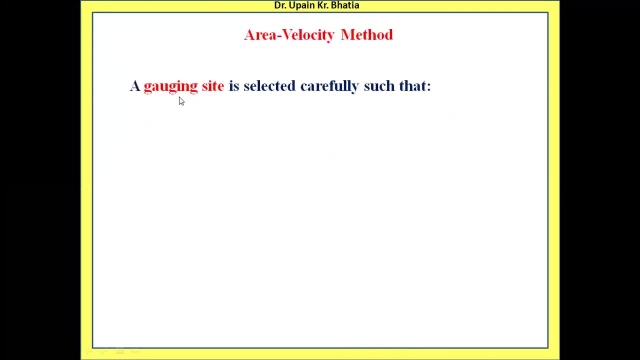 so, if you see, we have to take a gauging site. gauging site means where we measure this discharge. so gauging site is to be selected. so how to select it? it is to be selected carefully so that these four points are satisfied. so it should be well defined. 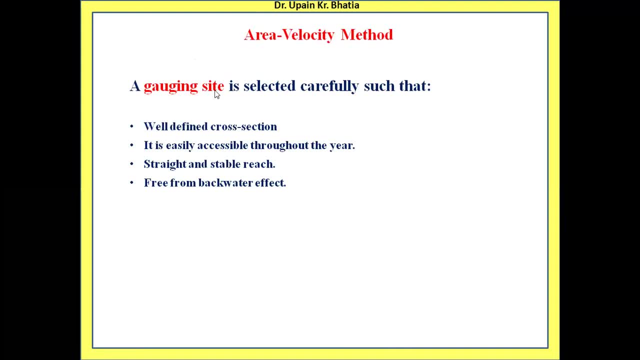 cross section. whatever cross section we have to take on any gauging site, that should be well defined cross section. that cross section should not change again and again. there should be only one cross section we prefer generally. the rocky terrain means river cross section in such a portion of river. 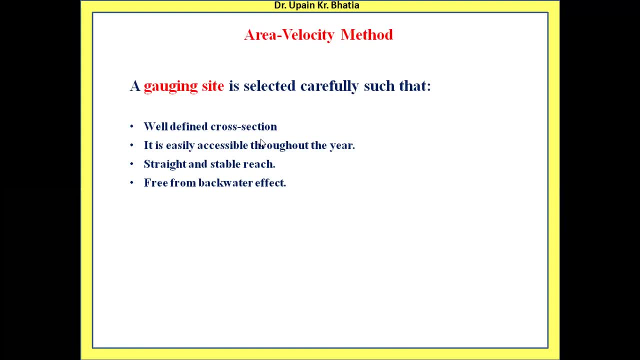 where in cross section, rocky banks or rocky bottom, which does not erode out much and more or less it remains same side and cross section. next is it is easily accessible throughout the year. it should not be accessible at any particular time of year, so it should be accessible. 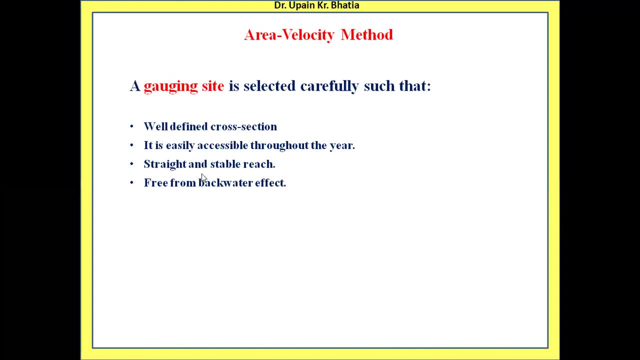 throughout the year. comparatively straight and stable reach should be before and after. comparatively straight reach means the length of the river should be almost straight. in that area. it should be free from the backwater effect, like in the bottom or on the bed or in the banks if there is any protrusion. 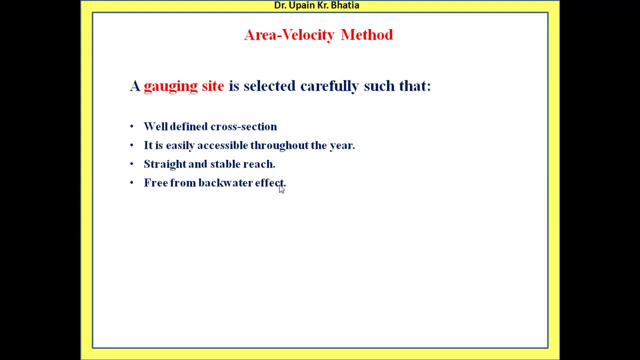 or rock, from there you get some backwater effect, or if there is any turn due to that, you get some backwater effect. so that is going to give you erroneous results. so generally we avoid such sites where the backwater effect is there. so our gauging site should be: 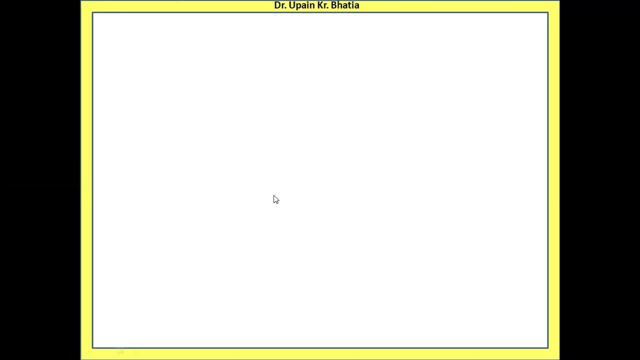 free from the backwater effect. now let us say this is the cross section, this is the river cross section, it is irregular cross section and this is the water surface. so this is the overall cross section area. now this is the vertical that we talked about in moving boat method also. 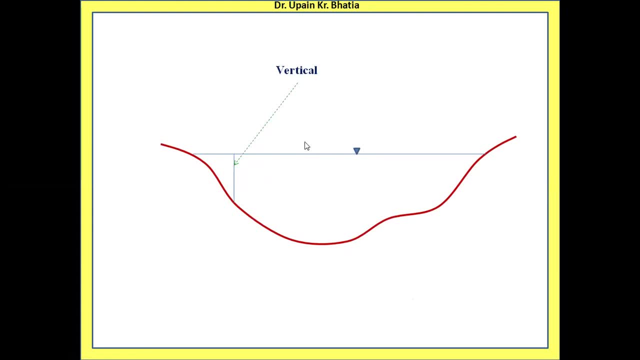 now we are looking at the cross section of the channel, not from the top. so this is the vertical line, which is simply called a vertical. so these are more verticals. so we basically divide this entire cross section with the help of these verticals. this is not one vertical. 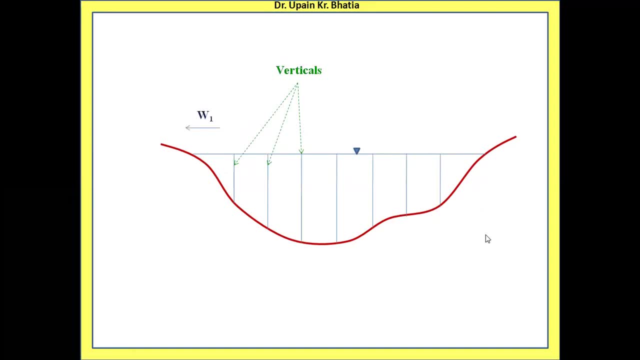 so there are number of verticals which are generally used. so if you see the distance of first vertical from the bank, that is W1. distance of second vertical from the bank, that is W2. similarly, if you see intermediate from ith vertical, the distance will be WI. 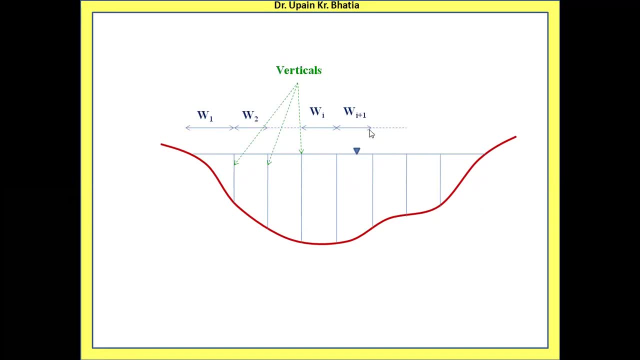 I plus 1 vertical W1 plus I plus 1 and ultimately we reach the other end where last one is WN and prior to that is WN minus 1. so these are various width between, or width of the river section or the channel section between these verticals. 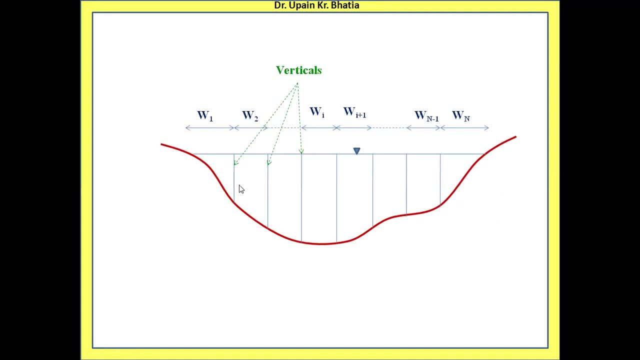 ok, now at a particular vertical, if you see, the depth depth of the vertical is generally determined by some acoustic acoustic meter depth meter. you release the ultrasonic sound, it comes back and gives you the depth value. so if this depth is, say, less than 3 meters, 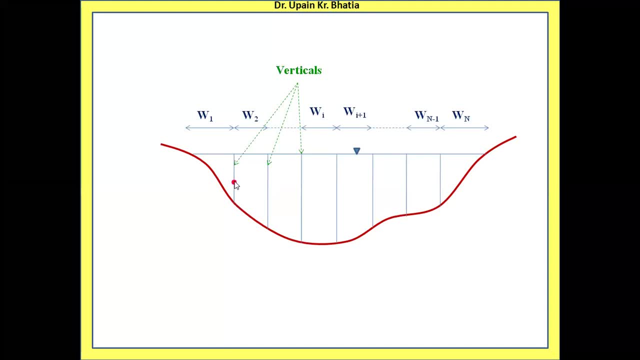 we can consider this to be shallow water over here. so we can take a single point at the depth 0.6 times this total depth of this vertical, so that we can measure the velocity at this red dot or this point similarly for the next vertical. this is the point. 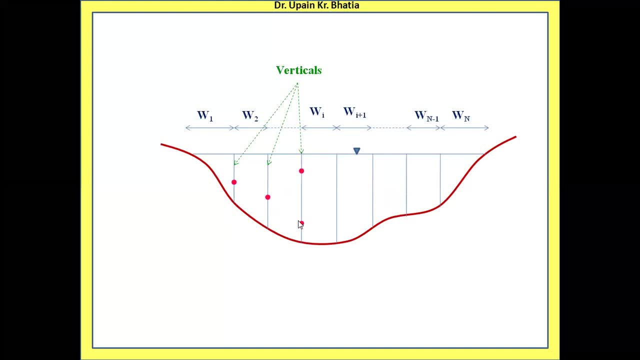 here the depth has increased, so let us take two point methods at 0.2D and 0.8D. so these two point observation method will be used at this vertical. similarly, we can select how many observations are to be taken at each vertical. so 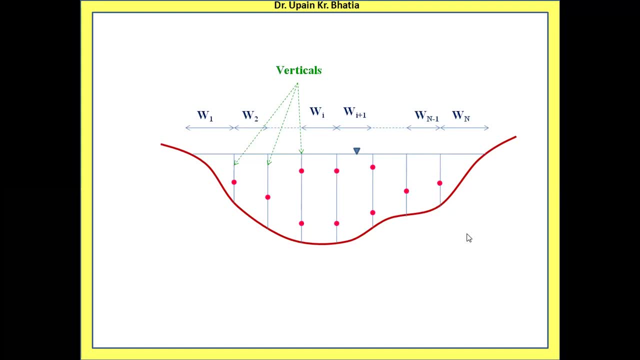 and on all these red dots, we basically measure the point velocities by using current meters. so in this particular method, we assume that we either we have the velocity values or we have some information so that velocities can be calculated at these points. now what you see is that 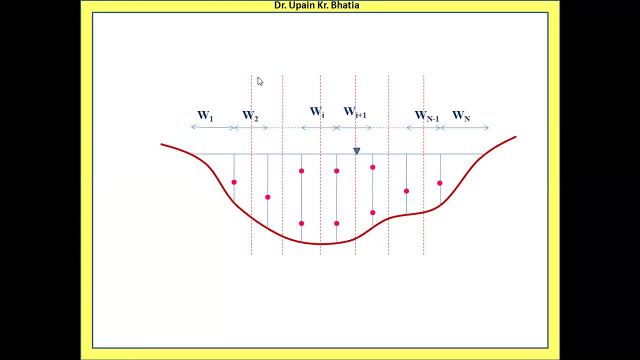 we have divided this reverse section with the red dotted lines also. so we have divided this reverse section with these red dotted lines also. and these red dotted lines are passing from the middle of these two verticals. that means from one vertical to the other vertical, somewhere in between. 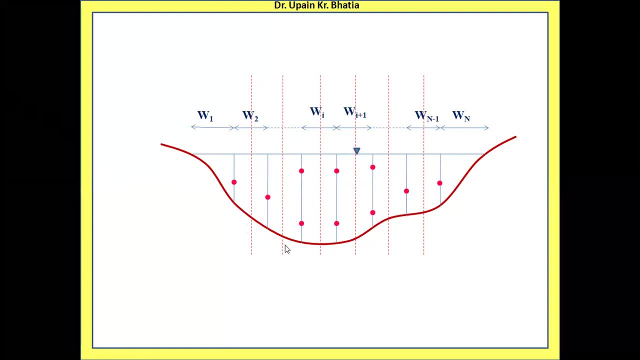 this red line is passing and then this next red line is passing. so the purpose is to divide this entire river cross section in such a way that from one dotted line to the next dotted line in between, it is enclosing certain area, and in that area we have at least one. 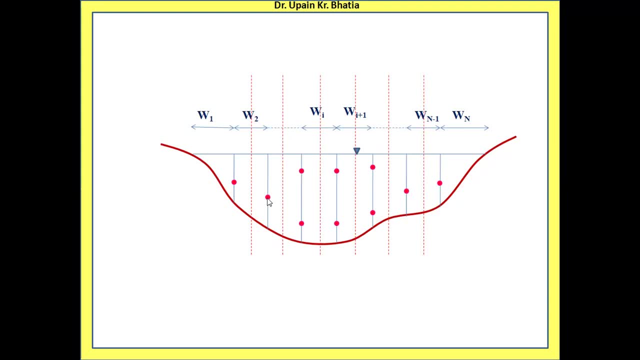 velocity, one point where the velocity is either known or it is measurable, or we have the data so that this velocity can be calculated, like from this dotted line to this dotted line. we have these two points and velocities at these two points is either known or we have. 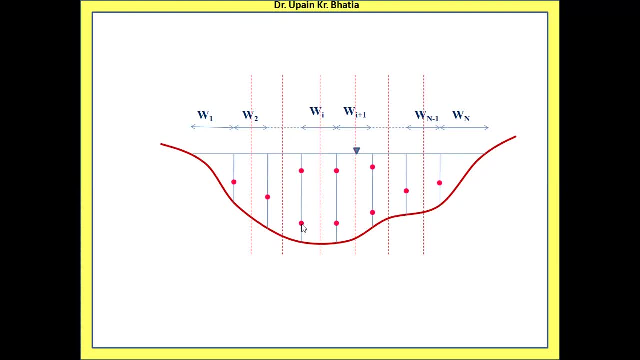 the information to calculate these velocities at these two points and ultimately we can calculate the average velocity within this area. so this is the first segment of the area, cross section area, which is at the end, so it is called the end segment. similarly, on the other side also. 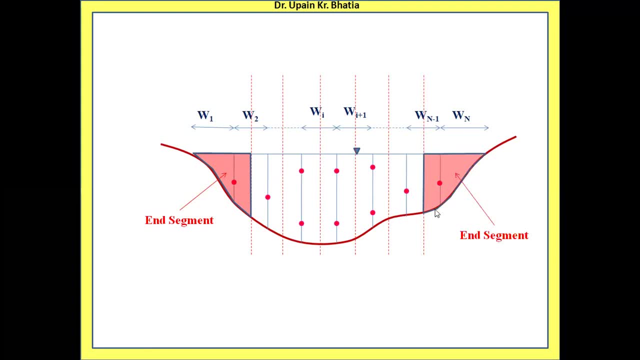 it is the end segment, okay, so in if you start measuring the distance from this left bank, so this is w1, this is w2 and the last one is wn and before that it is wn-1. and if you measure the distances from the right end, 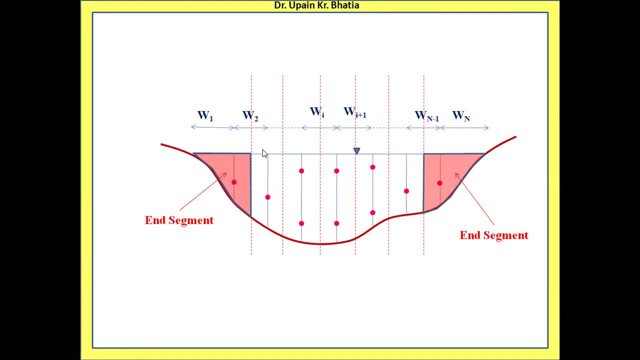 then this forms w1, this is w2 and this is wn-1 and this is wn. so basically the end segments. both are treated in the same fashion. somewhere in between the intermediate segments are between these red dotted lines and one represented by the negative intermediate segment. 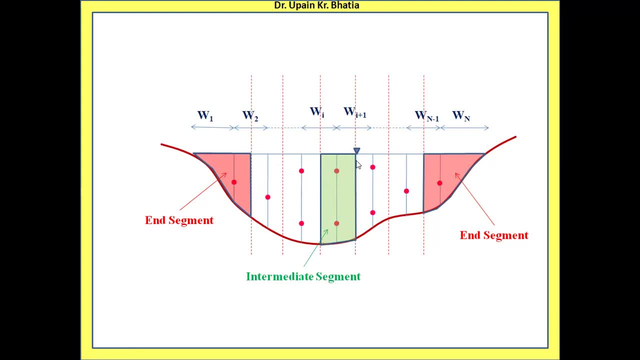 is shown in this green color. so this green shaded area is basically the cross section of this segment, with two points in between for the measurement of velocity. now we have to measure the effective width of this segment, so it is appearing that this w1 bar is equal to this. 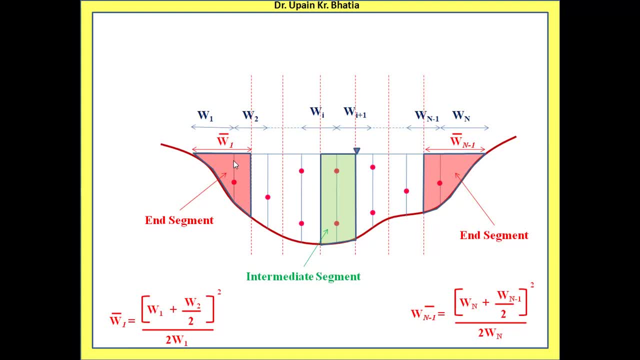 w1 plus half of w2. but it is at the bank so a special procedure is there. so w1 plus w2 by 2, that means w1 is taken complete and half of the w2, because half of w2 is on this side and half is on the other side. 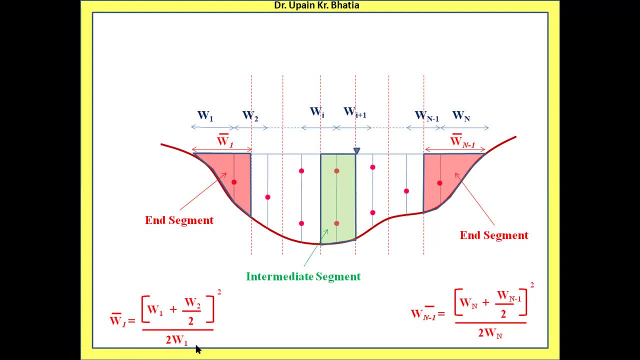 so half of the w2 is taken. then square it and divide it by twice the end width, okay, w1. similarly on the other side, if you see, same treatment is to be given because it is the end segment. so wn minus 1 bar, that will be equal. 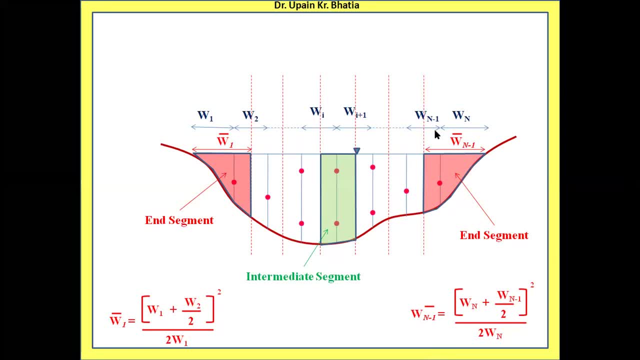 to wn plus half of wn minus 1, divided by twice of this end width wn, because it is squared and divided by twice of wn. so same treatment is given to the right side also. so if you just remember this expression, same expression is to be generated for the other side. 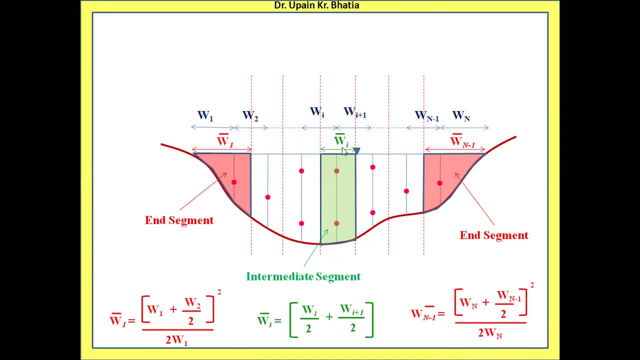 for the intermediate one at a distance, say with segment will be width of wi, segment will be wi bar, which is equal to half of this side, half of this wi and half of this wi plus 1. so both are halved and added together so that this wi bar. 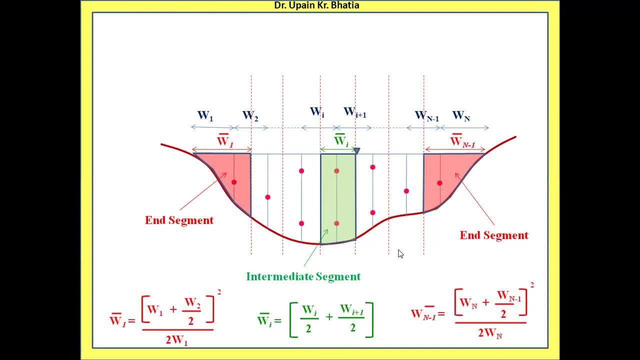 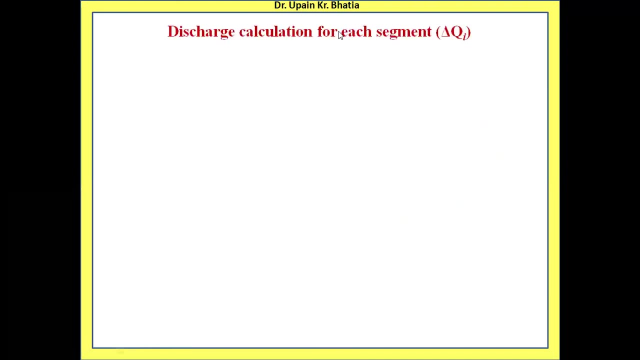 is computed, so this one is simple. so once you know the width of end segments and intermediate segments, then one by one, we calculate the discharge into each segment. so discharge calculation for each segment, that is delta qi, that is area of the segment multiplied by the average velocity. it is a simple method. 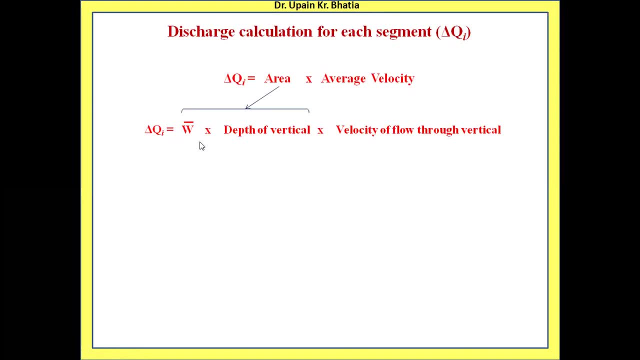 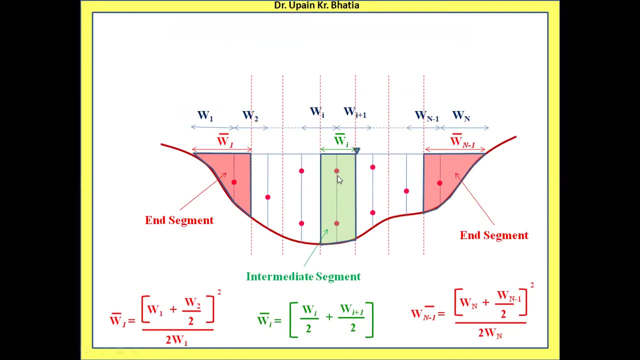 that is equal to this portion is area, which is average width multiplied by depth of the vertical. if you see, this is the average width and this is the average depth of the vertical, because it is in the middle. so we adopt this depth of the vertical that we already have noted. 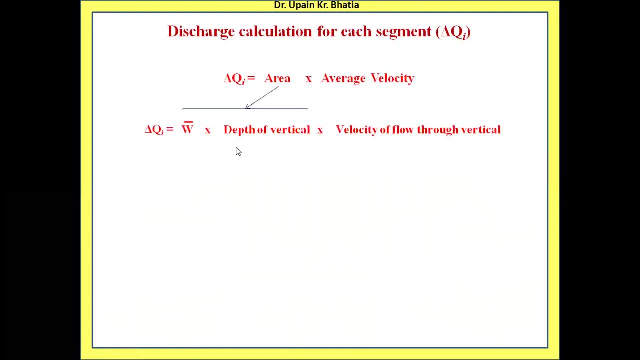 and so depth of the vertical multiplied by w bar, that gives you the area of the segment multiplied by the average velocity, which is velocity of flow through that vertical. and this velocity is taken as the average velocity as determined by either floats or by the current meters. ultimately, 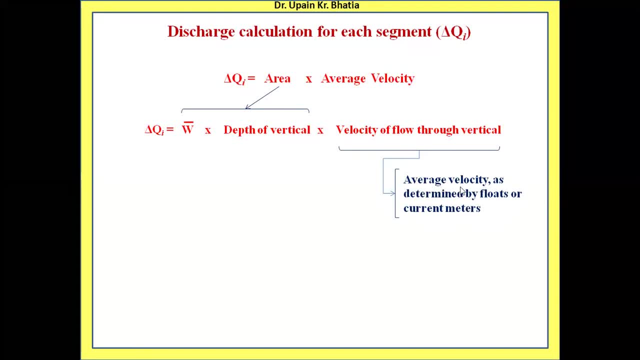 we have to take the average velocity. and how to take this average velocity from floats or by current meters, that was discussed in the previous lecture. so the total discharge that will be equal to sum of all delta qi values. so for all the segments we know some values. 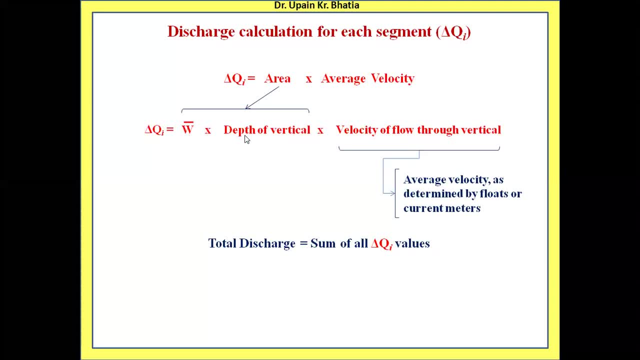 of w bar and we know the depth of vertical. every segment is having one vertical in it and depth of that vertical is to be taken and every segment is having some information for measuring the average velocity, so that velocity is to be multiplied by this area so you will be able to. 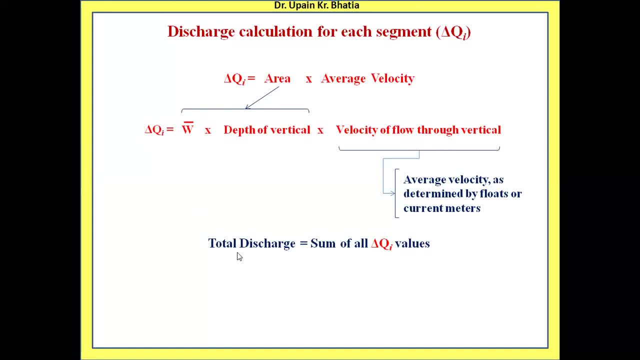 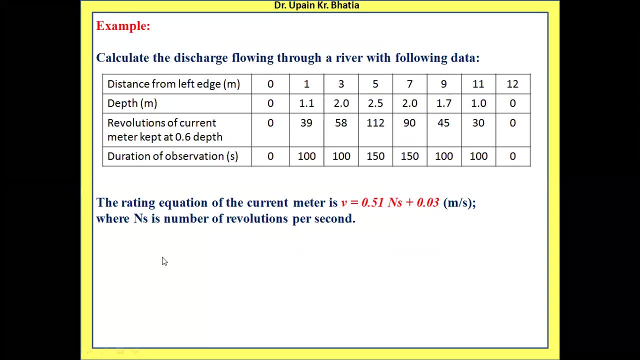 work out the discharge in every segment. so the total discharge will be sum of all these delta qi values. ok, so let us consider one numerical. if you see this numerical, if you calculate the discharge flowing through the river, this data is given to you. so, distance from the left edge: 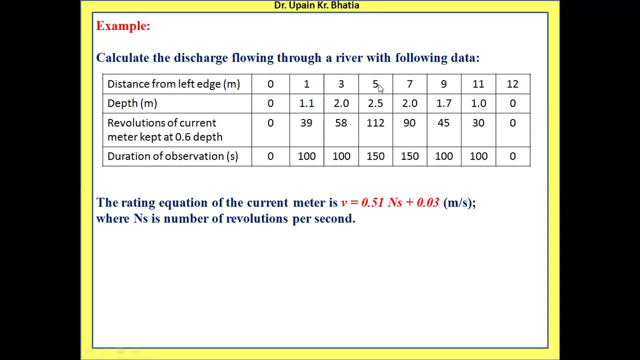 is given 0 meters, 1 meter, 3 meters, 5, 7, 9, 11 and 12, so intermediate, if you see, at the distance of 2 meters, each at the gap of 2 meters, but the end one is at 1 meter here. 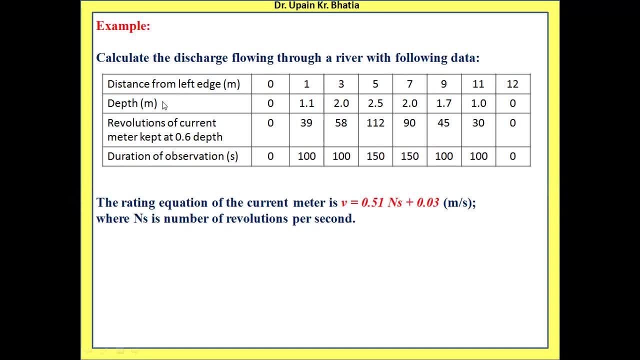 and 11 to 12. it is also 1 meter distance, 1 meter gap, so depth are measured from left edge and just at time, at distance 0, where the water surface is just touching the ground, here the depth will also be 0, and at all other distances. 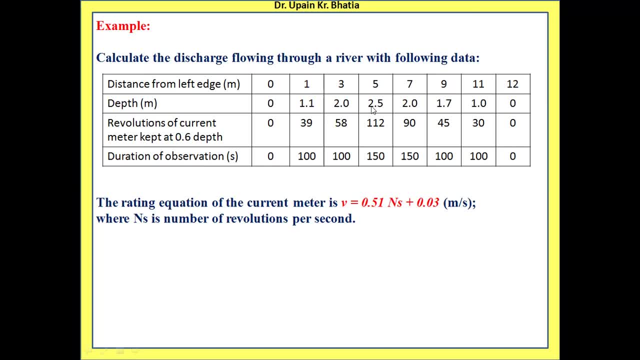 the depth are given to you as 1.1 to 2.5. again it is reducing to 2, 1.7, 1 and ultimately 0, because 0 is the depth at the other end. so 12 meter. so this total information: 0, depth at 0. 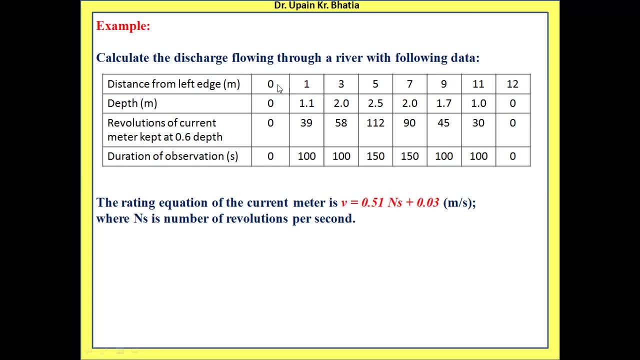 distance and 0 depth. at 12 meter distance, it gives you that the total width of the river is 12 meters over here. what further information is given to you is the revolutions of the current meter kept at 0.6 depth. if you see carefully, it is 0.6 times. 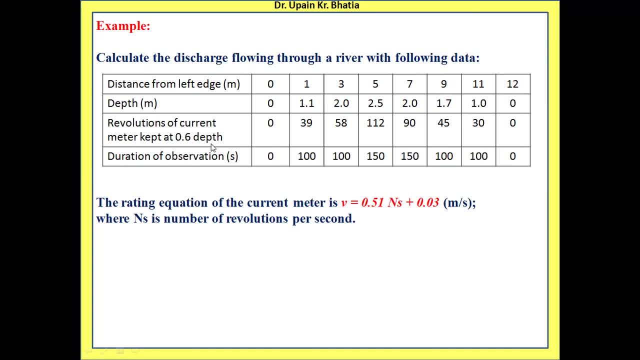 depth. that means this observation is directly helping you to find out the average velocity, so number of revolutions of current meter, and to note those revolutions. how much is the time duration that is also given to you. that means, let us say, at a distance 5 meters from the left edge. 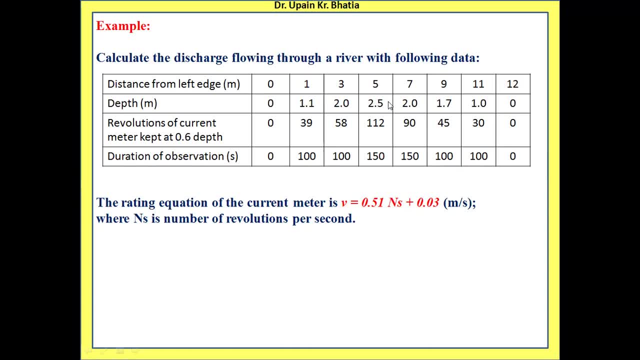 which is vertical, that vertical depth that is 2.5 meters, and that 2.5 meter- 0.6 times that. this value, current meter, was lowered into the stream and there 150 seconds continuously its rotations were counted and in that 150 seconds. 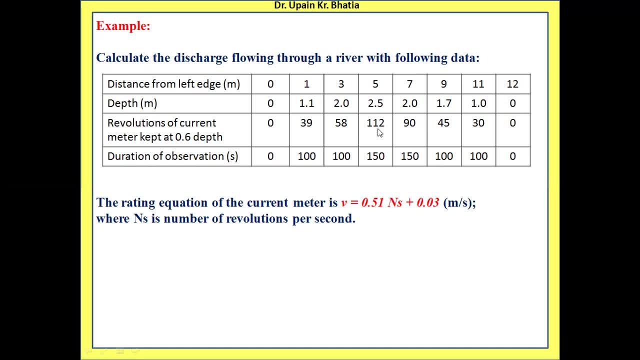 112 rotations or revolutions were recorded of that rotating element. so what is this information? this is basically information to work out the ns value, or the rotations per second value. number of rotations per second. ok, if you recall, every current meter has a calibration equation, which we also call rating equation. 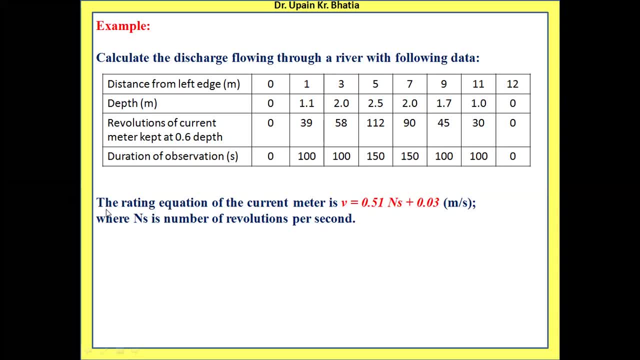 so here, what else is given to you is that the rating equation of the current meter is given as velocity v is equal to 0.51 ns plus 0.03, and the units of this velocity will be in meter per second. that means this rating equation. 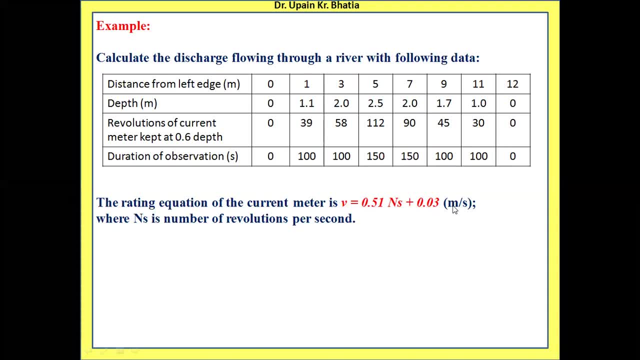 will be giving you the velocity in meter per second if you use ns as the number of revolutions per second. ok, number of revolutions per second, not per minute per second. here, fortunately, this data is given as number of revolutions and the duration in seconds. so if you divide this number of 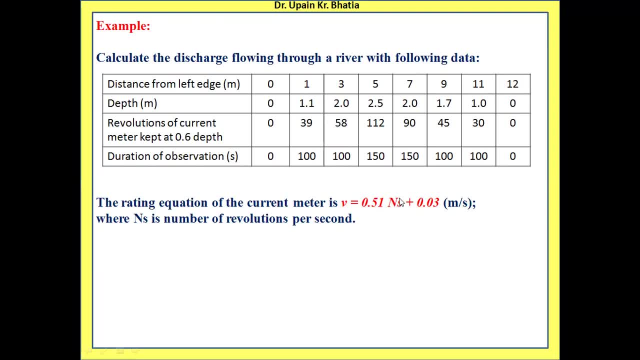 revolutions. with this duration, you will directly get ns value, ok, and if you put this ns value over here and calculate it, it is going to give you velocity in meters per second. ok, so this information is sufficient to work out the velocities. depth is also given and the distances are also given. 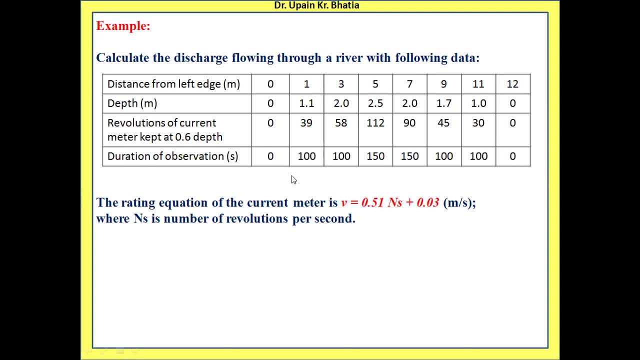 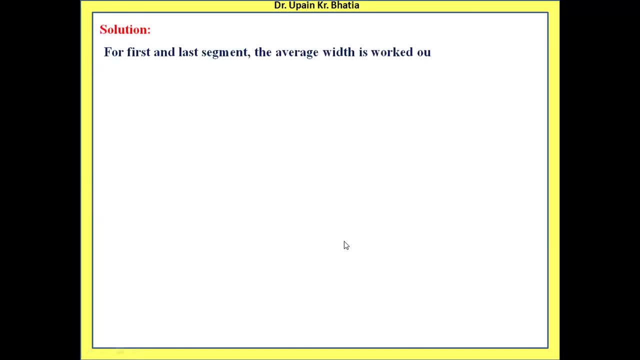 so what you need to do is to work out w bar values. remaining thing: everything is almost very crystal clear. so let us move further. for the solution for first and the last segment. first segment is, say left side segment, and the last means the right side segment, the end segments I am talking. 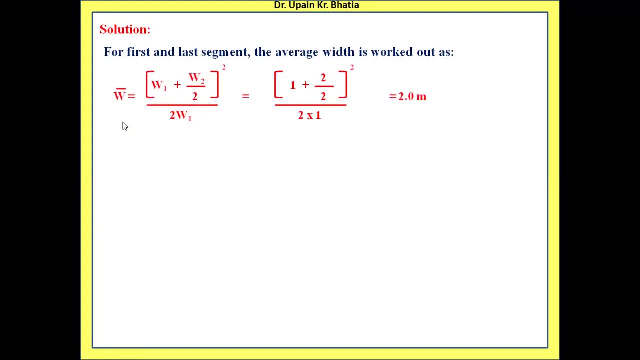 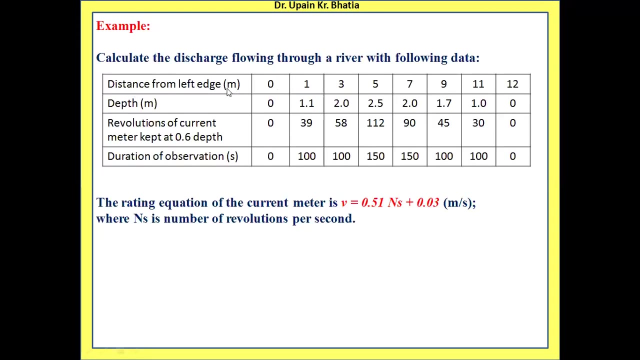 the average width is worked out as this is the formula. so w1 is basically the distance between the left bank to the first vertical. that is one meter, if you just recall this. the distance from the left edge is zero and the next vertical is at one meter distance. so this is. 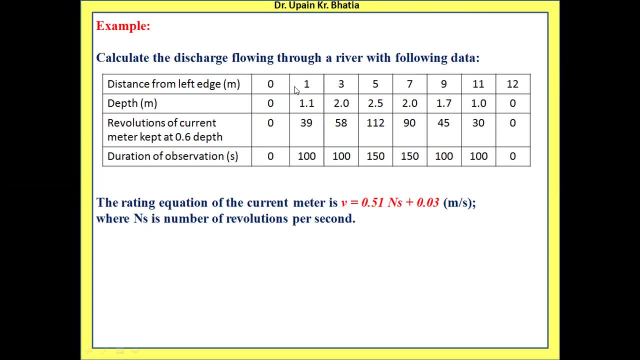 w1, so zero to one, is one meter. so w1 is one meter and w2 is from one to three, that is two meters. w3 is two meters. w4 is two meters, likewise, here it is: wn is one meter, again, ok, and this minus one is two meters. 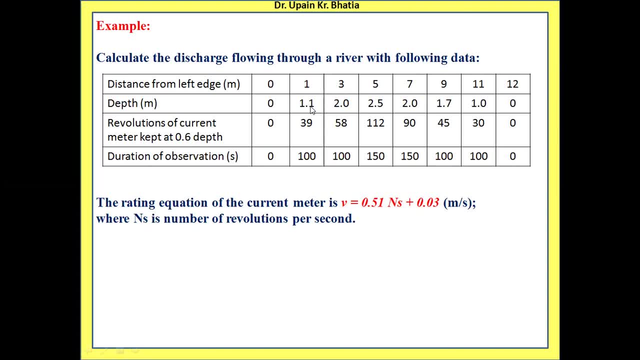 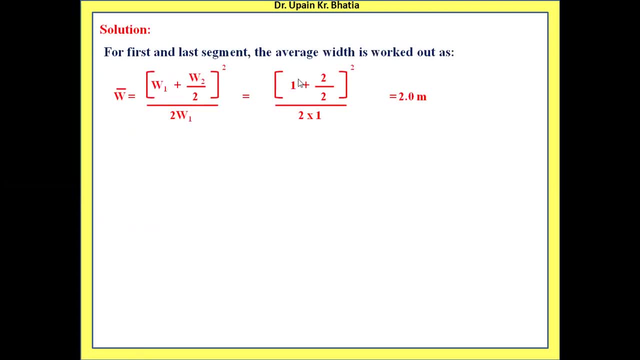 so it is just same as this particular end. so if you see, if you apply this formula, w1 is one, w2 is two. just by applying this formula you get the value of w bar as two meters. that means the w bar value for left side, or the first segment and the last segment. 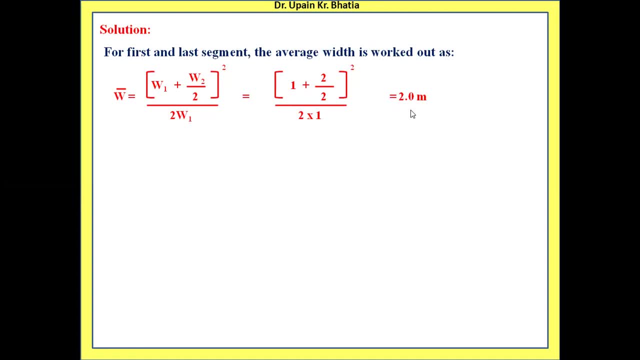 is two meters. ok, for both side, the w bar is two meters. and what about the intermediate segments? the remaining segments are worked out as this expression, which was given in green color in the previous slides. so w bar is wi by two plus wi plus one by two. 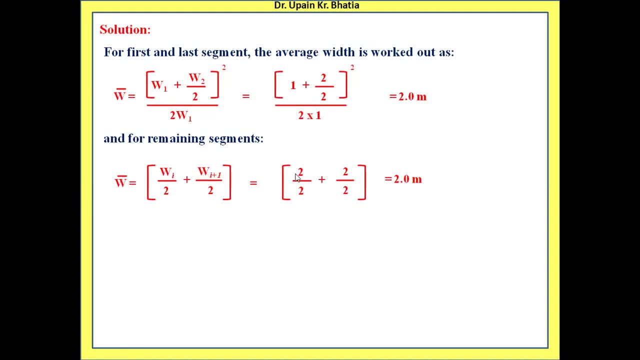 because intermediate, every w value is two meters. so two divided by two plus two, divided by two again, it becomes one plus one as two meters. so all the w bar values are coming out to be two meters. and since velocity is measured at zero point six depth, the measured velocity 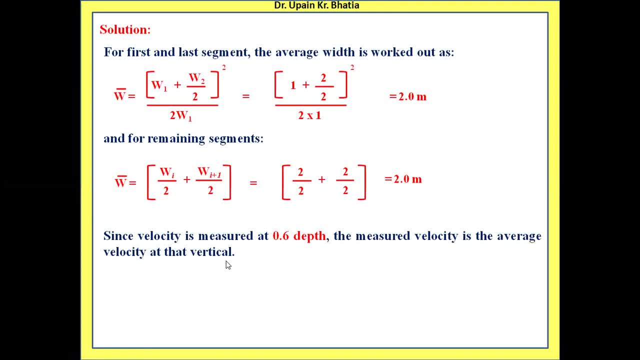 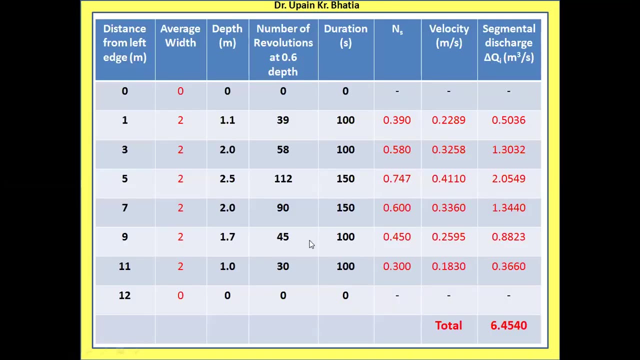 is the average velocity at that vertical. so that we have already discussed. the calculation of discharge is presented in the tabular form. now you can do this individually or in tabular form. so tabular form is better organized way of calculation. it is better understood and easy without. 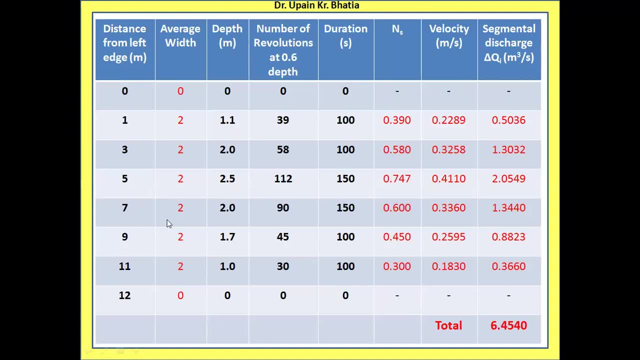 any confusion. you can do it. so the black entries are basically the data which is given to you and the red entries are basically what you have entered or you have calculated. okay, so, like the average width w bar values you have mentioned over here as two meters for all. so 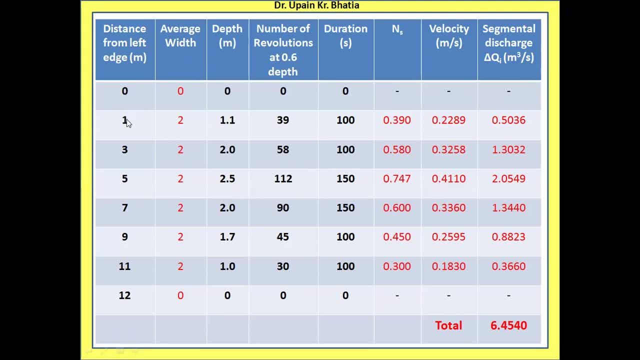 from zero to one. it is not from zero to one. it is taken as two. zero to one and then from one to three somewhere in the middle. this was w. two is two meters over here and somewhere in the middle up to this w bar is calculated to be two meters. 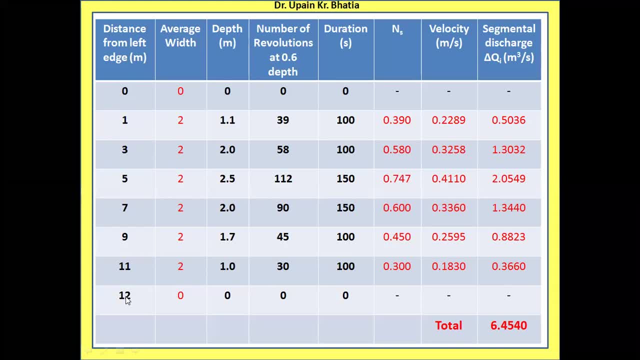 similarly here. this is one meter. from this twelve to eleven and then up to somewhere in between nine to eleven, somewhere here, up to this point only. we have calculated this average w bar as two meters. okay, so all intermediate values are two meters, so non zero values. that is the. 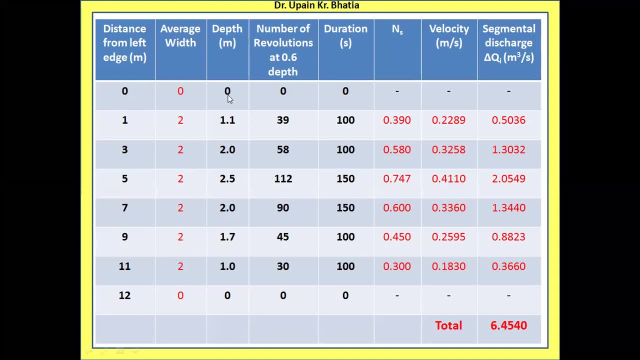 w bar values. okay, at zero, and on both sides you are not getting any average width. so it is. it is taken as zero only, and for every depth you have the number of revolutions and the duration. so thirty nine is the revolutions in hundred seconds. so if you divide, 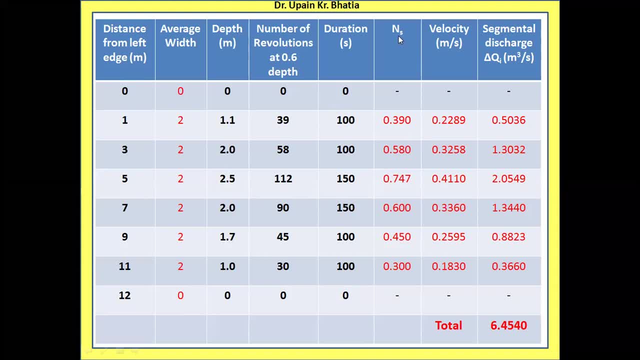 thirty nine by hundred, you get point three nine as ns value. and if you put this ns value in the rating equation, you get this as the velocity in meter per second. and if this is the velocity, then velocity multiplied by area, that means width multiplied by depth. so 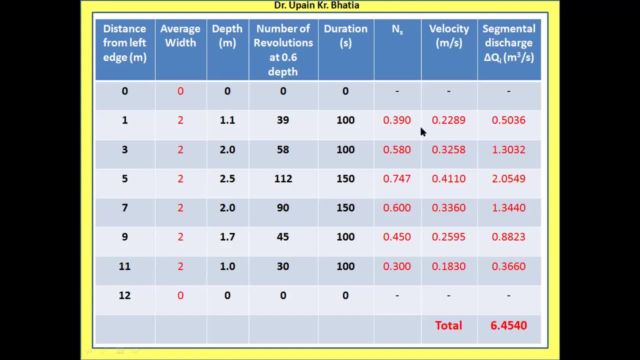 two multiplied by one point. one multiplied by this velocity gives you the discharge delta q in this segment. similarly, two multiplied by this, two multiplied by point three, two, five, eight, it gives you one point three, zero, three, two. it is the discharge in the second segment. similarly, at any segment, if 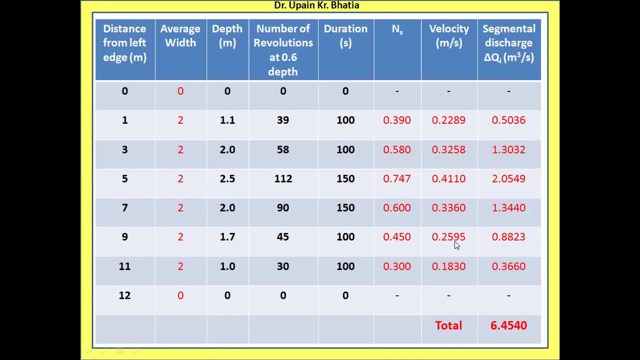 you see two multiplied by one, point seven multiplied by point two, five, nine five, that is point eight, eight, two, three. it is the discharge in that segment. so individual discharge values in each segment. they are calculated. you add them together to get this total discharge in the stream. 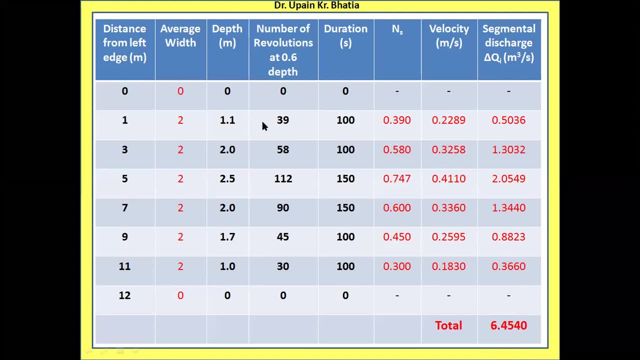 so it is always better to organize your calculation in tabular form. it is easy for you also, it is easy for the examiner also to understand, and there is no confusion, there are no chances of mistake, because if you calculate them separately in the form of, say, text, 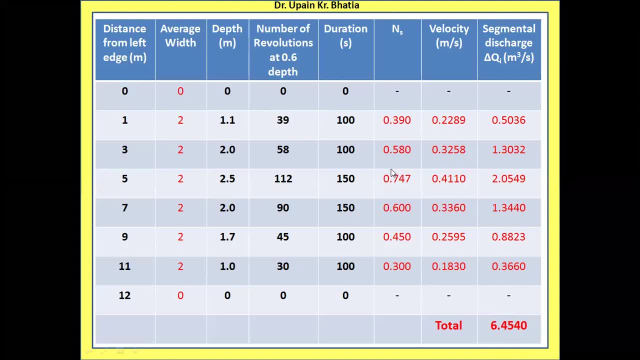 for each segment, then first segment, then for third segment, second, third, fourth, and then you have to collect all these values and then add, so likewise your number of pages will also be consumed more and it will not be easily understood. and if there is some say, some segment is skipped. 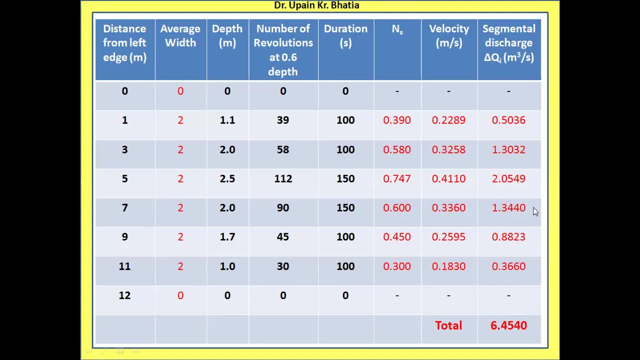 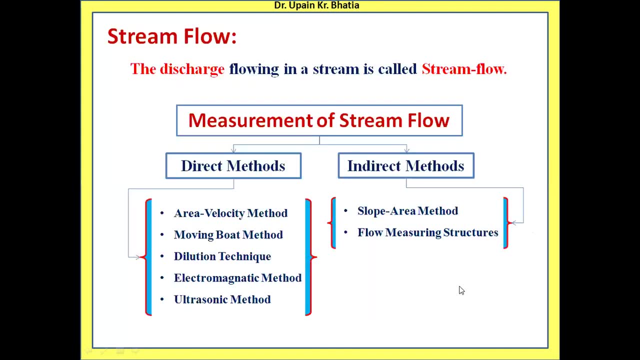 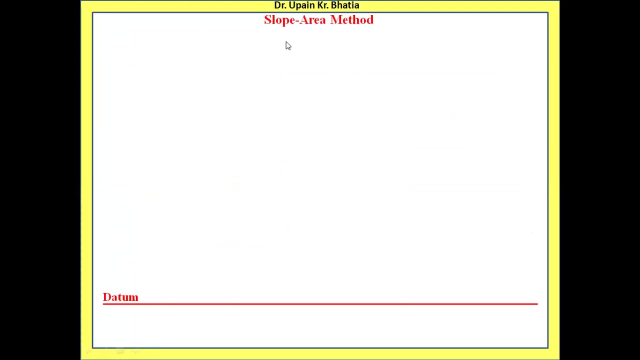 or missed, then you then also you will not be able to point it out. okay, so this is area velocity method. now, coming back to the same slide, we are done with these direct methods, now indirect method. so last method is our slope area method. so slope area method is involving 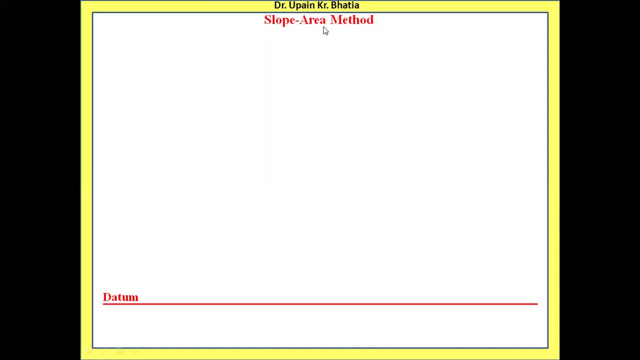 the use of slope as well as the area. okay, so in the previous method we had area velocity in area velocity approach, so in that we just assumed a particular cross section. but here, because we are talking of the slope, so again we have to look for some length. 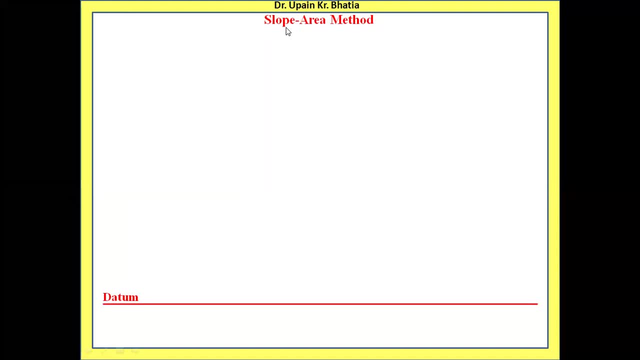 of the stream, so some length L is to be taken for the stream, so two sections are to be involved. okay, so let us say that this is a datum. some assumed datum is there and this is the river bed. river bed is sloping in this direction, sloping downward. 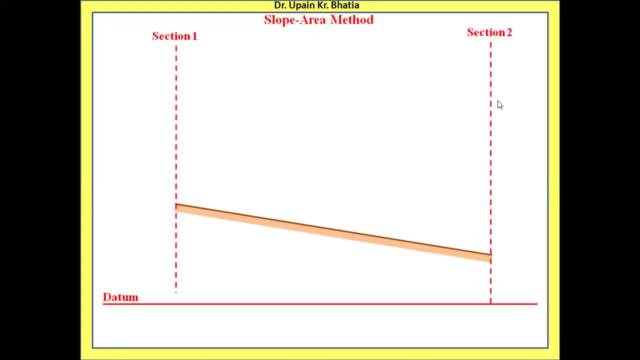 so that between two sections, section 1 and section 2, which are at a distance L apart, the elevation of river bed at section 1 is Z1 and elevation at section 2 is Z2, so Z1 is more than Z2. that is why it is. 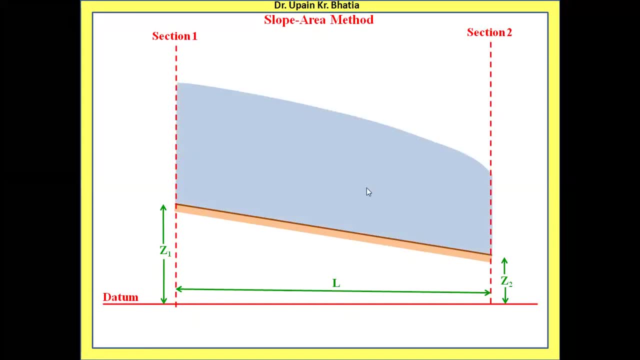 sloping downward. okay, if this is the water flowing in this river. if this is the water flowing in this river, so deliberately I have made this surface as curved one so that it can indicate the change in the water depth also. so water depth at section 1 and section 2 are 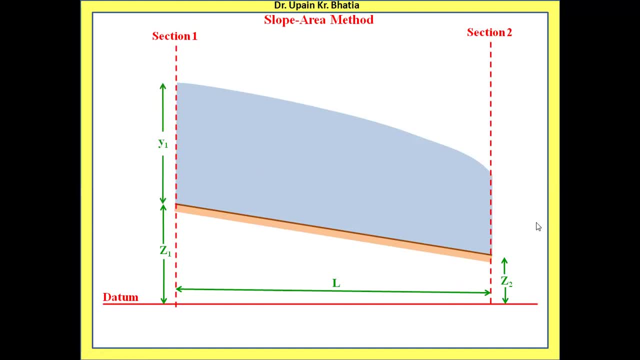 different. so water depth at section 1 is say Y1 and at section 2 it is say Y2 and these two depths are different. now if you draw this as the total energy line, if you recall, total energy line is basically sum of the datum head, the pressure head and 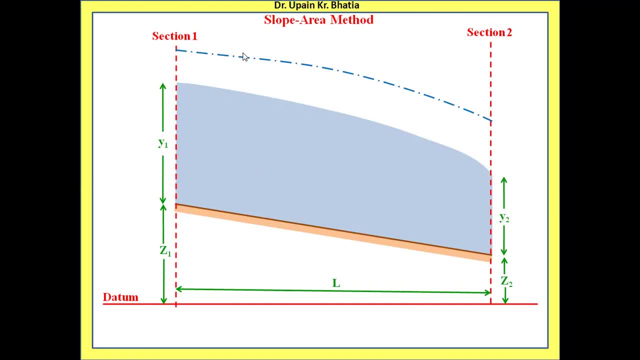 the velocity head. so this total energy line is drawn above this water surface level in the open channel by an amount which is called the velocity head. so at section 1 let us say the velocity head is V1 square by 2g. so V2 by 2g is the way we. 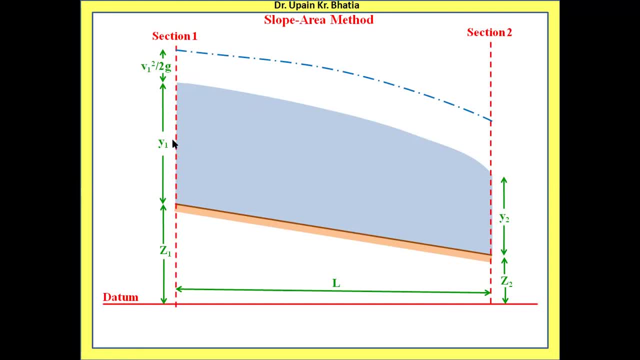 calculate the velocity head. so let us say V1 is the velocity of flow at section 1. so V1 square by 2g is the velocity head at section 1. similarly, V2 square by 2g is the velocity head at section 2. 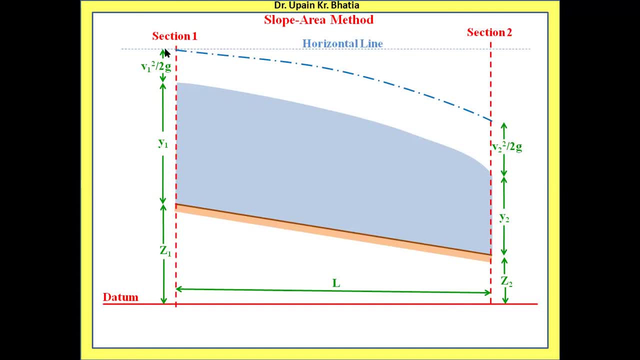 now, if you draw a horizontal line at section at this point, at section 1, and draw a horizontal line over here, what you see over here is: at section 1, the total head is Z1 plus Y1 plus V1, square by 2g. but here at section 2, 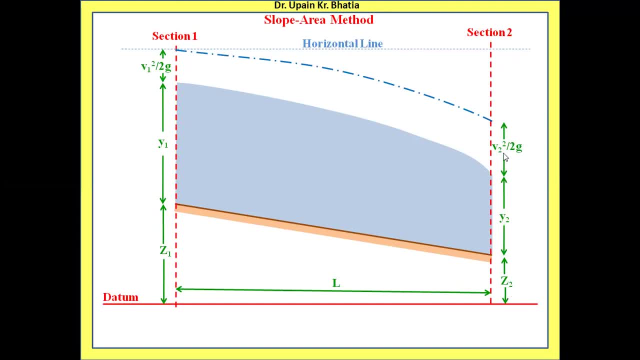 the total head is Z2 Y2 plus V2 square by 2g. it is less than what is available at section 1. so where is the head has gone? so some head is lost. that is head loss. so the total head at both the sections should be the same. 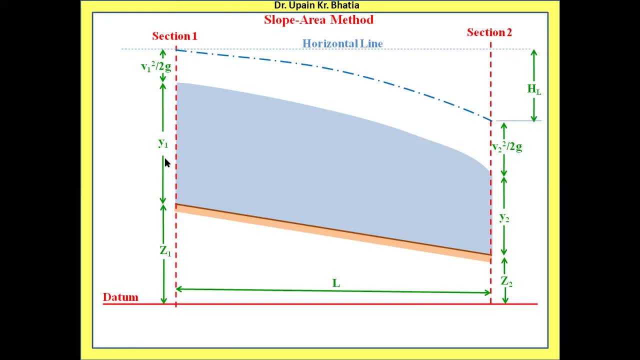 so total head is available as Z1 plus Y1 plus V1 square by 2g at section 1 and Z2 plus Y2 plus V2 square by 2g at section 2, with some head loss, HL, and this head loss is caused. 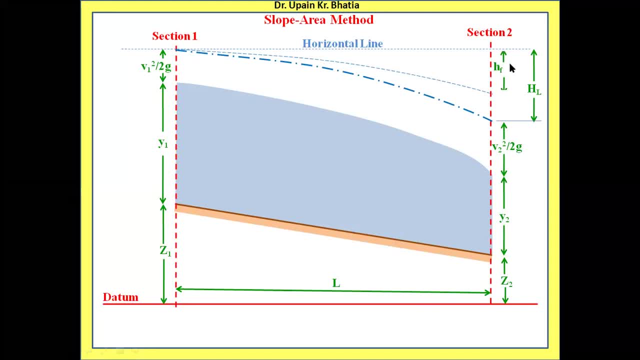 by two factors: one is due to the friction, which is called HF, and another is HE, that is caused by the eddies. so HL is basically divided into two per component, that is, HF and HE. so now you see that this horizontal line and this datum line, both are parallel. 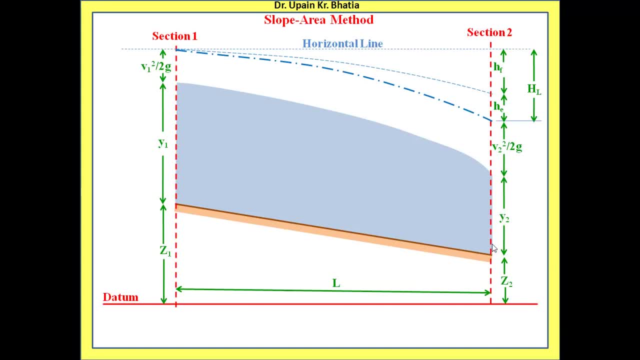 so the total head on this section 1 and at section 2. if you see they should be equal, now let us equate them. if you have understood how this is formed, so you can write this thing as an equation, which is called the energy equation, you can see the Bernoulli's equation also. 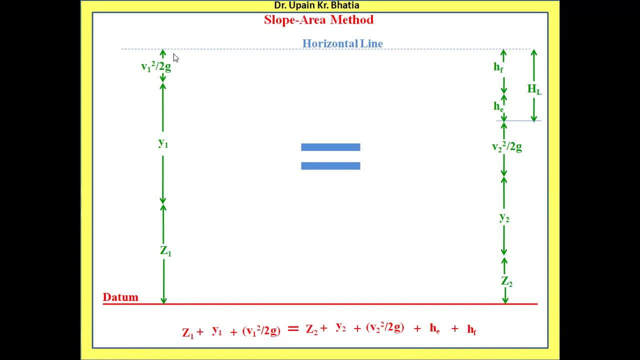 so simply Z1 plus Y1 plus V2 square by 2g, it is Z1 plus Y1 plus V1 square by 2g. that is equal to Z2, Y2, V2 square by 2g, HE and HF. so all these terms are: 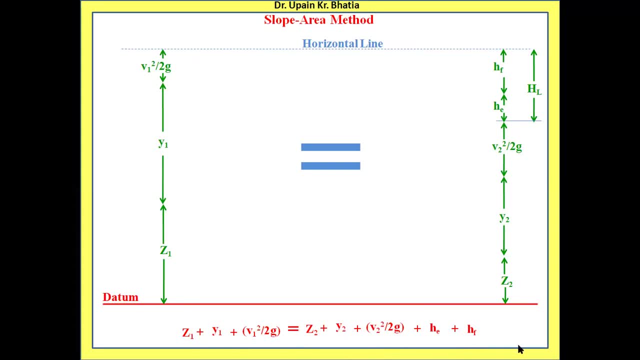 written over here. so this forms the equation. so how this equation has come that we have just seen. so let us rewrite this equation over here on the top: and Z1 plus Y1 is taken as H1 and Z2 plus Y2 is taken as H2. 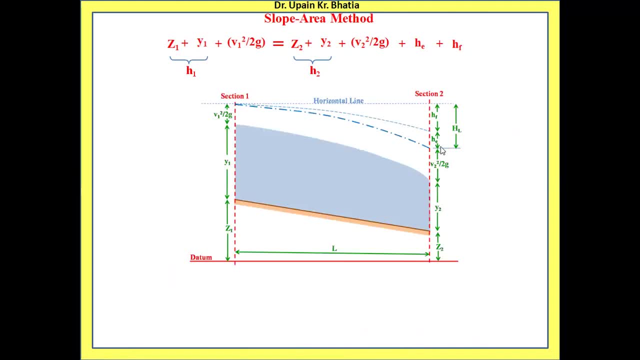 and do not get confused, these H1 and H2 values are, if you see, in this particular diagram, Z1 plus Y1 means Z1 plus Y1. it is this combined value H1, because it is measured from the datum. so this height H1 is basically. 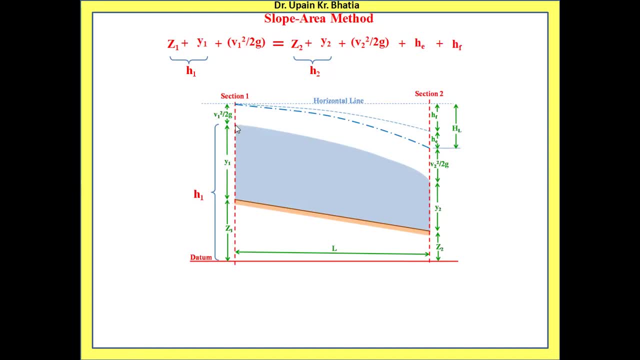 the water surface elevation at section 1 above this datum, of course. so water surface elevation at section 1 is H1. similarly, water surface elevation at section 2 is H2. so if you just measure, if you just observe the water surface elevations at section 1 and 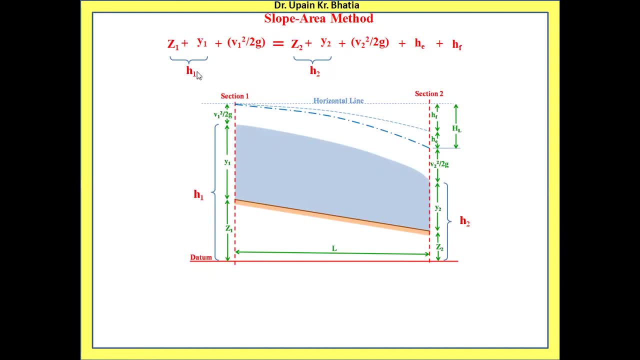 section 2. so you have worked out basically H1 and H2. that means Z1 plus Y1 is collectively observed as H1 plus Y2 is collectively observed as H2. now you rewrite this equation as this: instead of Z1 plus Y1, H1 and instead 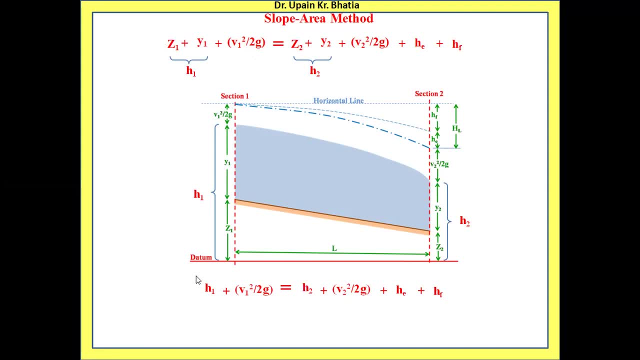 of Z2 plus Y2, you have written H2, yes, rest, everything is remaining the same. now, if you rearrange these terms for HF, so this HF is taken on one side and rest- all other terms- are taken on the other side, then because HF, you keep it over here, then H2 will be. 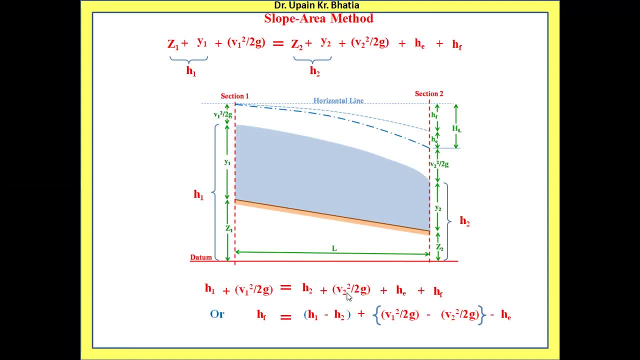 taken over there so it becomes H1 minus H2. so this velocity head at section 2 will be taken on the other side, so it becomes V1 square by 2G minus V2 square by 2G, and HE is also taken to the other side as negative value. 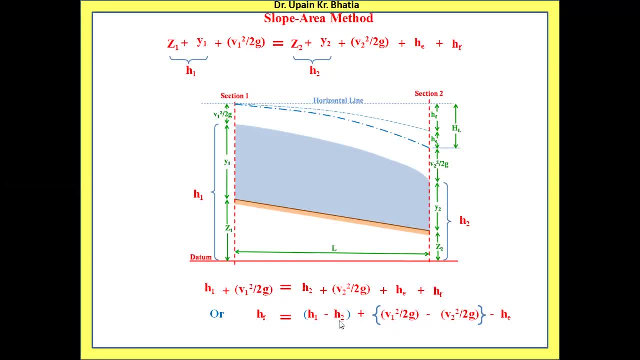 so and you have grouped them together as H1 minus, H2 plus, in these curly brackets as difference in the velocity heads at two sections, minus this eddies, head loss, head loss due to eddies. so this HF is written in this fashion. so let us rewrite here again. 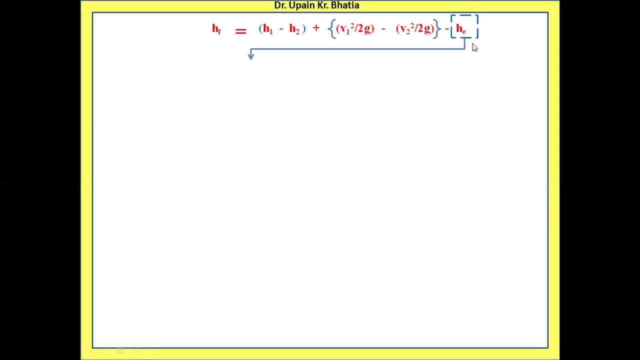 at the top. now this HE, which is called the head loss due to eddies. it is estimated as this expression. HE is also dependent on the difference in velocity heads. but sign is not important, only the magnitude values are taken. these two vertical lines means, even if it is. 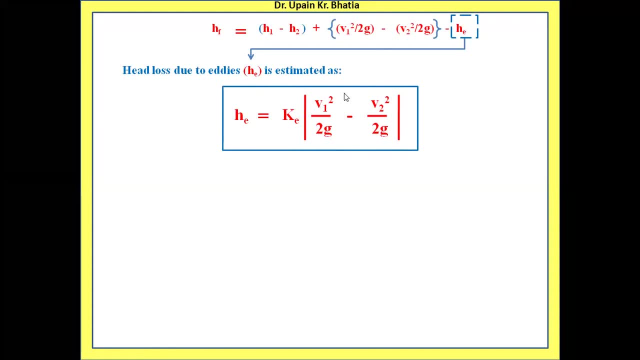 this expression inside it is coming out to be negative. you have to take the absolute value, so the positive value is to be taken. okay, so V1 square by 2G, if velocity head is more at section 1 and it is less at section 2. 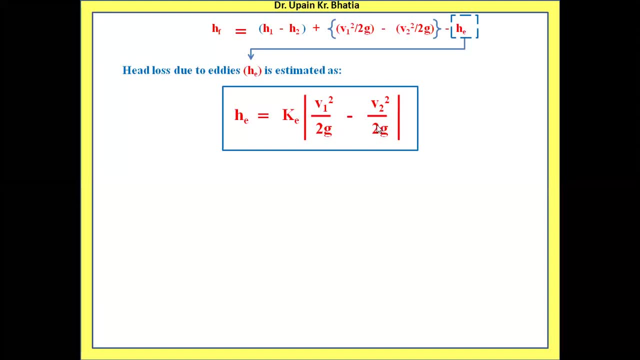 obviously this will be positive value. but if velocity head at section 1 is less than section 2, then this value will be negative. but you have to take the absolute value as the positive value only, and then this difference in velocity heads is to be multiplied by a constant. 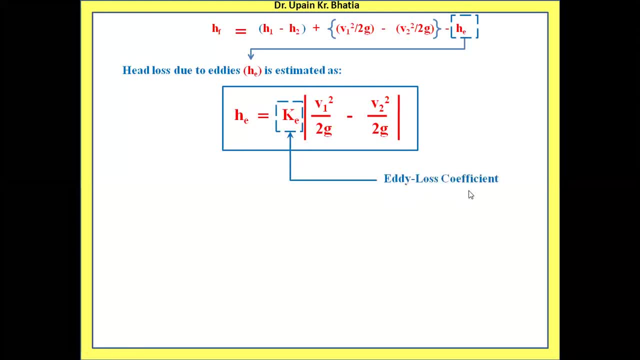 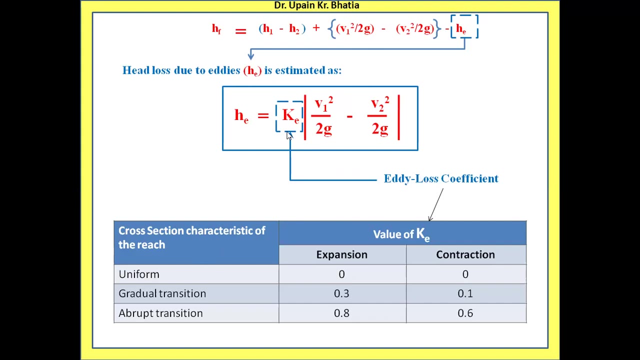 KE, which is the eddies loss coefficient. so this KE is eddies loss coefficient and its value is taken from this table. so KE value because it is because of eddies. so eddies are generally generated because of change in the cross section. if the cross section 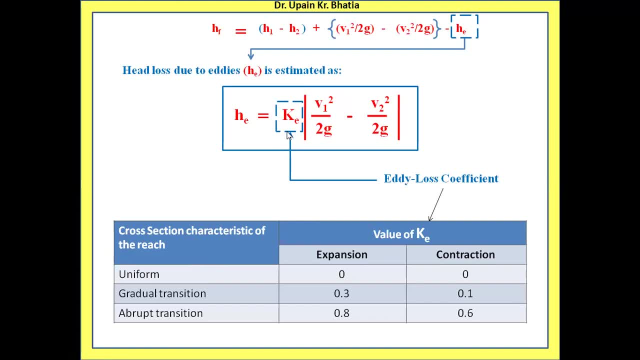 is either reduced or if it is enlarged, then the eddies are generally generated. so it depends upon the cross section characteristics of the reach. if the cross section characteristic is, say, the reach is uniform, that means from section 1 to section 2 there is no change in the cross section. 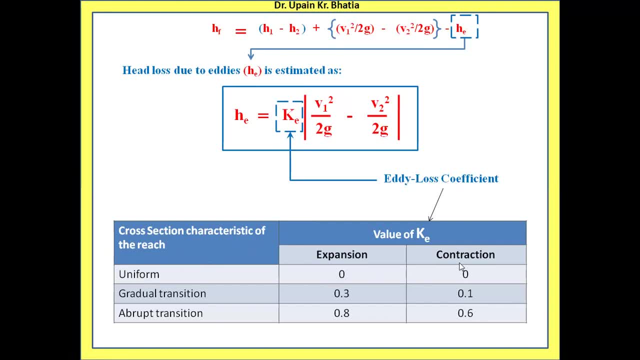 characteristics. then there is no expansion, there is no contraction, so value of KE will be 0. or you can say: for the prismatic channels this KE value will be 0 because same cross section is running from section 1 to section 2, so no eddies will be generated. 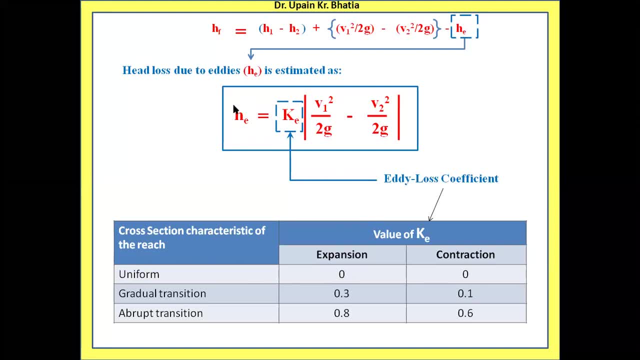 so no head will be lost because of the eddies. so head loss due to eddies will be 0. so HE value will become 0. but if the channel cross section is transiting, if it is changing from section 1 to section 2, 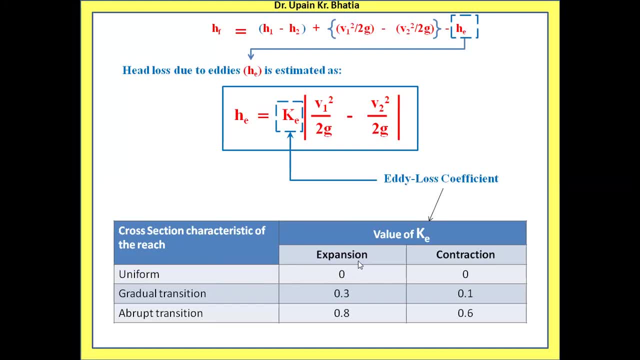 if it is increasing, that means expanding. and if that expansion is gradual- so gradually it is expanding from section 1 to section 2- then KE value is 0.3, and if it is gradually contracting from section 1 to section 2 it is 0.1. 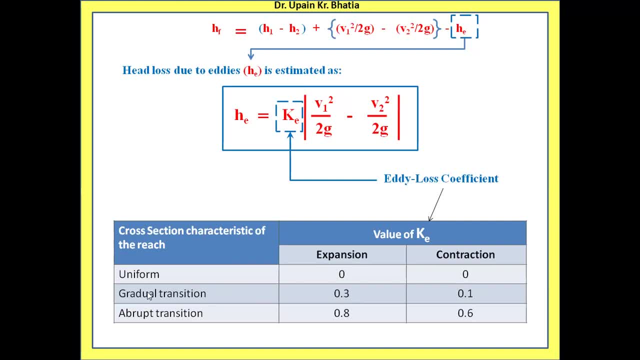 but if this expansion or the contraction is not gradual, but it is abrupt, all of a sudden it is expanding and all of a sudden it is contracting, in that case for this abrupt expansion the value of KE is 0.8. see increased value is there because more eddies will be formed in this. 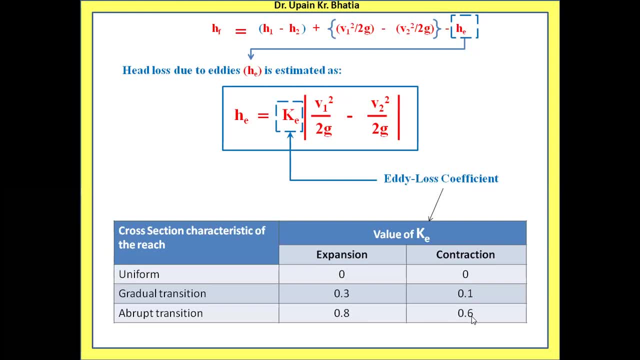 but in case of contraction it is 0.6, here it is 0.8, here it is 0.6. so more eddies are formed when the channel is expanded and less eddies are formed when the channel is contracted and gradual transition. 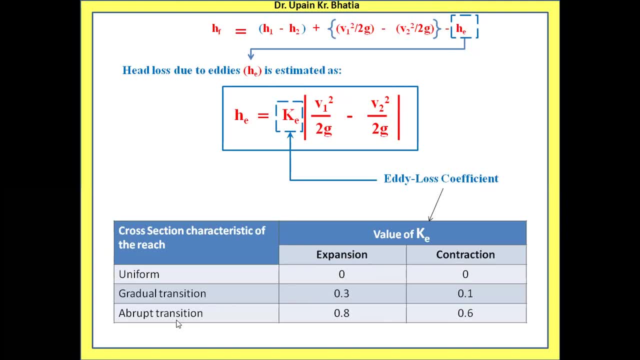 observes less eddies and abrupt transitions observe more eddies. so in the same pattern, the values of this KE. they are also written in this table and you can select an appropriate value of KE depending upon your condition, that situation, or you can say the characteristics of the reach. 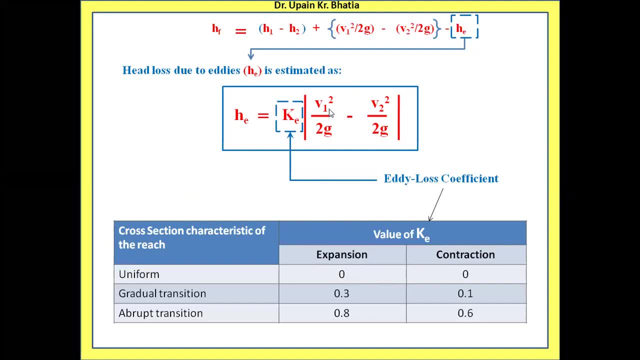 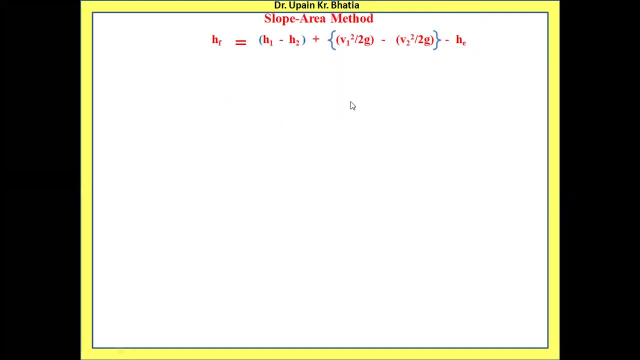 so KE value is suitably adopted from this table. so you can say the velocity head, section 1 and section 2. they are calculated separately now in the same equation. the energy slope, if you see that is SF. it is designated as SF. it is equal to HF by L. 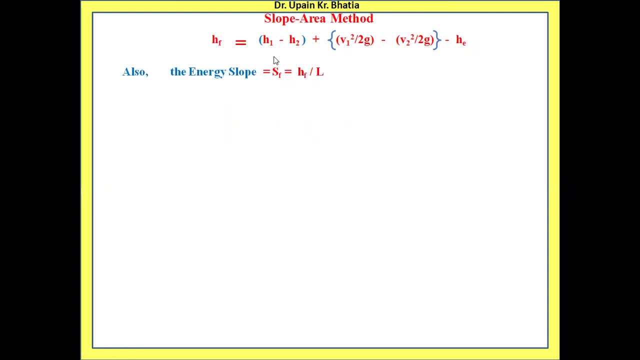 so this is generally what is adopted as the energy slope. it is the friction loss divided by the length, so in this HE is not considered. so energy slope is generally taken as the head loss due to friction divided by the length, and it is generally same as the bed slope. 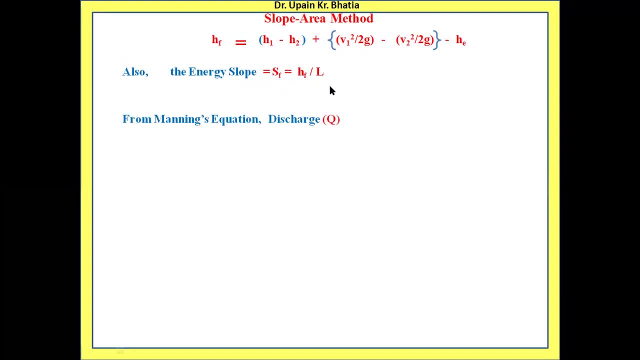 also so SF is equal to HF by L and from Manning's equation- if you recall from the fluid mechanics, the Manning's equation for calculating the discharge in the channel or the velocity that is given by this equation- so discharge is equal to area multiplied by this velocity. so this portion is: 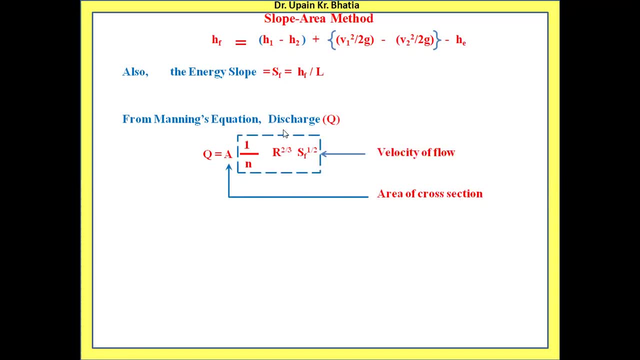 velocity. so this is the area of cross section and remaining portion is the velocity of flow, and velocity of flow is 1 by N. here N is Manning's coefficient, R is hydraulic mean radius and SF is the bed slope we have already discussed over here here this R is hydraulic mean. 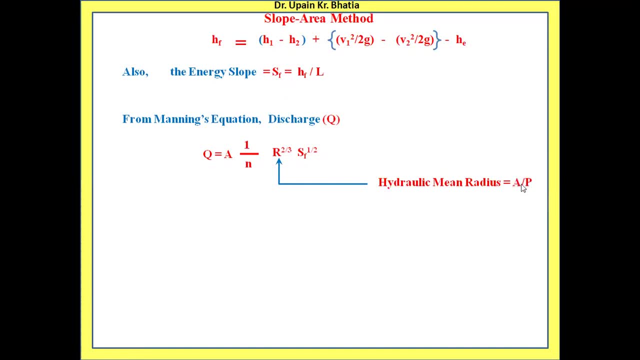 radius. it is calculated as the area of cross section divided by wetted perimeter of the channel cross section. so wetted perimeter is how much water has wet the perimeter of that cross section, how much of that portion is wet because of the water. so from overall cross section area, 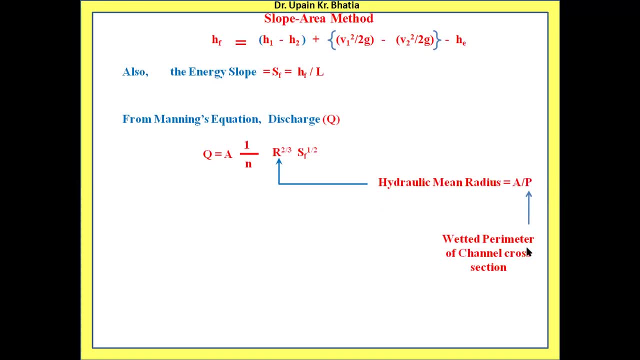 from its perimeter. you have to consider wetted perimeter. so area of cross section divided by wetted perimeter gives you the hydraulic mean radius. now, SF is the bed slope, which is equal to energy slope. HF by L we have already discussed. now, after this, if you club these, 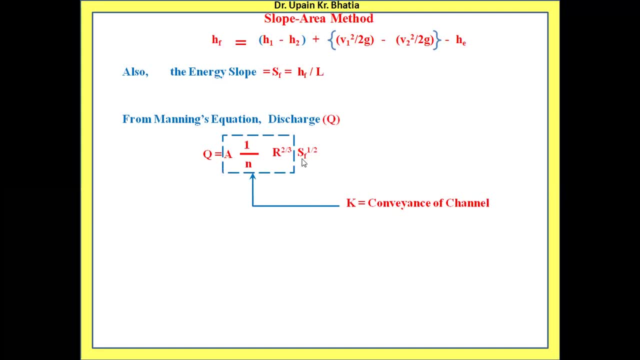 parameters together. these parameters, other than this SF, all these parameters collectively, are known as conveyance of the channel. it is represented by K. mind it. it is not KE, it is K. KE is the eddies loss coefficient that we are not going to use it here. 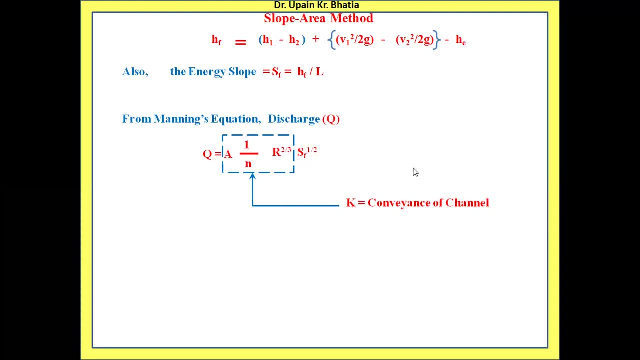 it is K, which is called conveyance of the channel and all the parameters in this blue dotted rectangle. they are related to the cross section. that means the parameters of a particular cross section, but here SF is the characteristic of the length of the reach. ok, so this is K, it is. 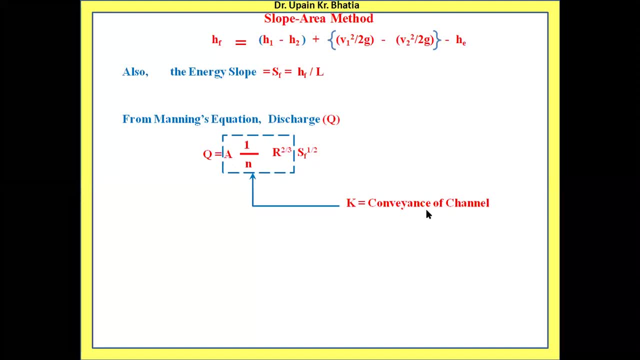 cross section characteristics and it is basically called the conveyance of the channel at that cross section. so if you rewrite over this equation, it is simplified simply written as Q is equal to K times square root of SF, or SF raised to power 1 by 2. 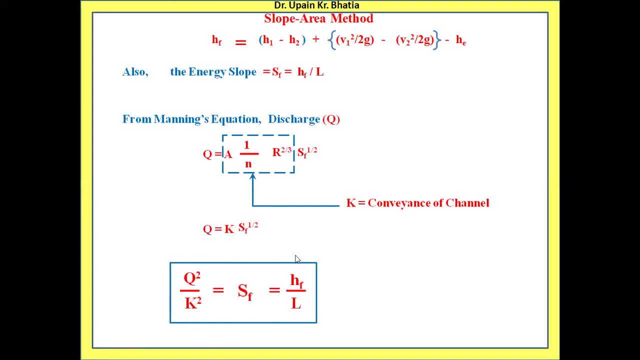 and this expression. you combine this and this. you can formulate in this fashion: like: Q square upon K square is equal to SF. if you just square it and rearrange it, it forms Q square by K square as SF, and this SF is also equal to HF by L. 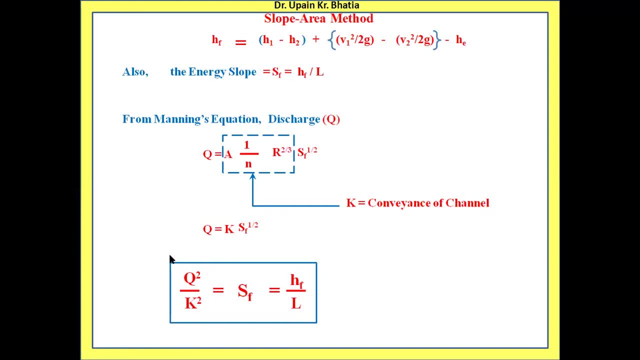 so this forms the basic equation which will be used for calculating the discharge. how it will be used, we will see it later on, but this is an important equation, so we keep it in our mind. so next is the channel cross section. if you see, in this particular 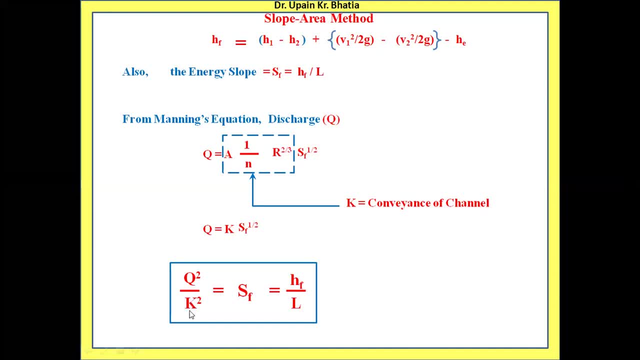 way, this value is K and I told you this dotted blue rectangle is related to a particular cross section only. so one cross section, either section 1 or section 2 we are talking of. so this K is K belongs to section 1 only, or section 2. 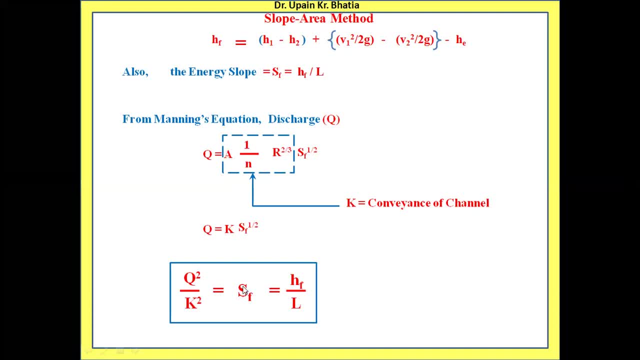 only, but here we are equating using a length and a particular, you can say the discharge. this HF and overall length of reach is also taken, slope is taken. so what value of K is taken? is it to be taken for section 1 or section 2? 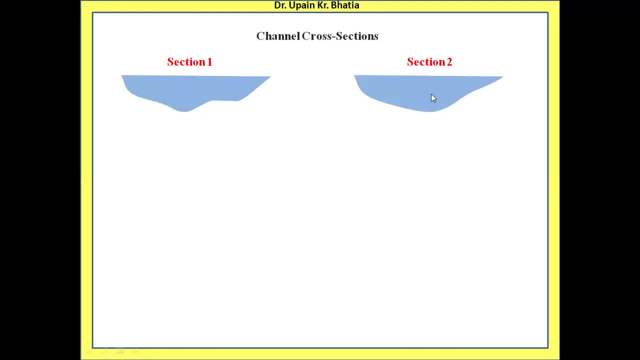 so let us see if this is section 1 and section 2 cross section is given. area at section 1 is A1 and area at section 2 is A2. this red line is the wetted perimeter. similarly, here, this portion which is wetted. 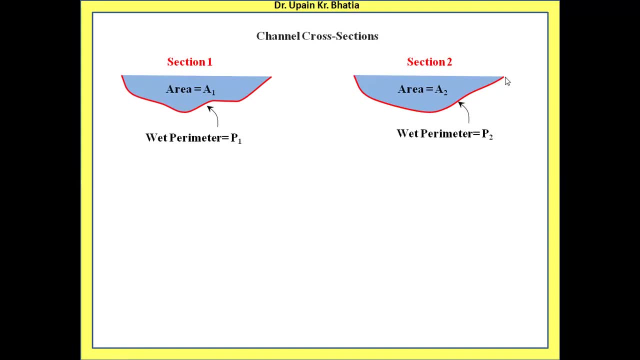 is here because the ground or the earth is going in this fashion also beyond this also, but that is not being wet because of this water. this is the water surface, so cross section is being wetted as per according to this water, only with this red line, only, so this is taken. 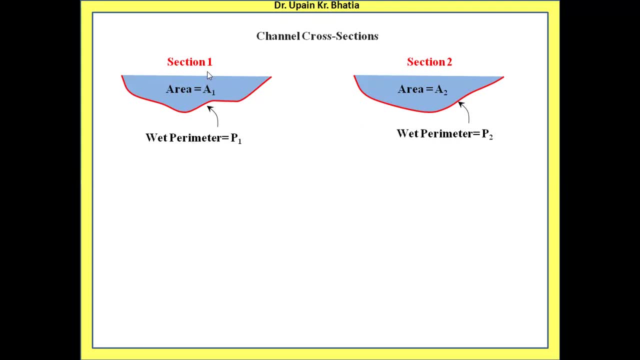 as the wetted perimeter. so wetted perimeter at section 1 is P1 and section 2 it is P2. so if you calculate the mean hydraulic radius R1 at section 1 it is equal to area A1 divided by this wetted perimeter, P1. 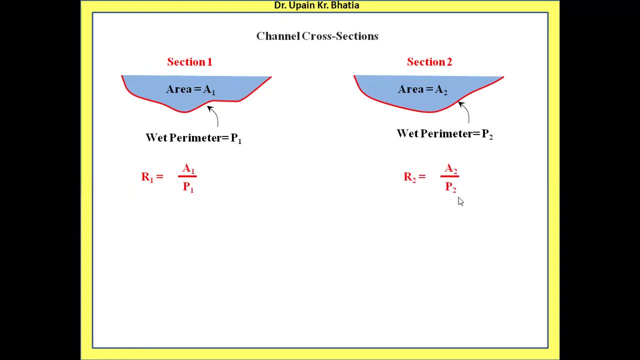 similarly at section 2, R2 is equal to A2 by P2. further, if you calculate the conveyance at section 1, it is A1, 1 upon N1. R1. raise to power 2 by 3, because R1 you have just calculated. 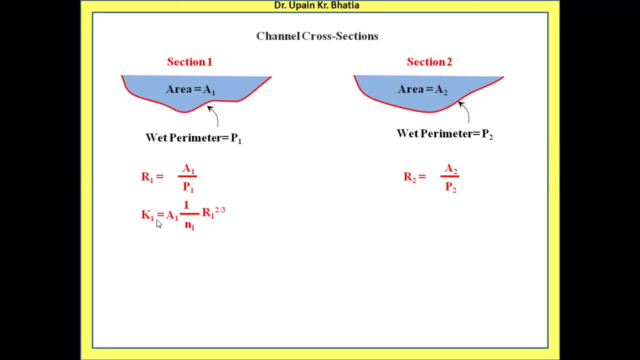 it can be used for calculating the conveyance of section 1. similarly, the conveyance of section 2 will also be calculated. now, the conveyance value at section 1 and section 2. both are calculated, so they will be combined together to get the average conveyance of the channel. 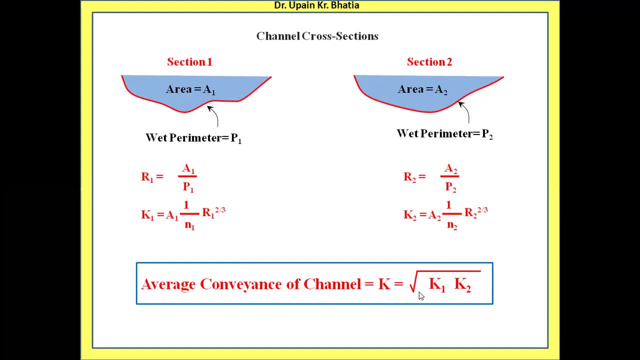 as K1 multiplied by K2 square root. so we are talking, we are calling it as average conveyance of the channel. and don't get confused: that average conveyance should be taken as K1 plus K2 divided by 2. that is basically the arithmetic mean or arithmetic. 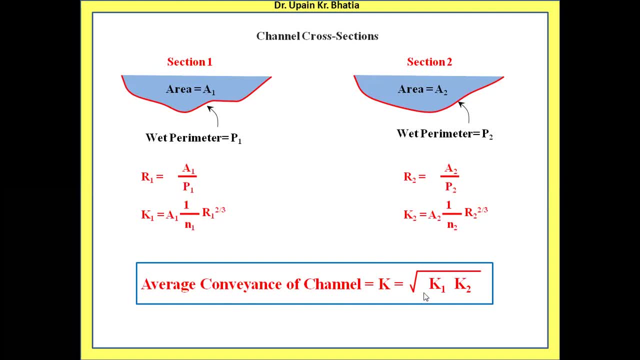 average here. this average conveyance channel is the geometric mean, not the arithmetic mean. so geometric mean is calculated by multiplying the two things together and taking the square root of the product. so K1 multiplied by K2, take the square root. that will give you the average value of conveyance, which 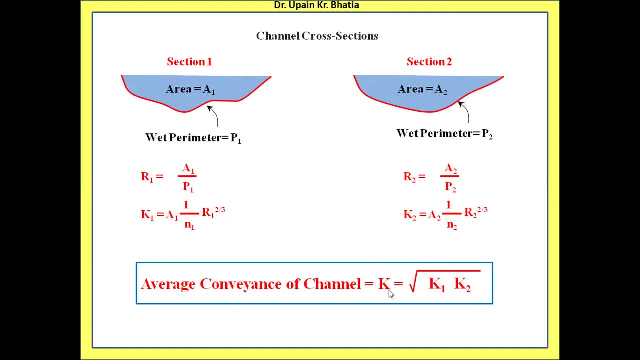 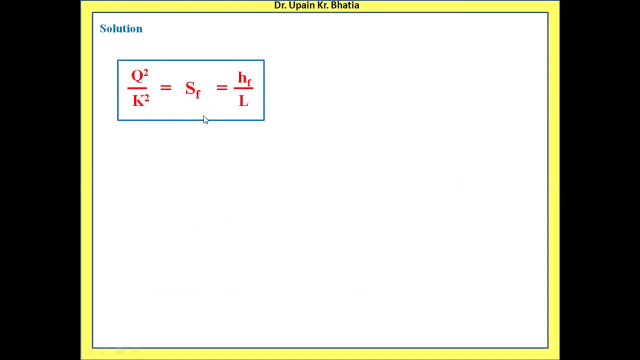 is to be used in that equation that we saw in the previous slide. in this equation I was talking, so this is the equation that we are going to use for calculating the discharge. now let us see how to proceed. this HF value is taken from this equation that also we have. 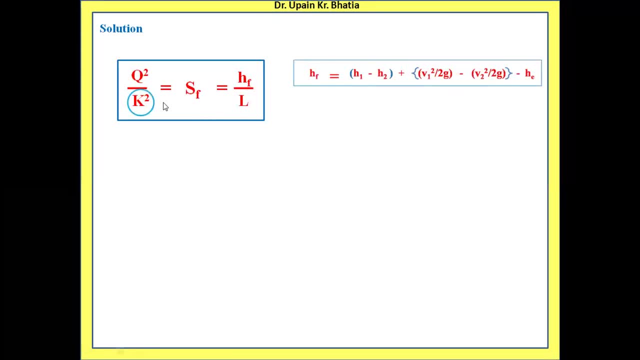 discussed. ok, this K value is to be taken as per this procedure that we have just seen in the previous slide. only this HE value is to be calculated in this fashion, depending upon the characteristics of the reach, whether it is expanding or contracting, gradually or abruptly. so suitable value of 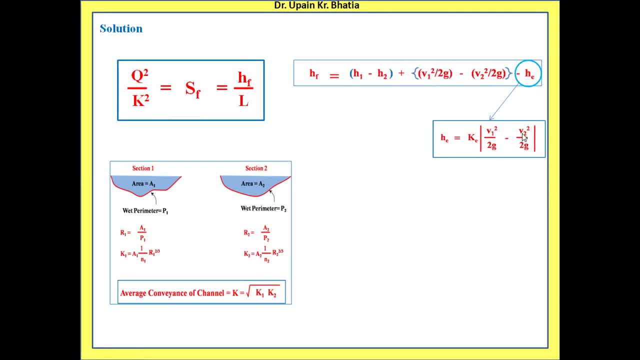 KE is to be adopted. rest other is dependent on the velocity heads. velocity heads are used here also and here also now. once all these parameters are in front of us in the single slide, only the discharge can be calculated in this fashion. if you see, discharge can be calculated. 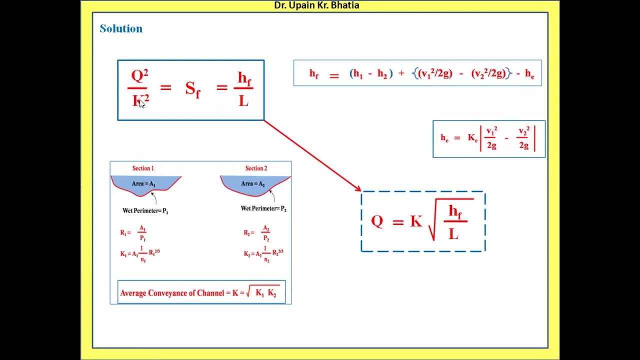 as Q is equal to take the square root, K is taken over here, K into SF, where SF is HF by L. so K multiplied by HF by L, because we are taking the square root of everything. so K multiplied by square root of HF by L. so this is the 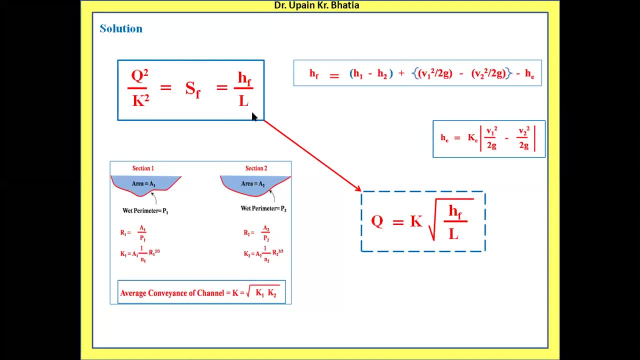 governing equation, which is taken from this equation. now, this is, this forms a concept board, because it is giving you all the expression and all the values over here. so first of all, we need to estimate the value of HF. so HF value is to be calculated. divide by the length of reach, take: 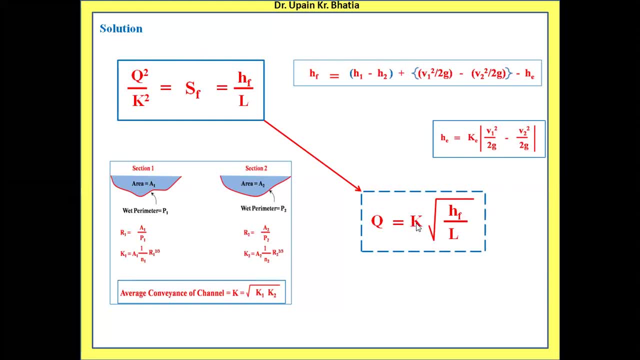 the square root multiplied by the value of K, which is obtained in this fashion. so this is the overall procedure. then get the value of Q. it appears to be a simple procedure, but when you start calculating it, the very first thing HF needs the value of H1. 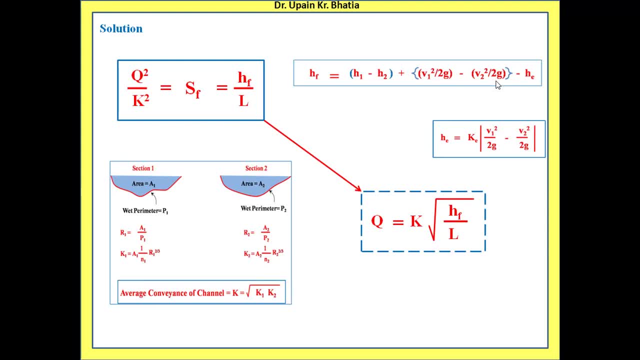 minus H2, then V1 square by 2G, minus V2 square by 2G, and then HE also ok. so everything is to be known so that HF can be calculated. so, in the beginning, because we don't know the values of V1 and V2, if we 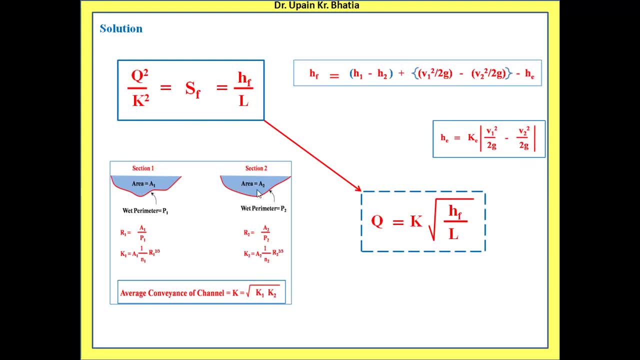 knew the values of V1 and V2, then the area A1 and A2. we know we can directly multiply them and do the discharge work out. ok. that means V1 and V2 values are not known to us, so velocity heads are also not known. 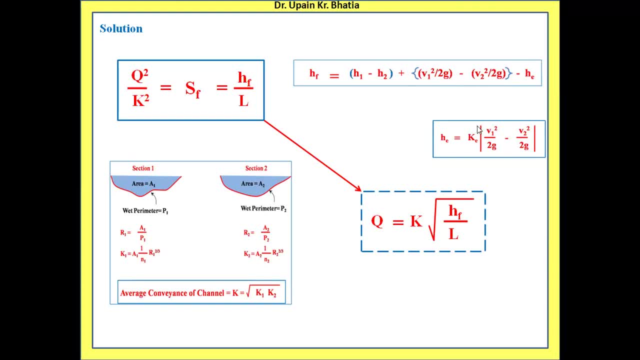 and the you can say this head loss. HE is also not known to us, sorry. so what we do is: initially we assume that V1 is equal to V2, so that this entire parameter becomes 0 and this term becomes 0. similarly, V1 square by: 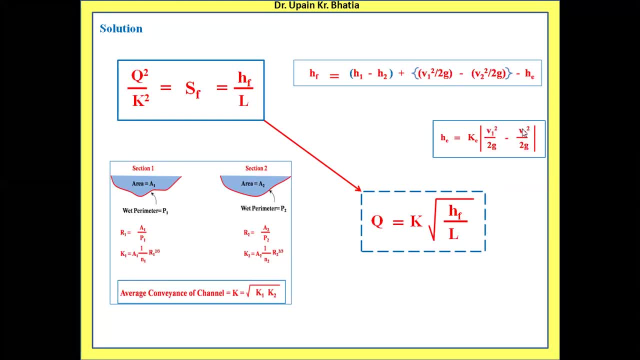 2G and V2 square by 2G. if they are equal, this difference becomes 0. so this entire thing becomes 0. so in this entire equation, HF is initially assumed to be equal to H1 minus H2, which is the difference in the water surface. 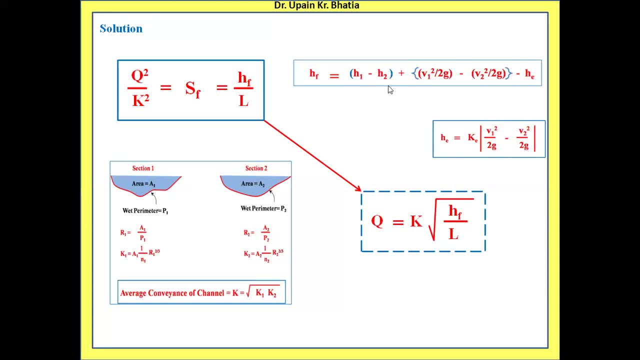 elevations of the stream at two sections. now the water surface elevations we have observed on both sections, we first assume their difference as HF. so at very first we take the value of HF as H1 minus H2. when we put that, the value of Q 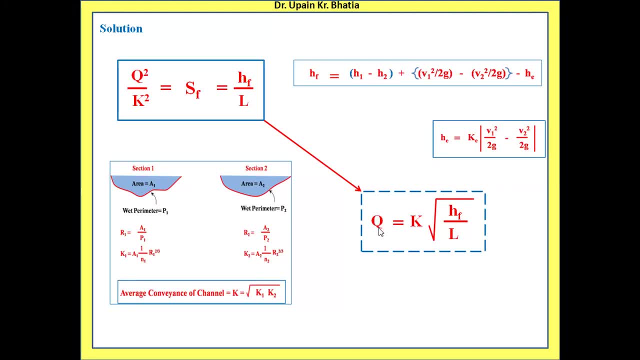 discharge will be calculated. that will be the first trial value of, you can say, discharge. once the discharge is known, then this discharge is divided by cross section, area A1, to get V1 and that discharge because it will pass from section 2 when we divide it from A2. 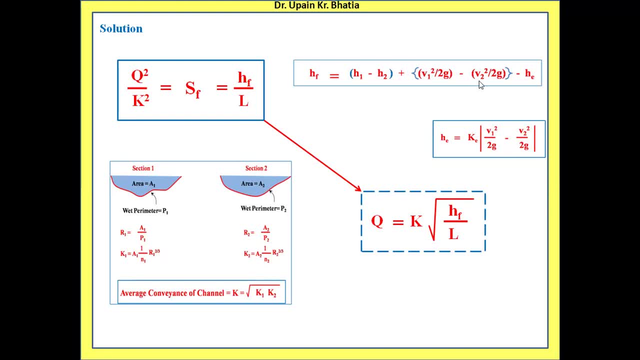 then we will get velocity V2. that means now we have to calculate velocity heads, sufficient information. now. we have calculated the values of these velocity heads so we can calculate the value of HE also. so this entire value of HF will get modified. so if this value of HF 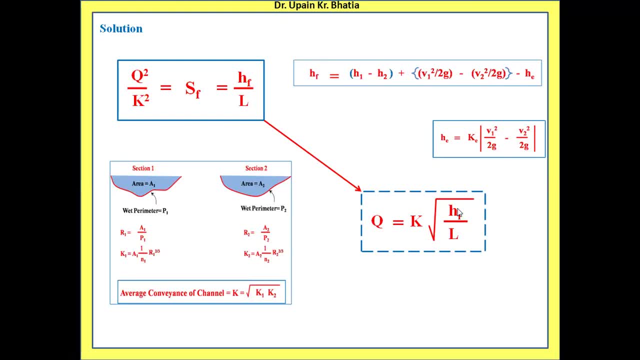 is modified, obviously this modified value will be put over here and ultimately this Q value will be modified. so this modified value of Q will further modify the value of V1 square by 2G and V2 square by 2G. so we have to do this cyclic calculation. 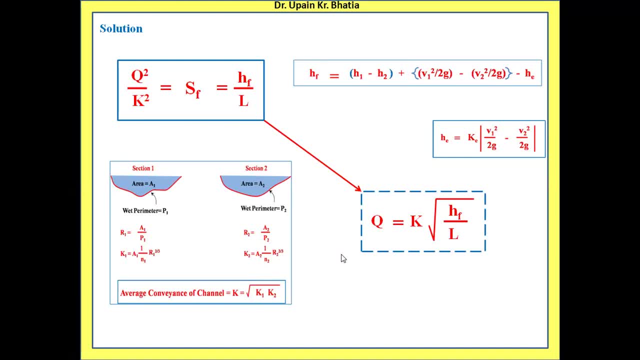 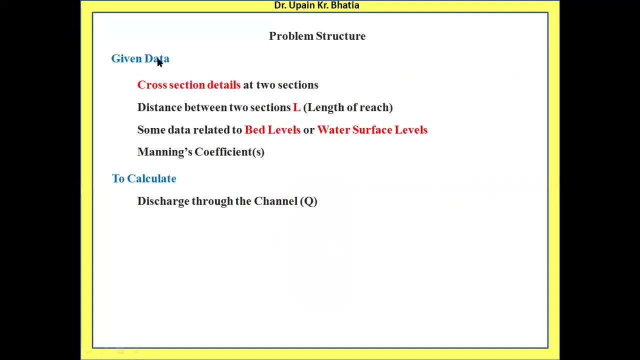 till we get the same value of Q as calculated in the previous step. so this is the procedure. so let us see the problem structure that the given data will be of the form that cross sectional details at two sections will be given to you: the distance between the two sections. 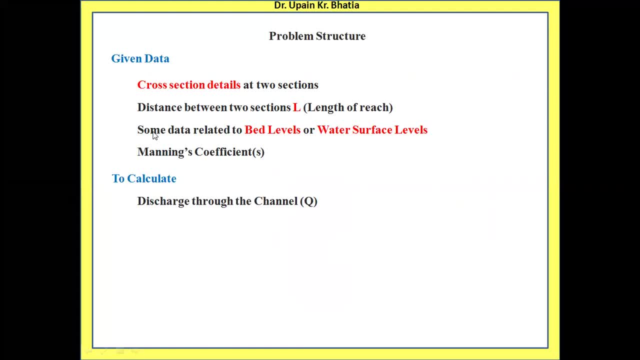 L will also be given to you, it will be known to you, it will be given and some data related to the bed levels or the water surface levels will be given to you so that you can start with the calculation of the value of HF as H1. 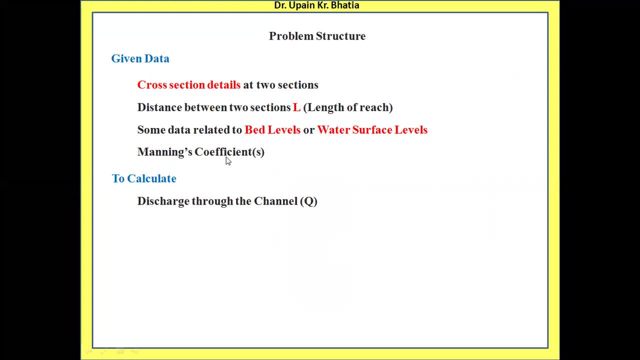 minus H2 Manning's coefficient will also be given to you, because that is going to be that is used in calculation of the conveyance and hence the average conveyance. you will be required to calculate the discharge through the channel. okay, so this much data will be given to you. 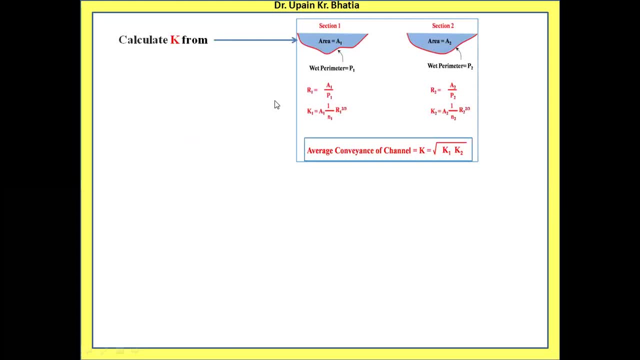 and if you see this particular diagram, you have to calculate the value of conveyance from this. initially assume V1 is equal to V2, that I have just told you. in this equation, HF is reduced to H1 minus H2, H1 minus H2, so HF is equal to. 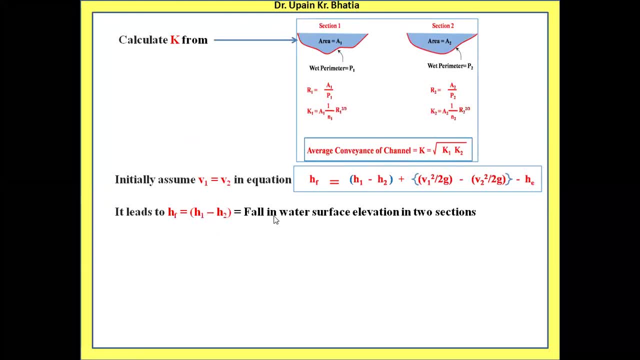 H1 minus H2 is what we have to take initially, which is equal to all in the water surface elevation, in two sections. then calculate the value of Q from this equation, because K you have already calculated, HF you have taken from here, L is already given to you in the 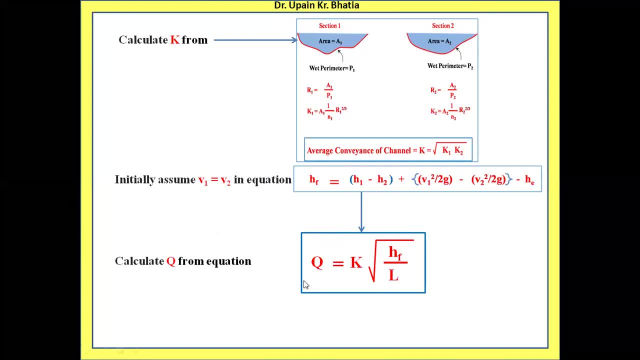 given data so you can calculate the value of Q once Q is known, calculate V1 and V2 as Q upon A1 and Q upon A2 respectively, and use them to calculate HF again now, because earlier you assumed HF to be equal to H1 minus H2 only.